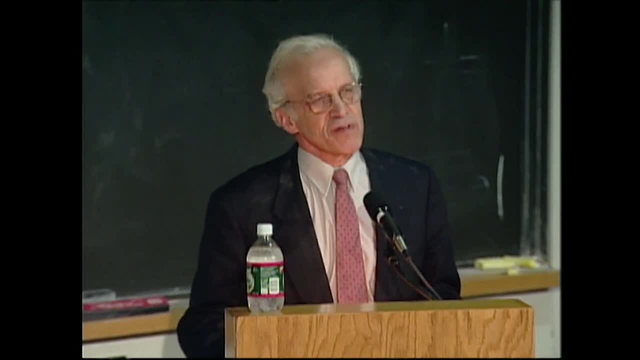 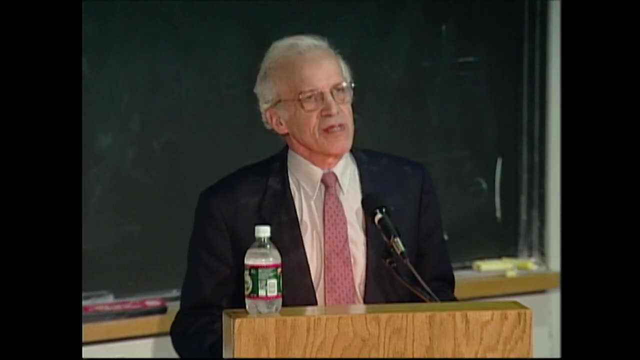 I had the great good fortune to have Dave Pritchard as one of my first graduate students and to have the experience of him as a colleague at MIT for many years. Dave has many accomplishments. This year he has mentored directly two of the Nobel Prize winners, Wolfgang Ketterle. 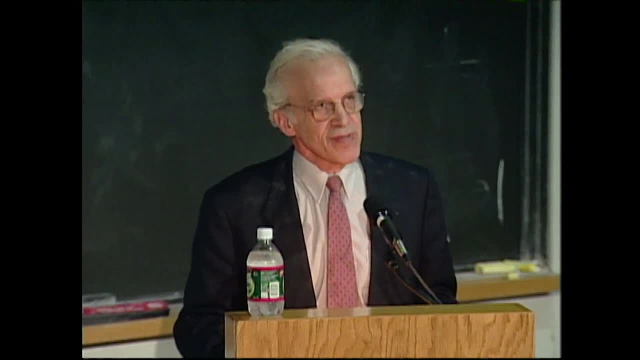 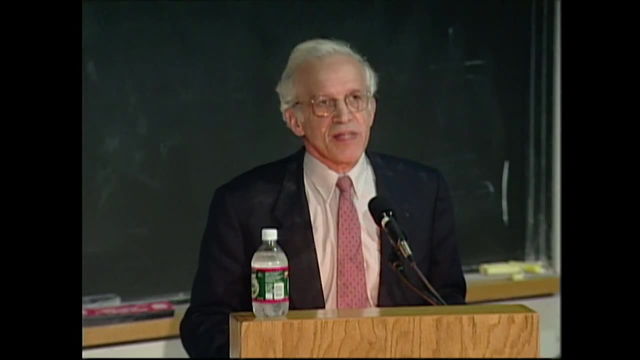 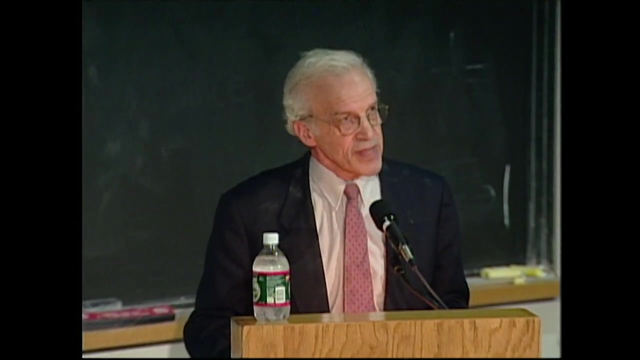 and Eric Cornell, who is a graduate student of his. He has made many seminal contributions to physics. He invented the field of atom optics and he made seminal contributions to the work which garnered the Nobel Prize in 1997 for atom cooling and trapping. 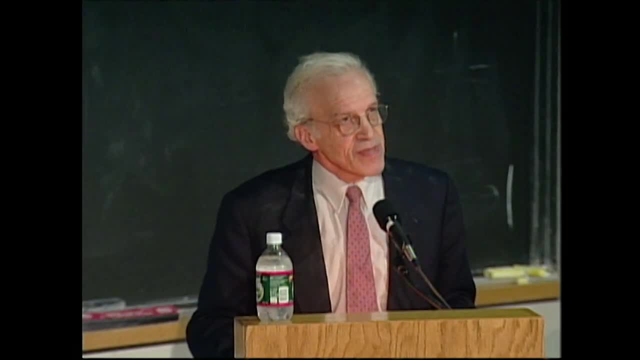 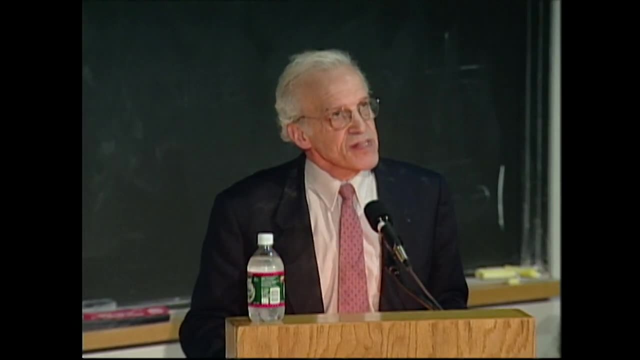 He invented the Oppie-Pritchard trap, He did the seminal work on what's called the Mott, which is the workhorse in that area, And in 1990, he invited Wolfgang Ketterle to come as a postdoc to work with him on atom. 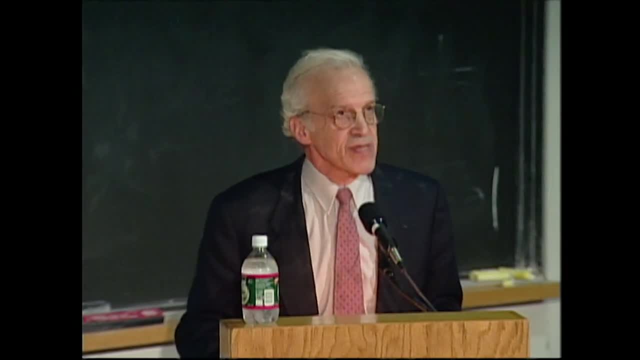 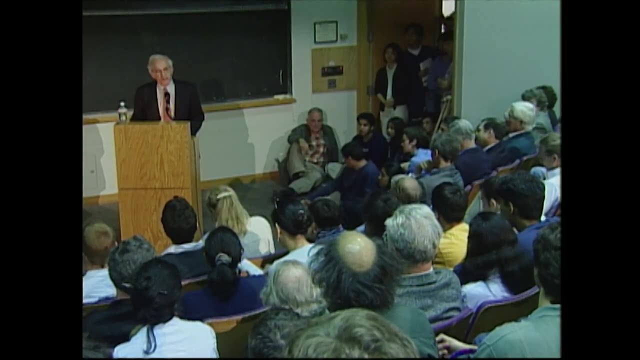 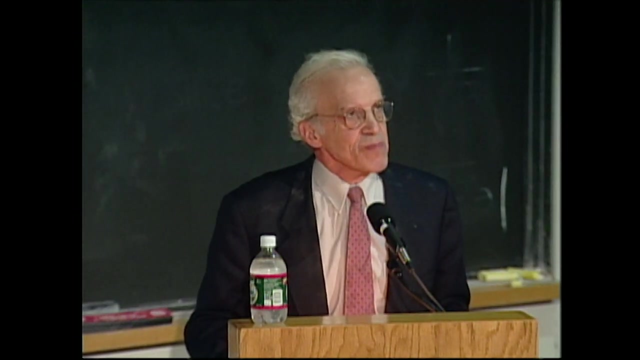 cooling, even though Wolfgang had no background in that area. He spotted Wolfgang's qualities, and the two of them together did such fabulous work that it was clear that Wolfgang was headed for great things. But not at MIT, because we could not appoint a young faculty member who would be in competition. 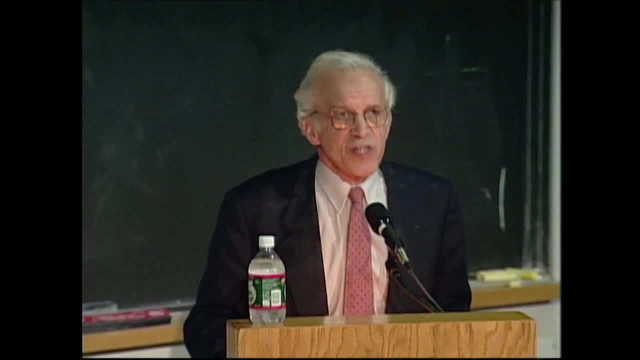 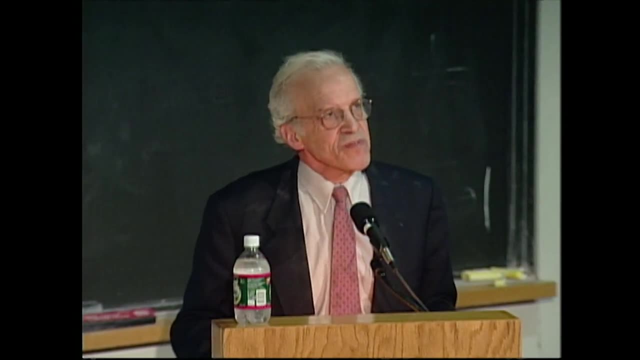 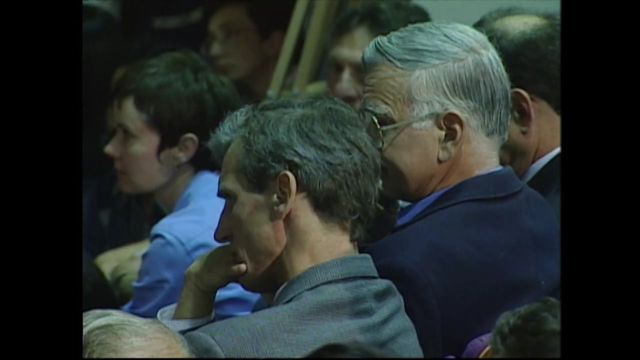 with a senior faculty member or who would really be in close collaboration, because we expect our faculty to be able to work independently. Dave overcame that obstacle by withdrawing from the field and turning over his equipment to Wolfgang, so Wolfgang could start out his work towards Bose condensation at top speed. 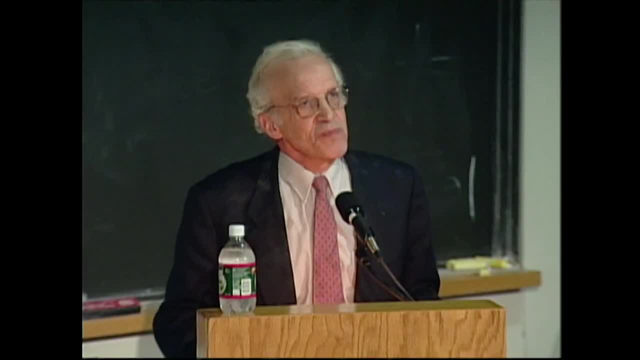 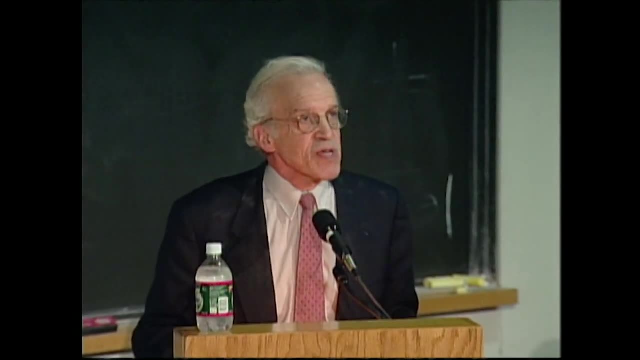 And the rest of that is history and you will hear more about it. But to me, this example of mentoring, which is to leave a field in which you're very interested in doing outstanding work to make room for young talent, is in the very best tradition. 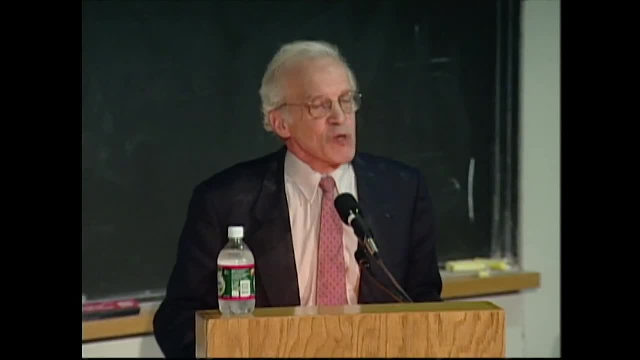 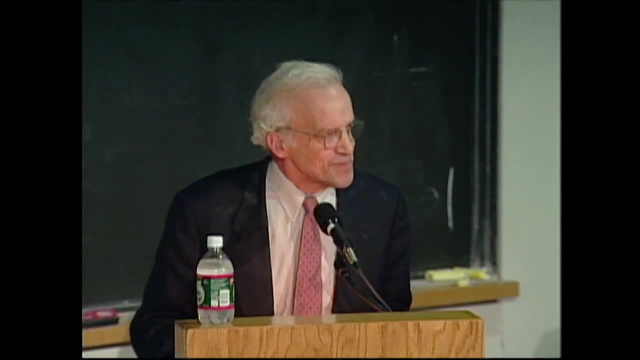 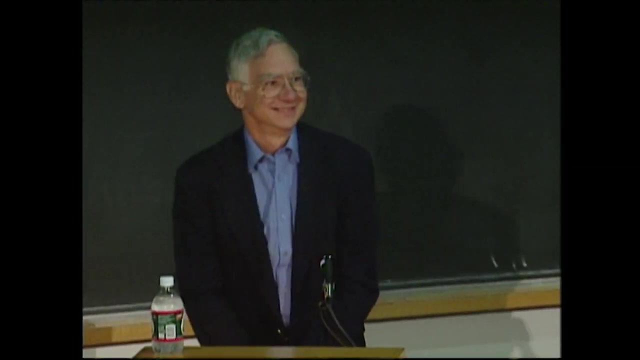 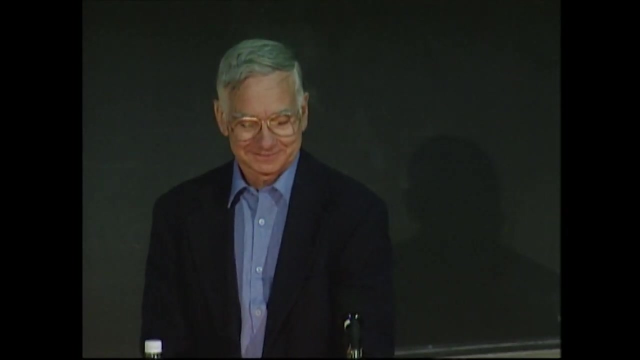 of science and of teaching, and, I hope, in the very best tradition of MIT. So with those thoughts, I would like now to introduce to you Dave Pritchard. Well, thank you very much, Dan. By my count, this is the fourth time that Wolfgang has given an MIT physics colloquium. 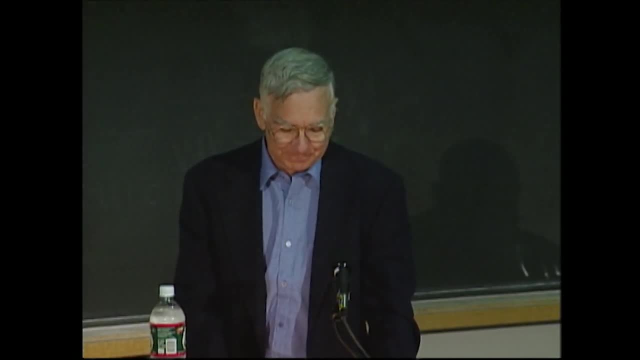 here in the six years since he's been on the faculty- and I'll give you seven now. This is a sign that well, it's actually in the past six years. this is a sign that MIT has recognized his worth somewhat before the Nobel Prize Committee. 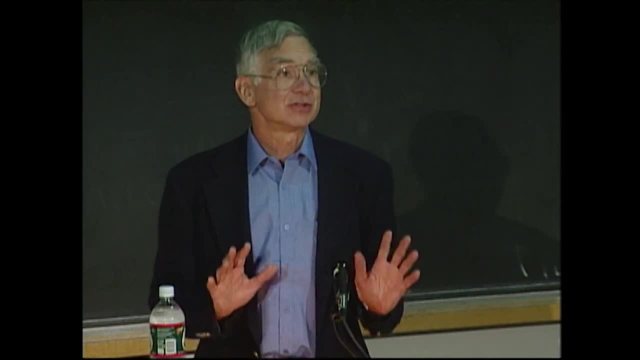 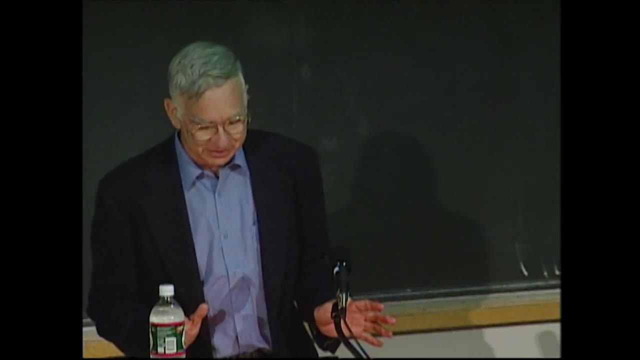 Since I've had the honor of introducing him three times, I thought I might just summarize those introductions to give you an idea of his growth. Now I know some of you are saying: wait a minute, three introducers and now three introductions. 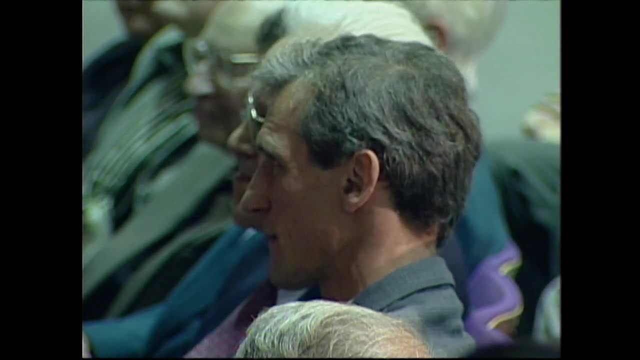 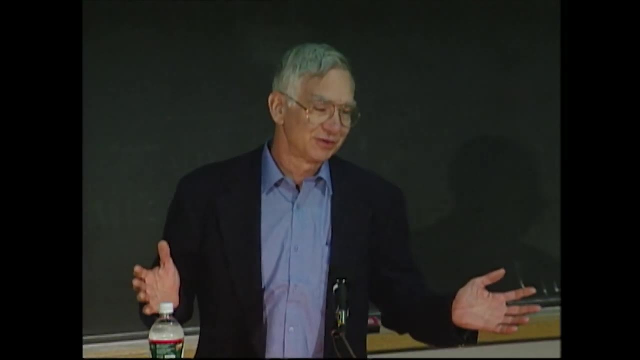 But it's OK, because we discussed it and we realized that if each one of us talked a factor of three longer than the first, than the previous speaker and Wolfgang followed suit, he'd still talk for more than 2 thirds of the time. 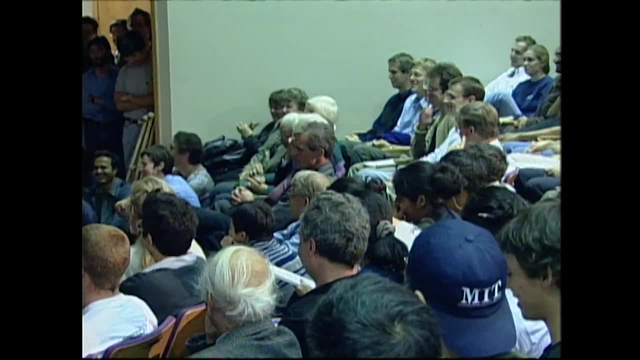 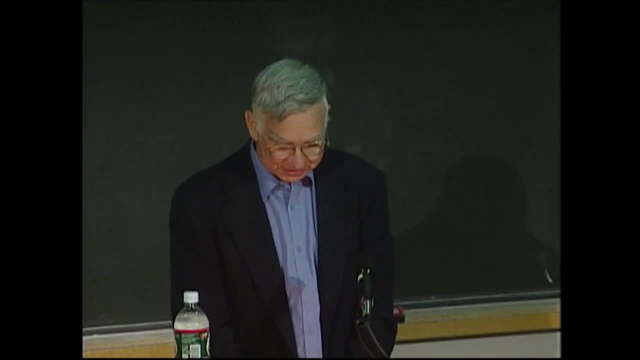 You can work that out. So in the first introduction I said Wolfgang was my postdoc and we were fortunate to get him here to take over running my cold atom apparatus, because he can run it so much better than I could. As expected, he has made fantastic progress now, having made an observation of BEC. but 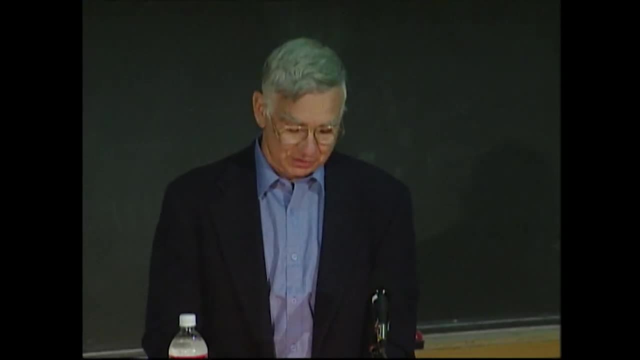 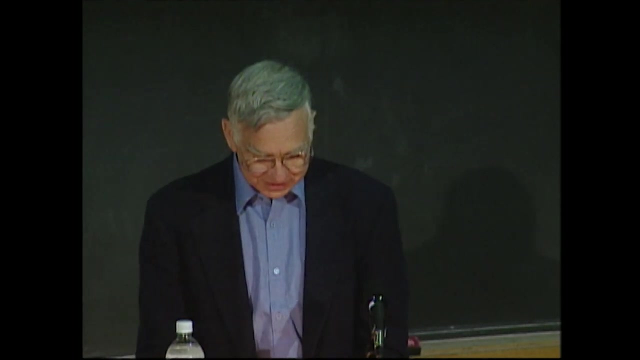 with orders of magnitude more atoms than the condensate that Eric Cornell made at GILA. And the second introduction. introduction not too much, but a year later. I said: Wolfgang is absolutely courageous, With the best BEC, the biggest BEC in the world, and with his phone ringing off the 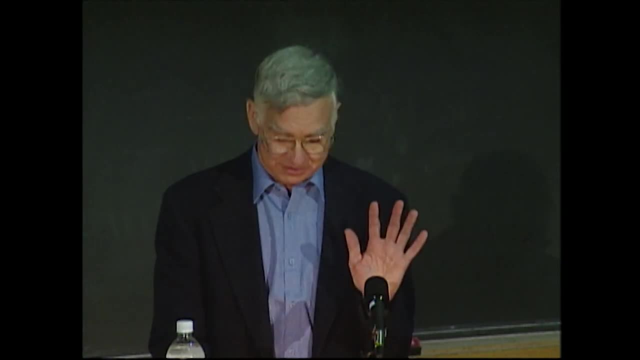 hook with the invitations. neither of these is an irrelevant concern for a professor who doesn't have tenure. He decided to scrap his magnetic trap. He felt that a new cloverleaf magnetic trap that he designed would allow for better scientific studies of the condensate. 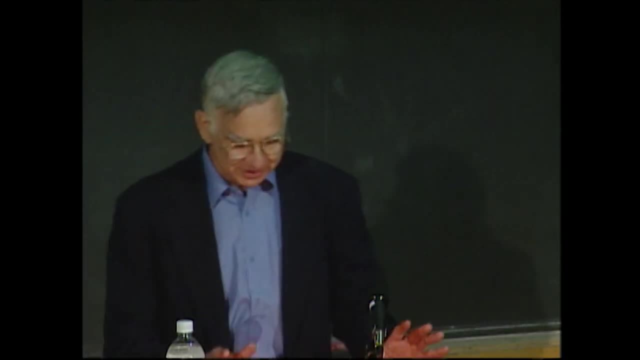 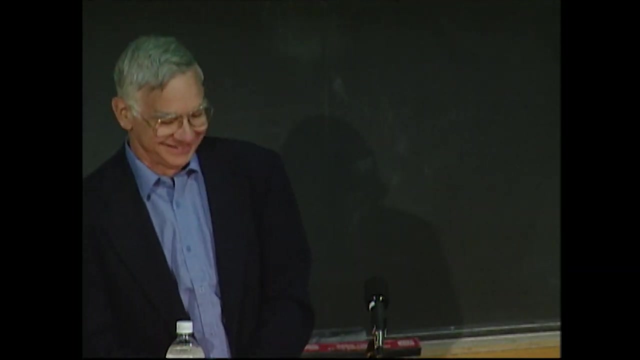 As usual, he was right and so on. so you want to hear it. so that was the second one. The third time I said Wolfgang Ketterle needs no introduction. He was just promoted from assistant professor to full professor in a single jump and he 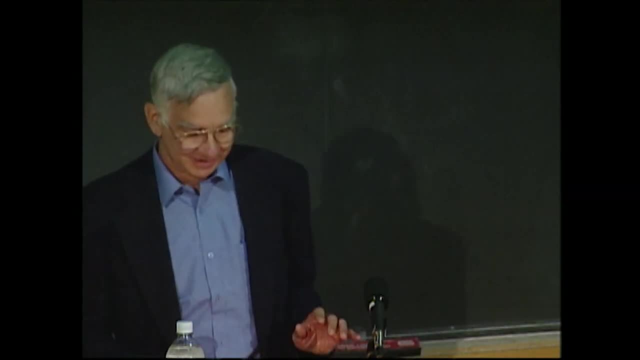 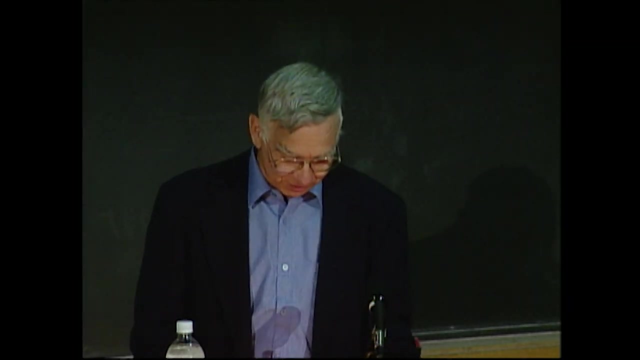 justifies this by doing spectacular research and so on and so forth. Now when I hear the trite phrase needs no introduction, I often know the speaker myself and I then agree, of course, with the introducer, But it always raises in my mind: 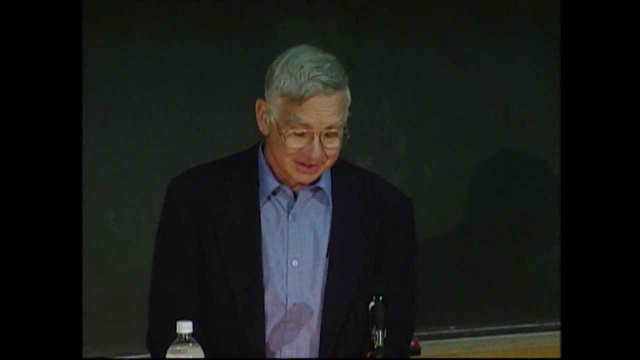 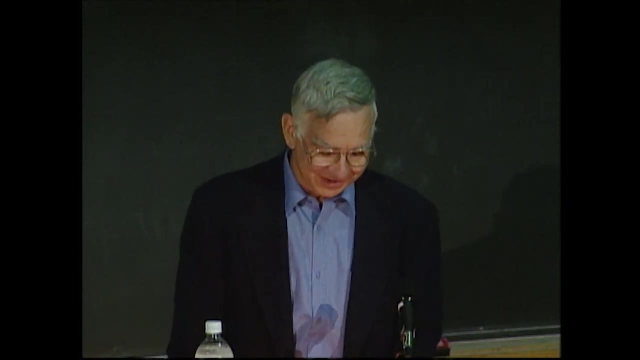 The question: well, who's this guy? who's doing the introduction? Doesn't he need an introduction? And at this fourth introduction I see that the relative stature of Wolfgang has grown so disproportionately that many other people are now concerned with this issue and that 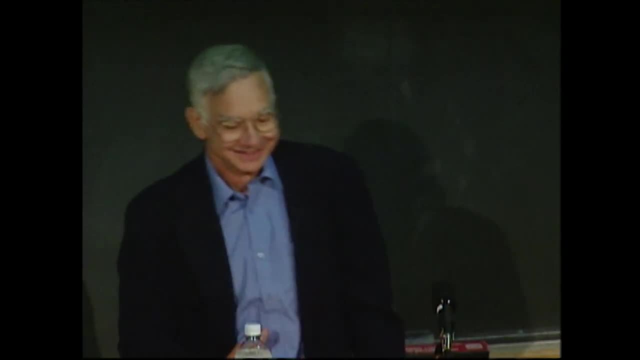 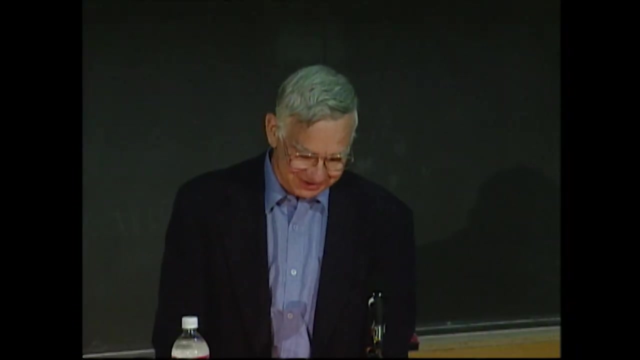 obviously explains today's format, where there were two guys who introduced me Occasionally. I feel that I should try to retain some of my mentorship skills. I think that's a good thing, A vestige of that, and so I try to challenge Wolfgang to get even better. 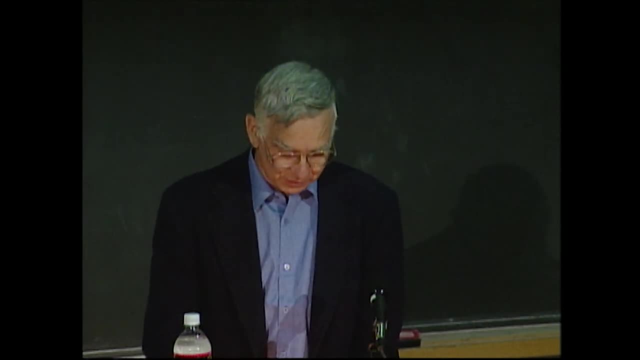 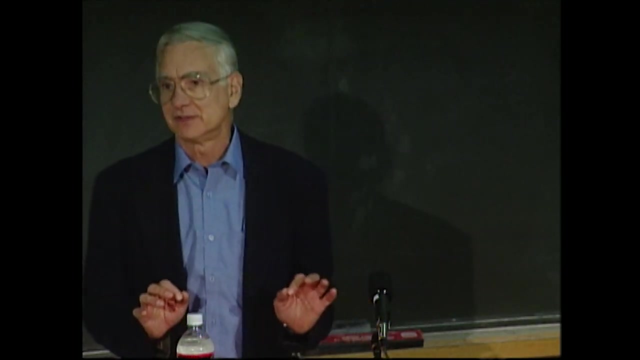 This is really difficult to do because of all the people that I've worked with, which so far includes six Nobel laureates, he's the only one who is A-plus at absolutely everything: Scientific taste, design, organization, group management, writing, scientific talks, public. 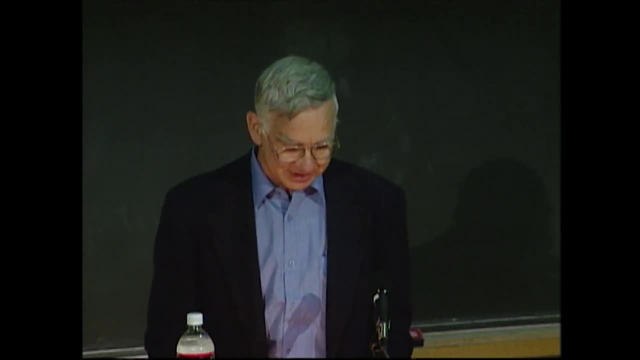 lectures A-plus. So challenging is like saying, well, very good about jumping over all those barriers, Very good about jumping over all those tall buildings with a single bound, But if you could learn to jump over whole cities you wouldn't crush so many automobiles. 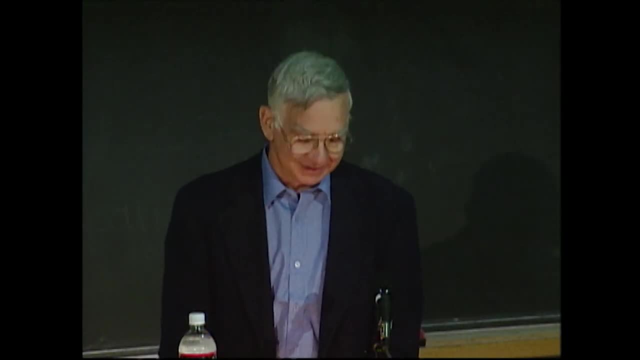 Now, previously I've challenged him by guaranteeing that he would give a spectacular talk And actually today I can raise the bar simply by challenging him to do that again, because I know that this is a week where he hasn't had much sleep and he's had numerous distractions. 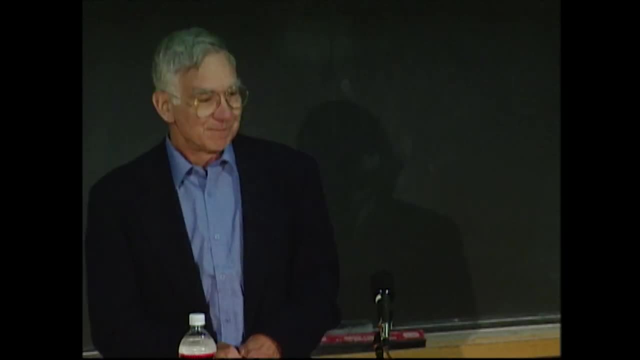 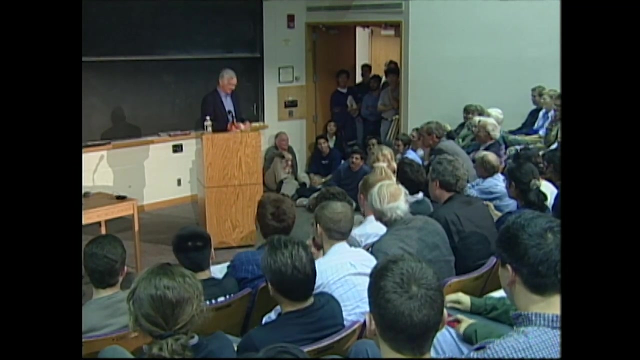 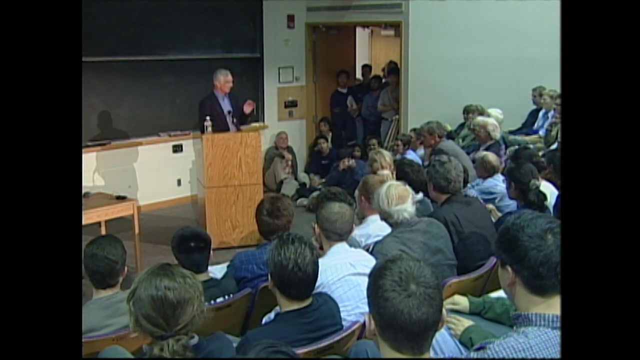 from the press and from many interviews, But I'm sure that he's up to it. One final note, Just from my personal perspective. I want to say that your most important A-plus ability is as a colleague and friend. My world has been tremendously brightened since you walked into my lab and I'm glad. 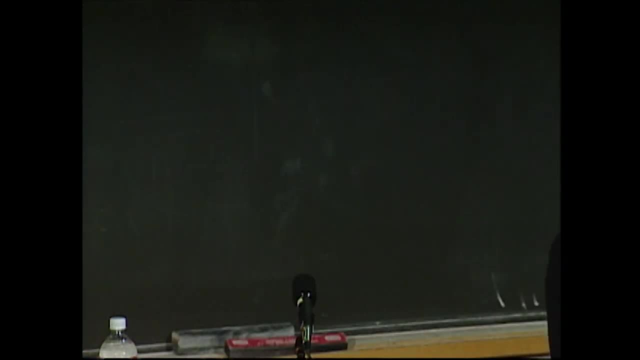 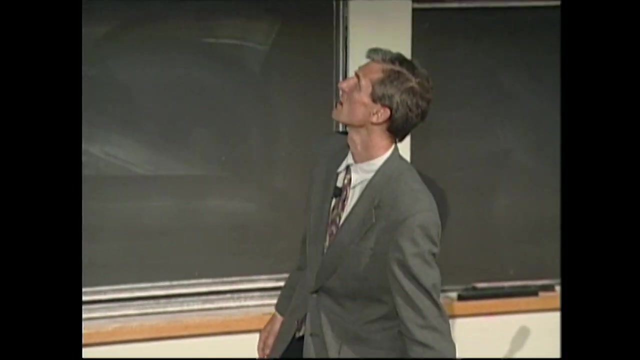 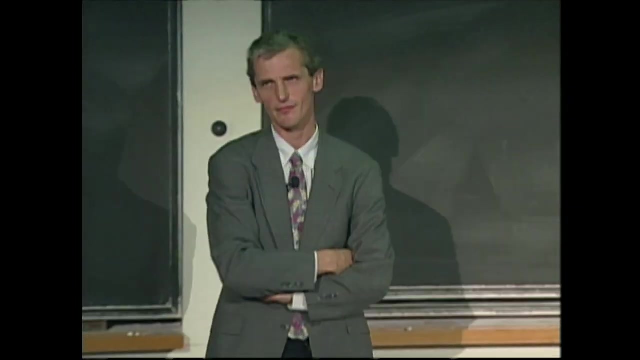 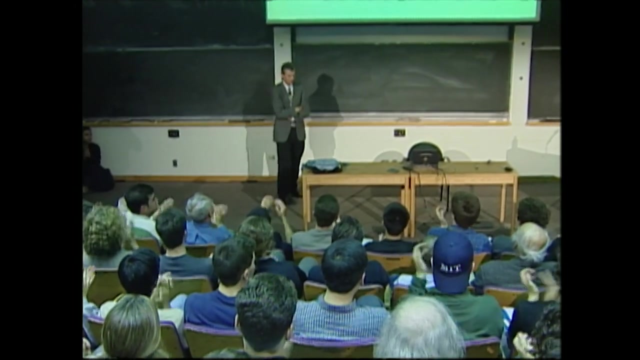 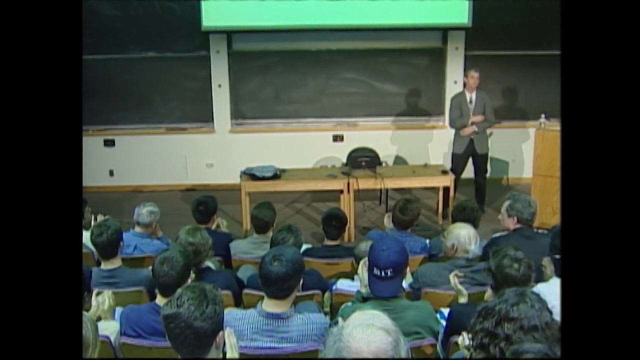 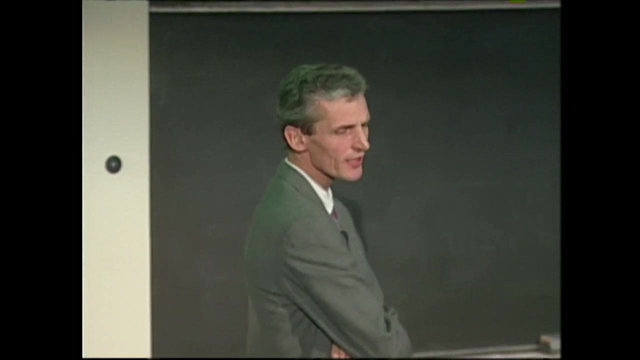 to see that MIT is the same way, And I think, for MIT, that you'd be the same, though, and the opportunity that we see is really in herausst waving. That's actually what's really happening in this room. Welcome, Welcome. It's my pleasure to introduce Michael. 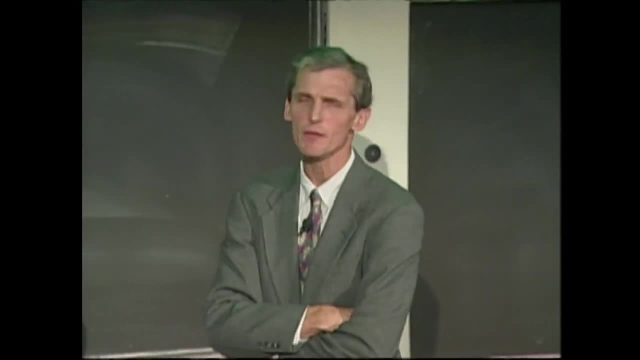 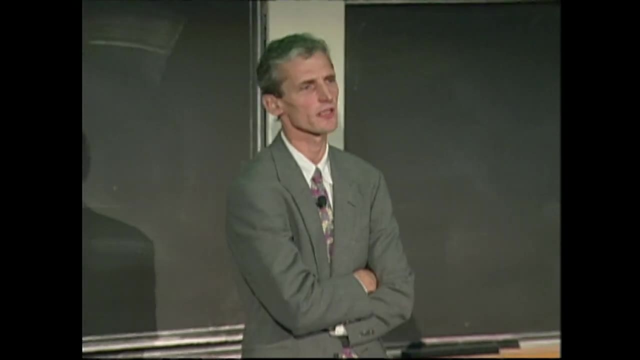 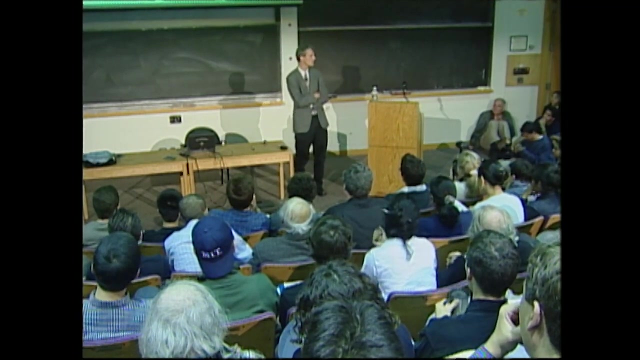 Thank you very much. what great mentors I've had And sometimes I feel I was privileged to finish what those people have started And you will see that in my talk. But I think you've also heard from those introductions that this place and the atomic physics community or the physics 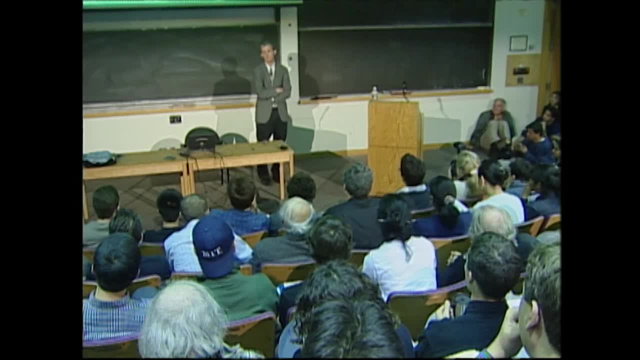 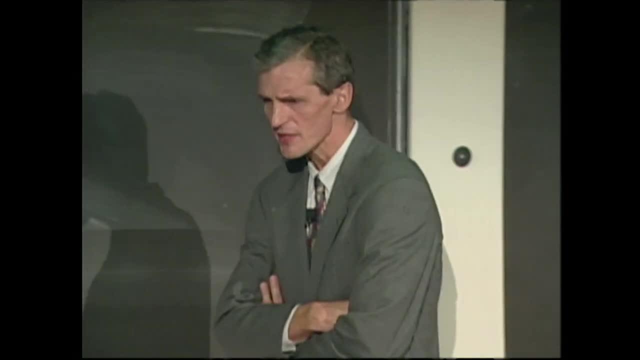 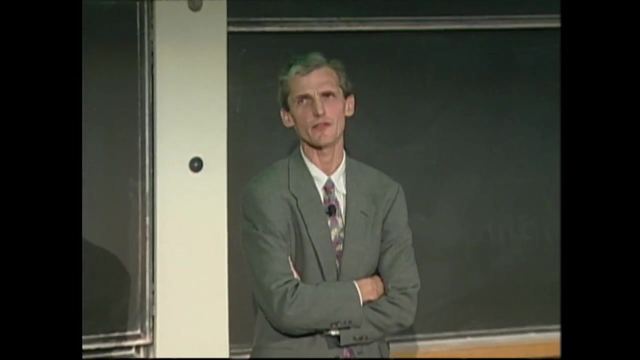 department is an inspiring and friendly environment And it is this environment which brings the best out of us. Now Dave was raising the bar by saying, by sort of announcing an A-plus talk. I think this talk, for me, has two superlatives. 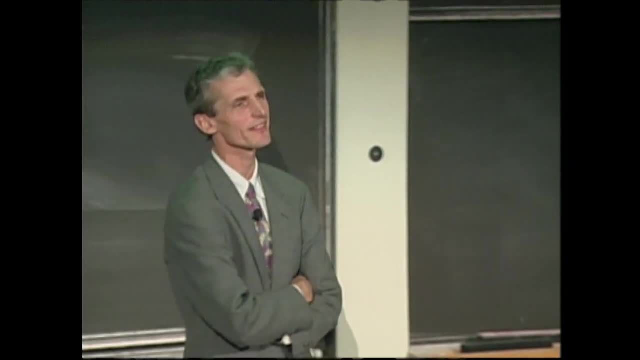 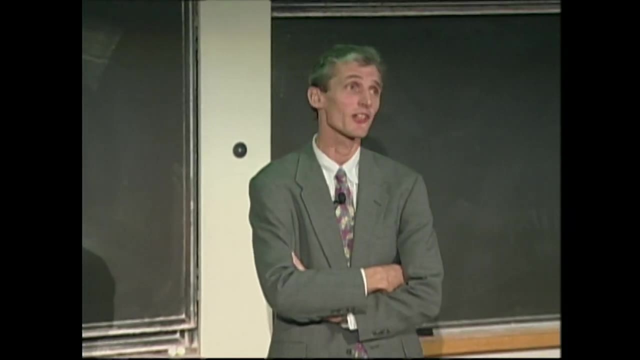 Number one: it is the best attended lecture I've ever given, But now I'm embarrassed to say. number two: it's the worst prepared one, Because I was given very short notice And I thought so well, I just put a few view graphs together. 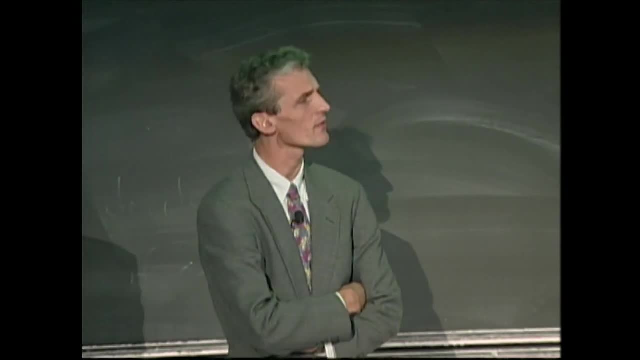 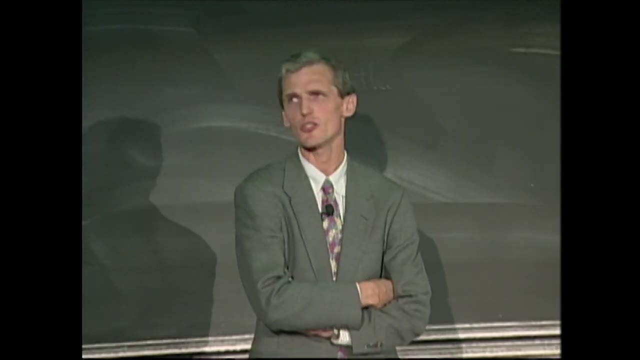 But the closer this talk came, the more I felt it's a very emotional talk for me, Because this is my family, This is my place And I want to tell a story and not just give a talk on our recent results. So I tried to prepare something special. 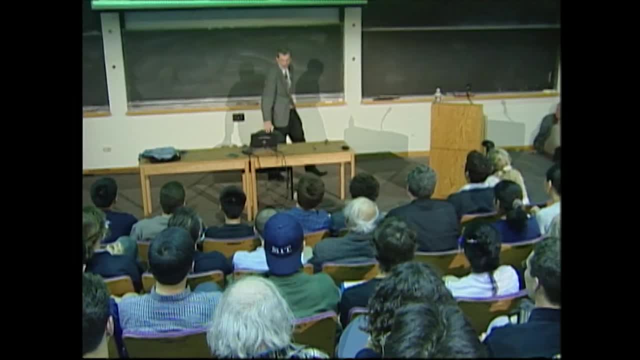 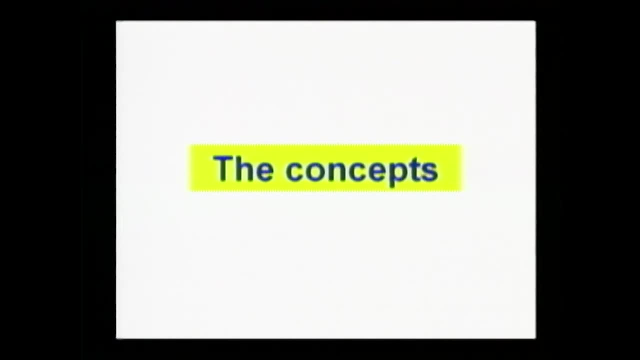 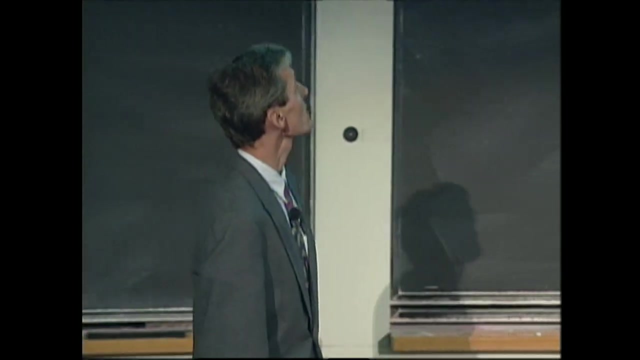 but I couldn't really polish it, So let me tell the story of Bose-Einstein condensates, which is the coldest matter in the universe. And since I know here's a broad audience, I want to be explicit in one of the concepts. 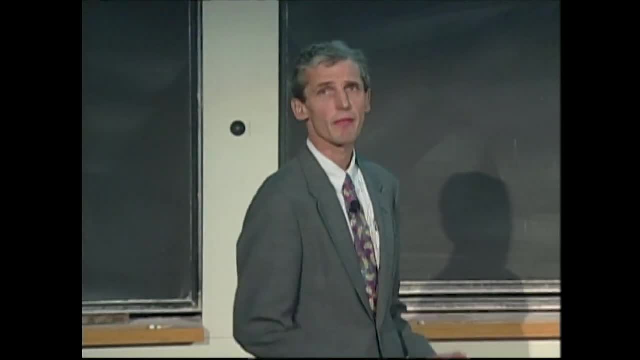 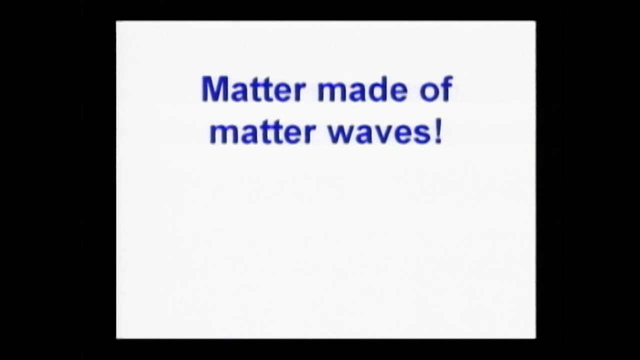 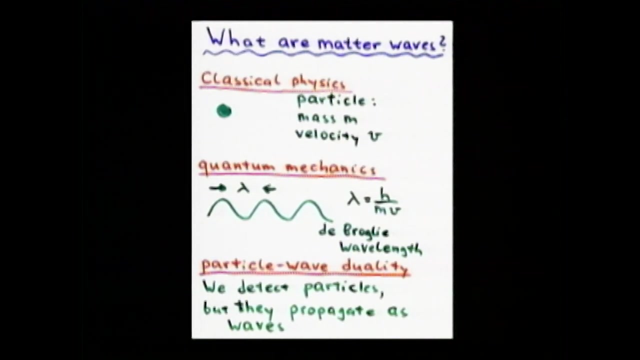 So the Bose condensate. you can regard it as matter made of matter waves. It's a form of matter where the quantum mechanical nature, the wave nature of matter, manifests itself at a macroscopic scale. So you're all familiar with- or most of you, I hope- 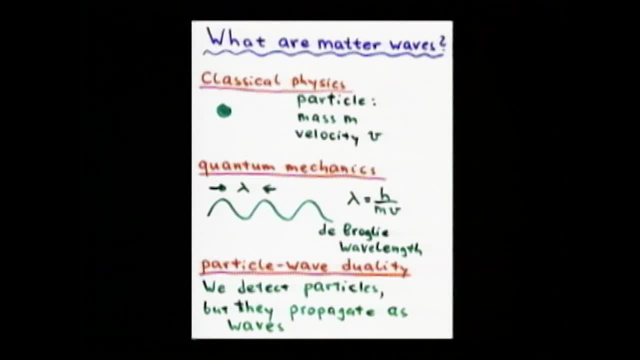 with a particle wave duality for light, for photons, But we have the same particle wave duality for all particles. We know from the early days of quantum mechanics that a particle which is classically characterized by position and velocity- The velocity should rather be described- 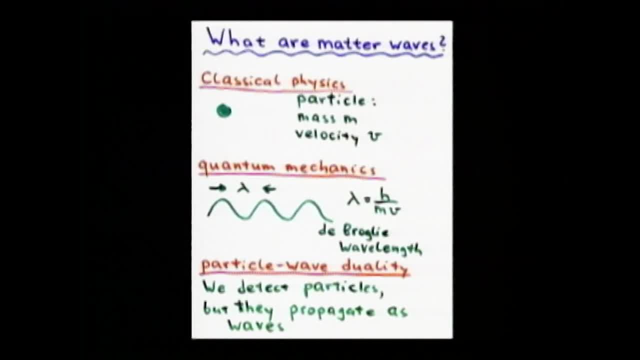 as a quantum mechanical wave, a de Broglie wave, And the wavelength of the de Broglie wave, of the quantum mechanical wave, follows the famous de Broglie relation. It's inversely proportional to the velocity of the particle. 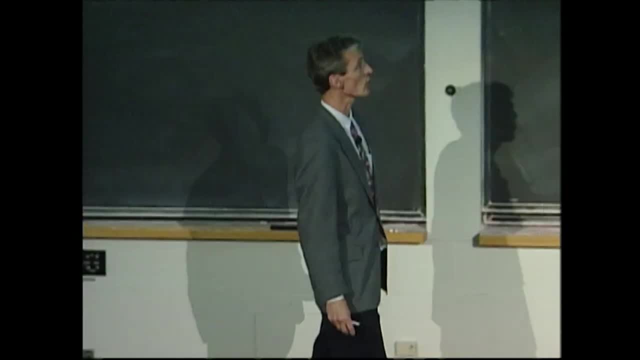 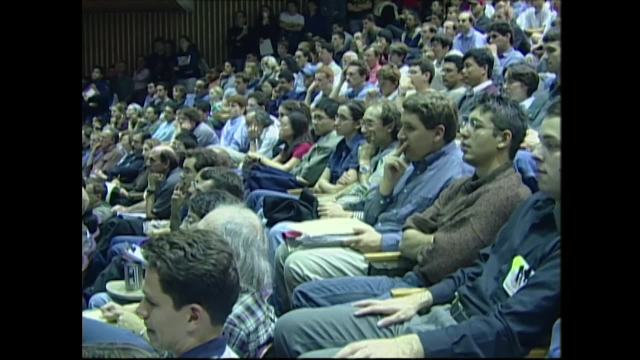 And I know when we learn physics we all struggle with the concept that particles are all objects- You and me- and microscopic objects and macroscopic objects are waves and particles at the same time. Particles propagate as waves, but when we detect them, 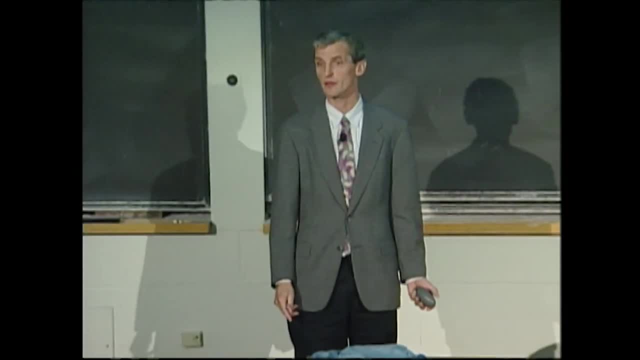 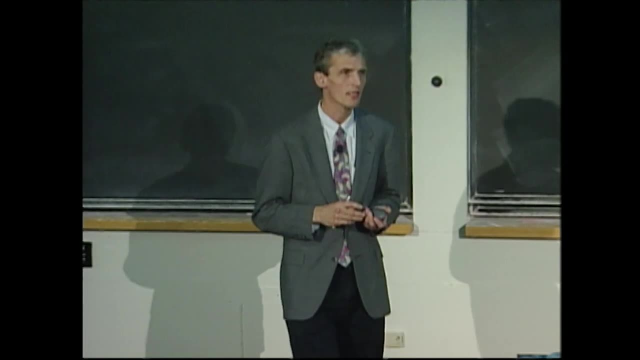 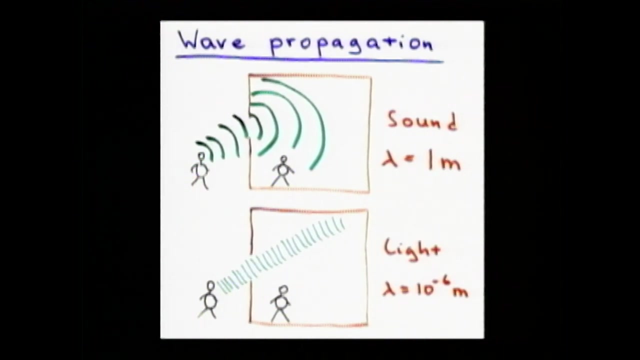 it makes click in a detector. So well, if you and me, if we are all waves, why don't we perceive the wave nature of matter in every day's life? So let me raise you, let me raise the question: how do we perceive if something is a wave or not? 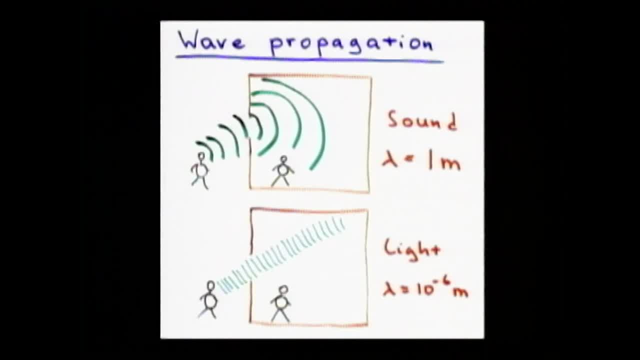 So if I would challenge you and say: explain me why sound is a wave, a very reasonable answer would be: if there are two people who talk to each other, they can hear each other even if they don't see each other, because a wave propagates, deflects around corners. 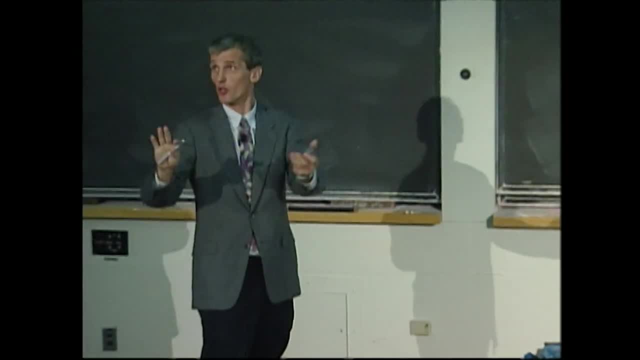 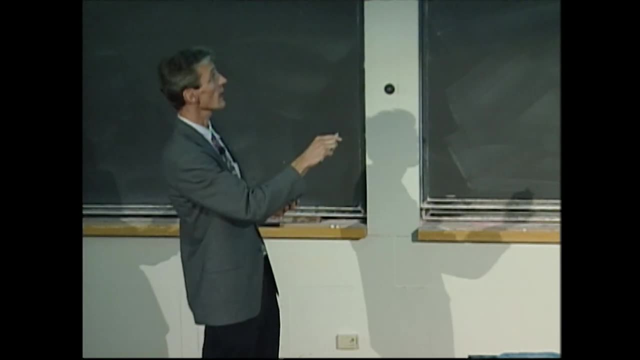 If I would ask you what happens in the case of light? You all know that light is an electromagnetic wave. It's not so obvious because the wavelength of light is so short that light is just deflecting a little bit and you can't really perceive the wave nature of light. 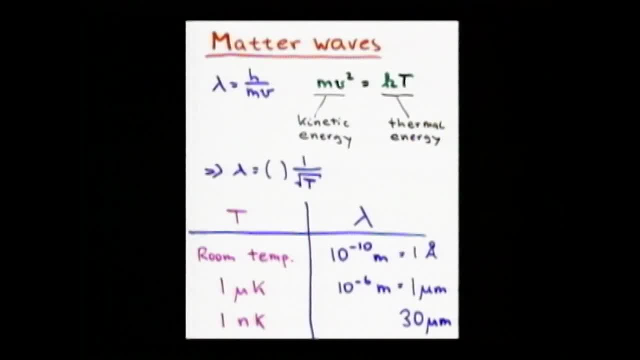 very easily. But now, in the case of matter waves, the wavelengths are even shorter. The wavelength is given by the de Broglie relation, and the velocity of a particle is determined by its temperature. So from that we know that the colder the temperature. 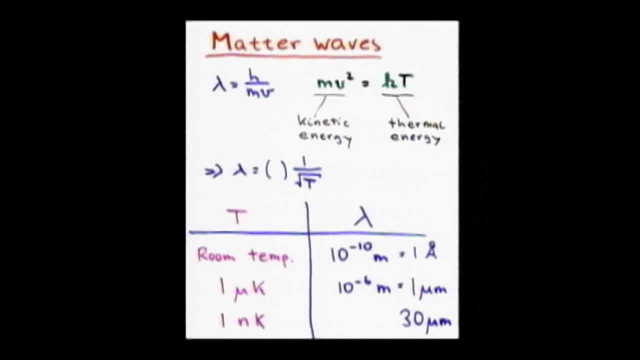 the longer is the de Broglie wavelength. Now, talking about atoms at room temperature, the matter wavelength, the de Broglie wavelength, is smaller than the size of an atom. So therefore, the wave nature, the way, the nature of atoms, is not manifest. 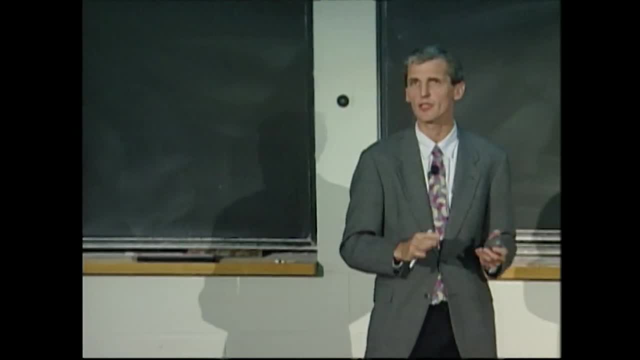 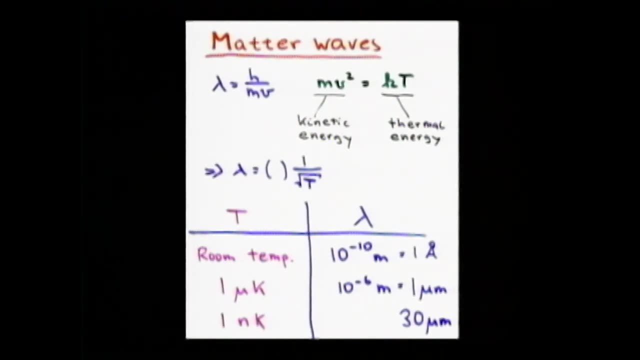 But now we can cool down, and the title of my talk is the coldest matter in the universe. We cool down to micro and nano Kelvin temperatures more than a million times colder than interstellar space, And the de Broglie wavelength becomes longer and longer. 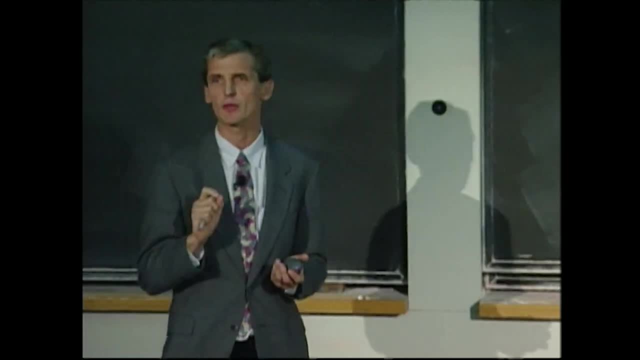 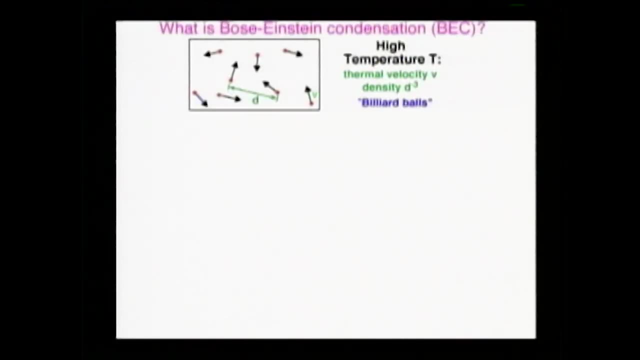 And this value is 30 micrometer is a fraction of the diameter of a human hair, So it's really getting macroscopic. And this long de Broglie wavelength, they are at the heart of the phenomenon which I want to describe Bose-Einstein condensation. 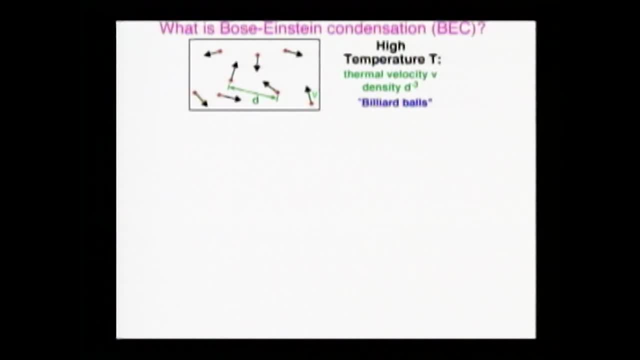 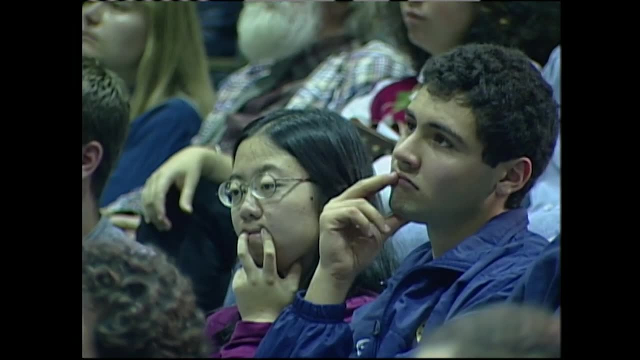 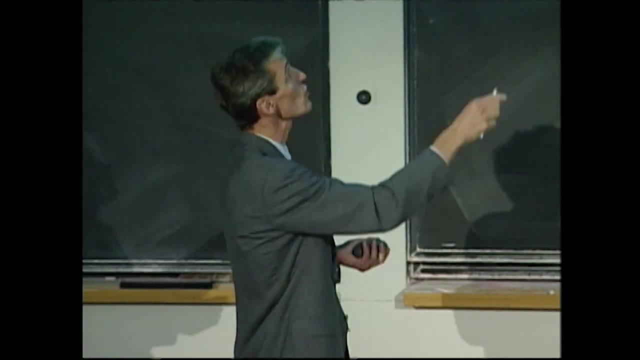 What happens if you take a gas in a container and cool it down? The particles slow down. As I just mentioned, we shouldn't describe the particles as sort of little billiard balls. They are wave packets. They are quantum mechanical waves, But as long as the wavelength is very short. 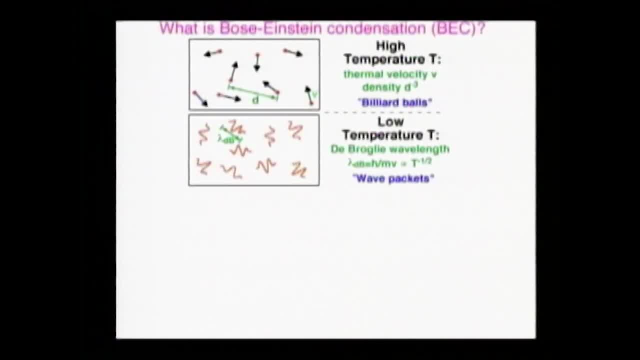 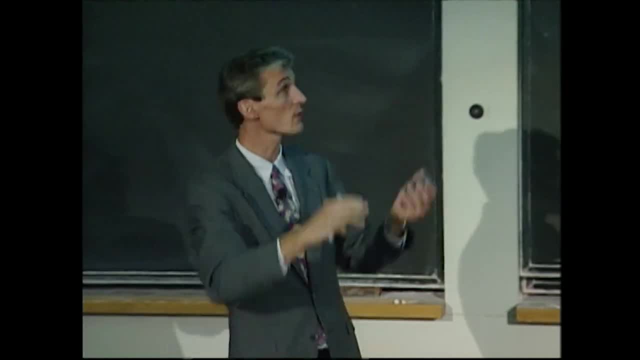 those wave packets are very localized and we can follow the motion of those wave packets As if they were particles. But now we can cool down. The de Broglie wavelength becomes longer and longer And when we reach the point where the wave packets, where 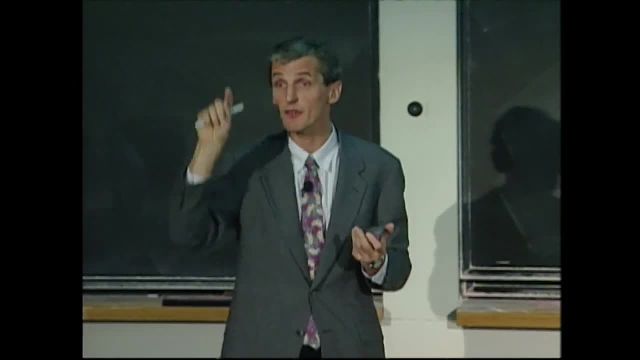 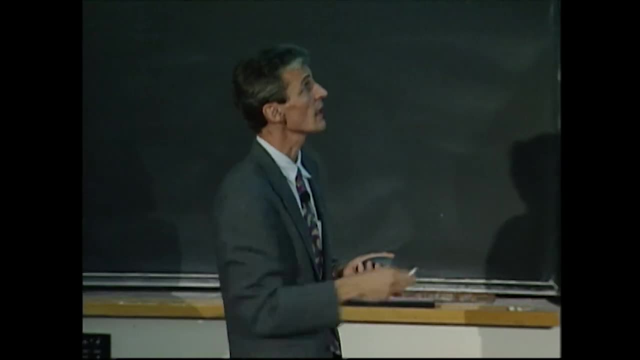 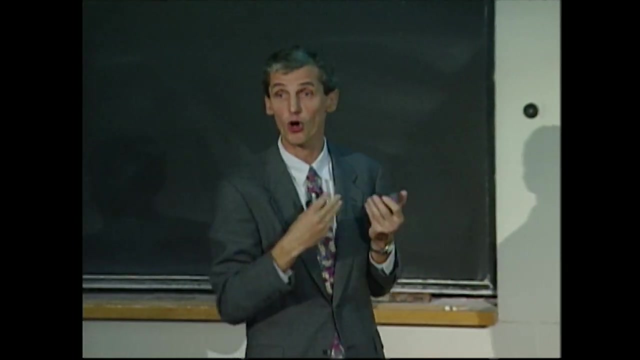 the de Broglie waves overlap, then we cannot follow individual particles anymore. They become sort of a quantum soup of wave packets. And it's exactly at this point, when the wavelengths- the de Broglie wavelengths is comparable to the spacing of particles- that a new form of matter forms. 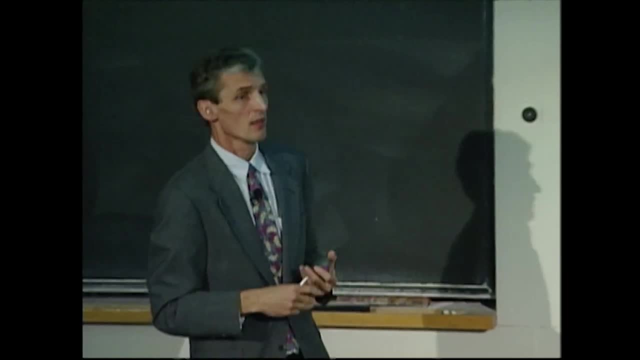 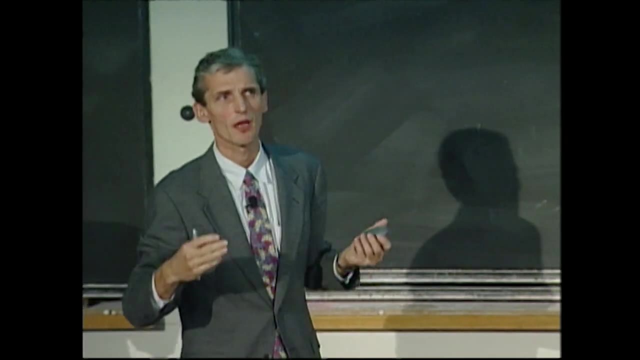 And this is the Bose-Einstein condensate. Or to say it again: if the de Broglie wavelengths become longer and longer and those matter waves overlap, then all the particles in the gas, they start to oscillate in concert. 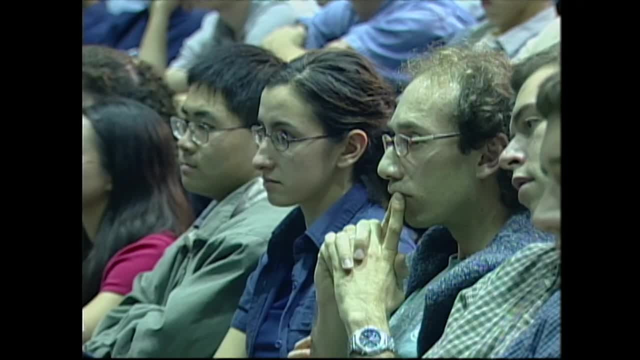 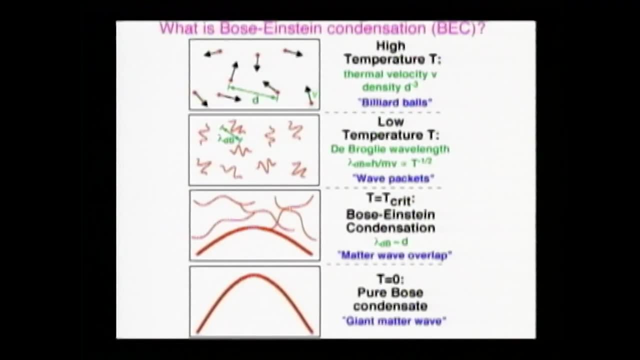 And what they form is one giant matter wave, And this is the Bose-Einstein condensate. Just to use an analogy, the difference between atoms in random motion and the Bose condensate is exactly the same difference as the light from a light bulb. 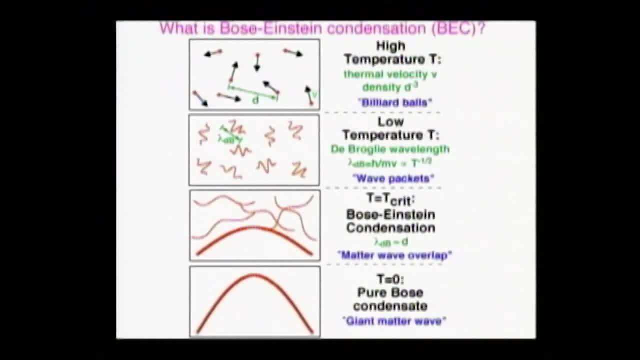 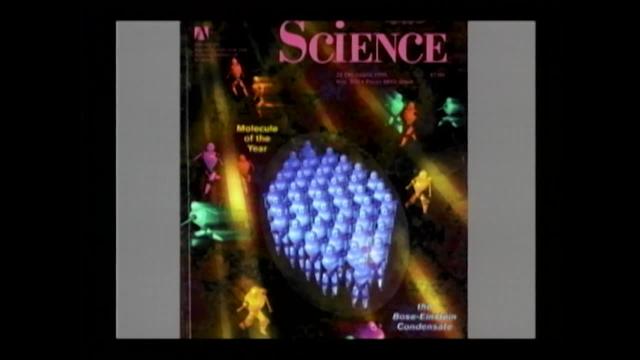 and the light coming out of a laser. So what Bose-Einstein condensate is about? it's about the creation of atoms with laser-like properties, And this is a nice artist's conception of how you can imagine the Bose-Einstein condensate. 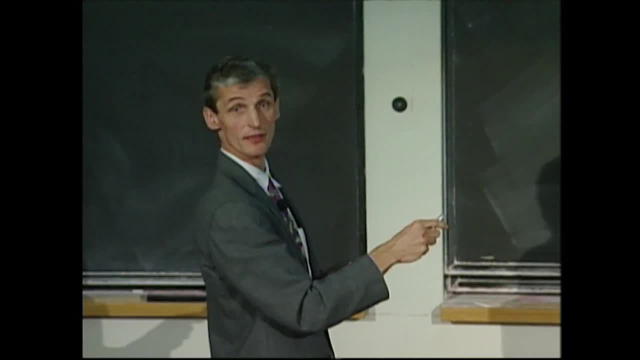 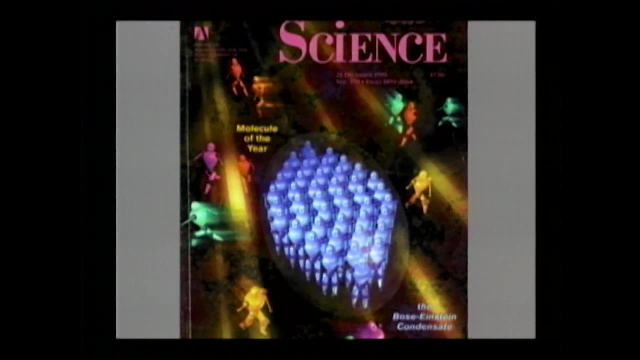 First of all, these are indistinguishable atoms. You see, they have all the same facial expression And they march in lockstep, which means they are in phase. it's a single wave function, And this is how you can imagine what happens. 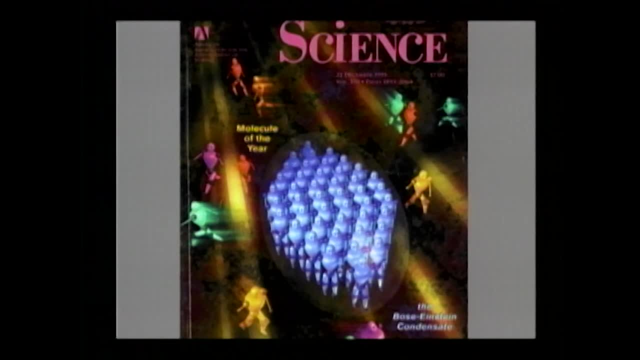 in a Bose-Einstein condensate. You also see sort of those other guys. they walk in random direction. They are not Bose condensed. They are in different quantum states and are therefore distinguishable from the atoms in the condensate. 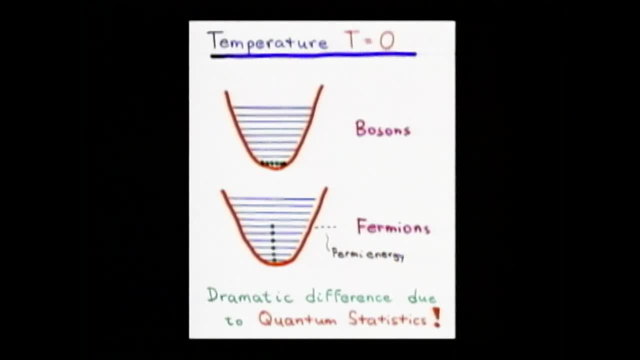 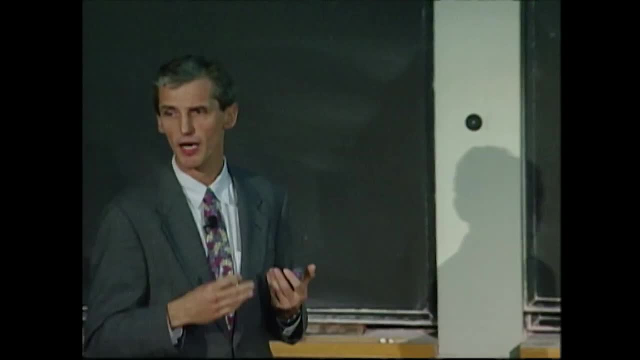 Now, of course, what I just said- that all the atoms go into one quantum state and fall in lockstep- is only possible for atoms which we refer to as bosons particles which have integer spin. I don't want to go into details here. 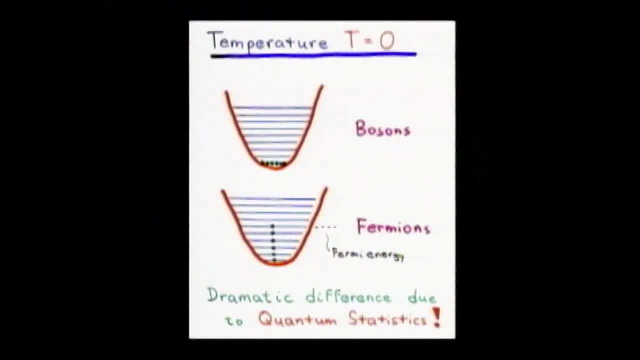 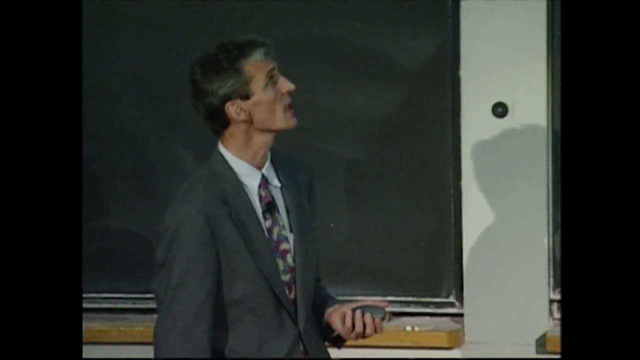 but there is another class of particles called fermions. They have half integer spin And their behavior at low temperature is completely different. So the phenomenon of Bose-Einstein condensation can be regarded as the most striking manifestation of quantum statistics, of the difference. 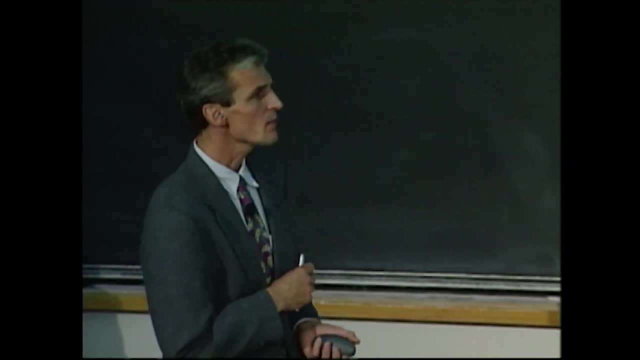 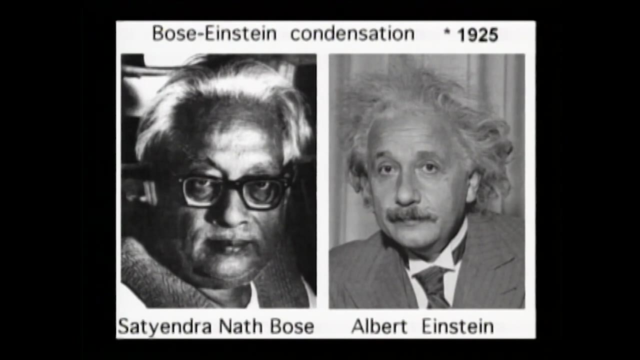 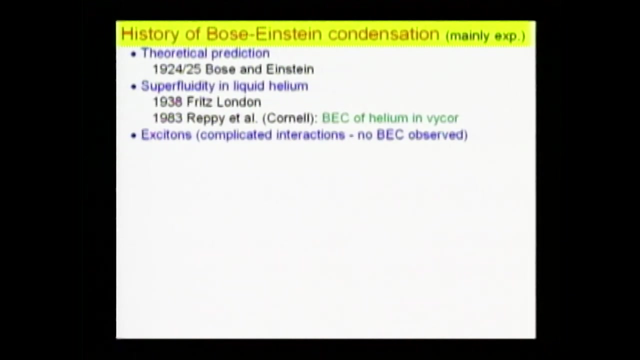 between bosons and fermions, And the name Bose-Einstein condensation is derived from those two well-known people who predicted it In the 1920s. However, Bose-Einstein condensation in a gas was not realized until 95, for reasons 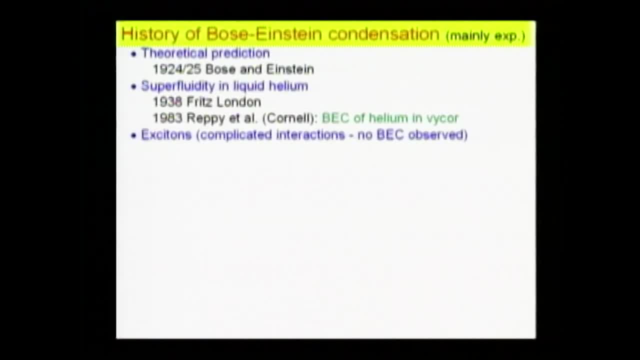 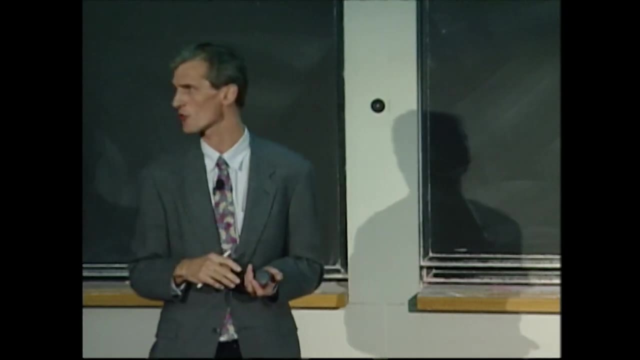 which will become obvious in a moment. So the prediction of Bose-Einstein statistics was 1925.. And for many, many years, the only manifestation of Bose-Einstein condensation was in liquid helium. The superfluidity of liquid helium is a consequence of Bose-Einstein condensation. 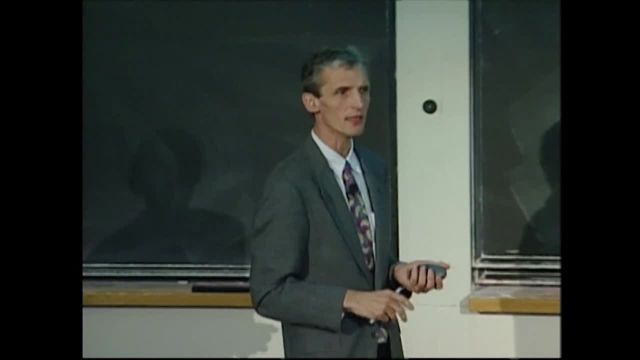 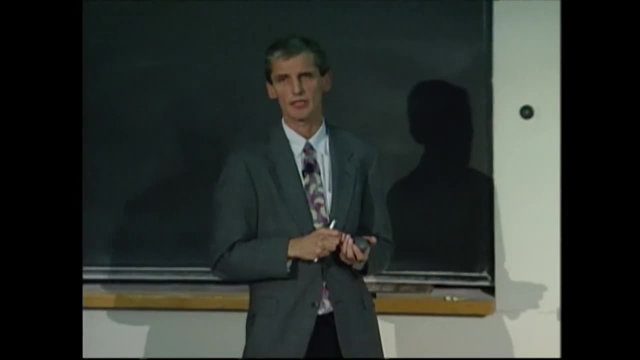 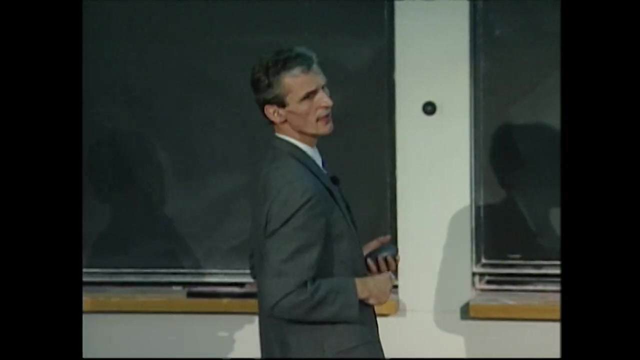 But it's a liquid, It's not a gas And there are high-density effects which modify this phenomenon greatly. But then there was an attempt to realize Bose-Einstein condensation in dilute gases, And a lot of credit for that should go to Tom Gratek and Dan Kleppner, who 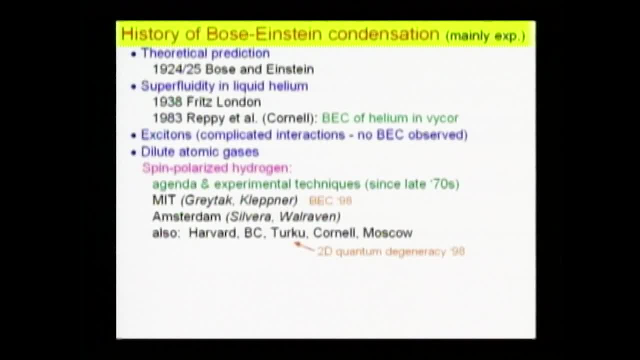 are here on the faculty. They really put Bose-Einstein condensation in dilute atomic gases on the agenda and made it a goal, And it's I'm very pleased to mention that after 20 years of efforts, they realized Bose-Einstein condensation in hydrogen. 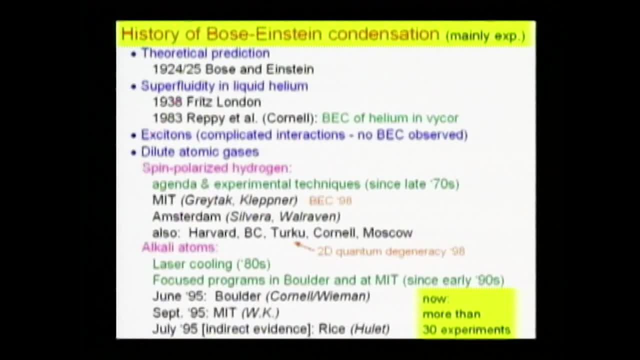 and achieved a longstanding goal. However, a few years earlier, there were new cooling techniques developed: laser cooling- I will briefly comment on them- And new systems. alkali atoms could be cooled to ultra-low temperatures And it's really the alkali atoms which 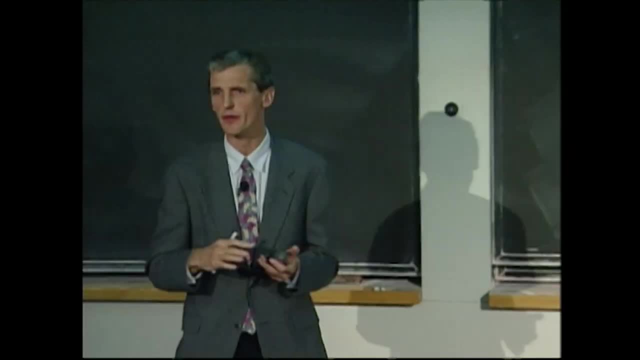 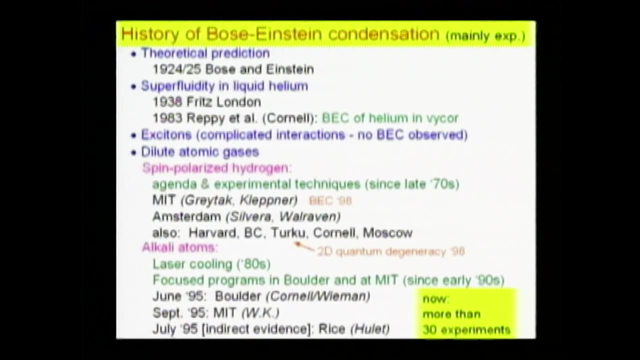 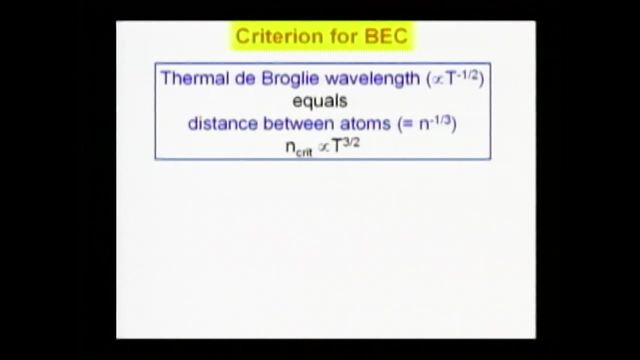 have created this whole new field of Bose-Einstein condensation with many, many activities, And the success here came In 1995, and I will tell you the story today. So well, I think, from the concepts I've presented, if you want to achieve Bose-Einstein condensation, 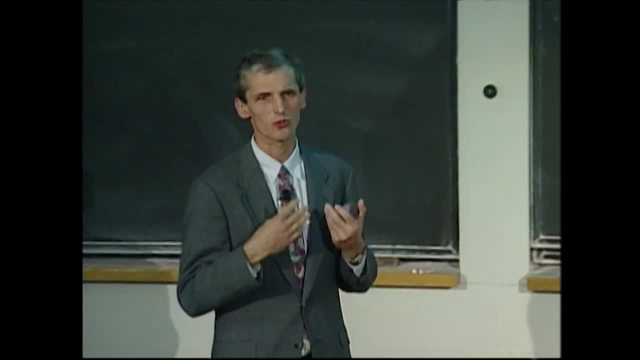 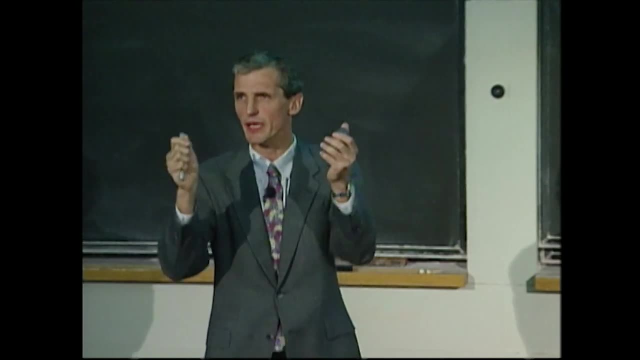 quote, unquote. all you have to do is you have to cool down the gas to micro and nano Kelvin temperatures. You have to cool it down until the de Broglie wavelength is comparable to the spacing between atoms and the meta waves overlap and start to oscillate in concert. 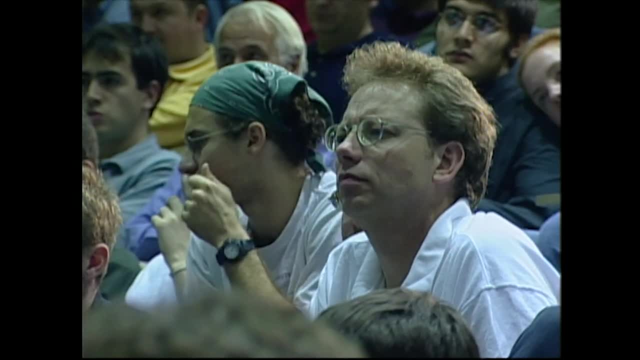 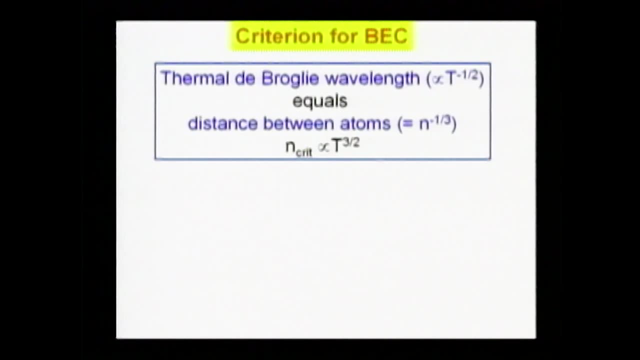 So I mentioned that the de Broglie wavelength depends on temperature, The distance between atoms depends on density, So we have an. so the transition to Bose-Einstein condensation is characterized by a combination of temperature and density. So let's just look at this relation for something. 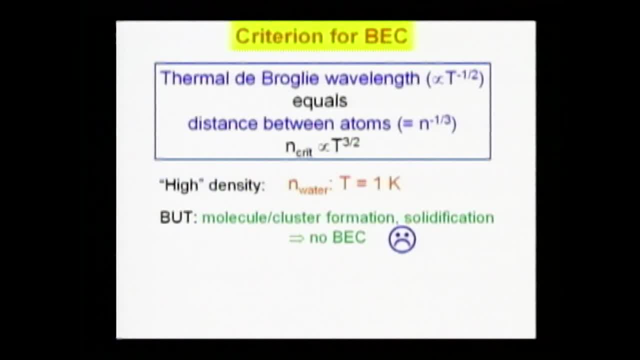 of the density of water, You would predict that the transition temperature is 1 Kelvin, which is easy to reach. However, tough luck, At 1 Kelvin everything is liquid or frozen and you can't observe the phenomenon of Bose-Einstein condensation. 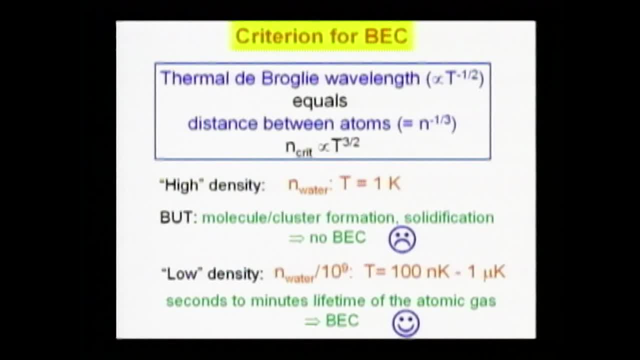 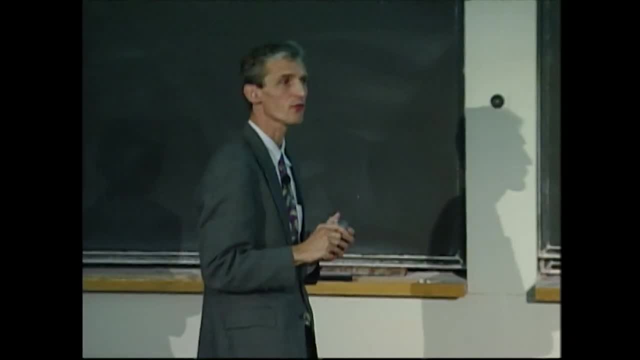 So in order to prevent that and also to prevent formation of molecules out of the atomic gas, we had to work at extremely low density. So the system I'm referring to is at a density which is a billion times more dilute than water. 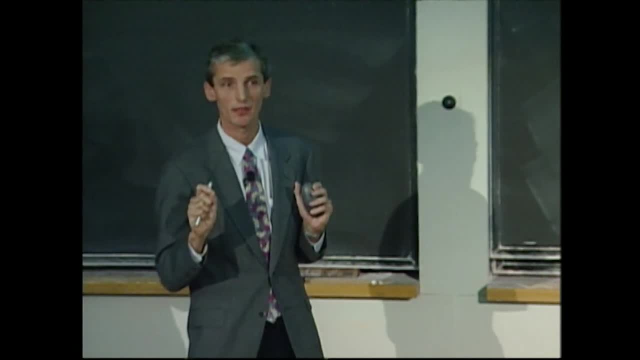 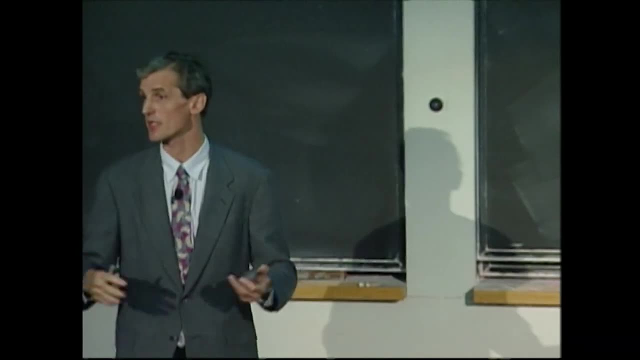 It's 100,000 times thinner than air And in those gases we can observe Bose-Einstein condensation without self-destruction, by molecule cluster formation And solidification. But there's a price to be paid If you work at ultra-low density. you need ultra-long de Broglie wavelengths to make those matter waves oscillate in concert. So we needed the lowest temperatures ever achieved. So we needed cooling methods, And what I'm actually talking about is the combination of two different cooling methods which were developed in two different sub-areas. 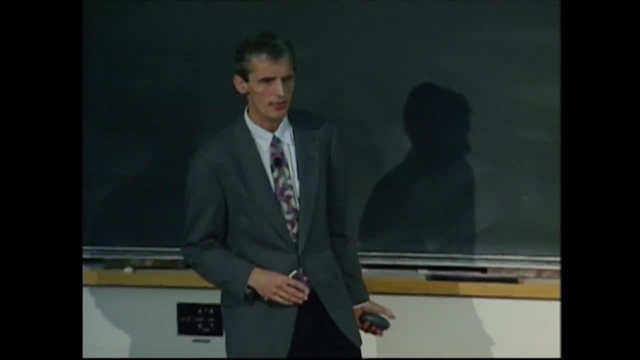 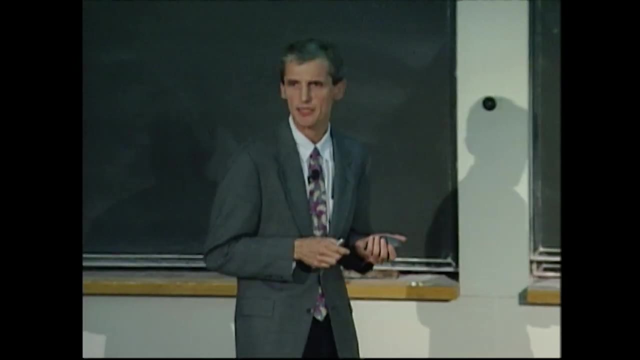 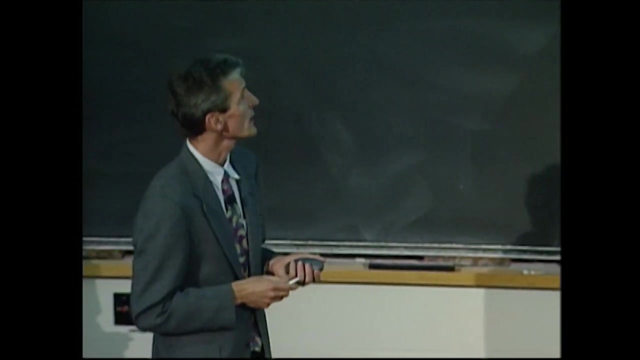 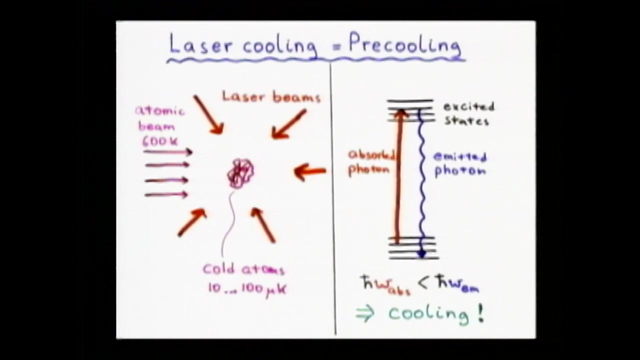 One is laser cooling. The pioneers of laser cooling, some of them were recognized with the Nobel Prize in 97. And major developments to laser cooling were also done by Dave Pritchard at MIT. The principle of laser cooling is fairly simple: You shine laser light on atoms. the atoms scatter light. 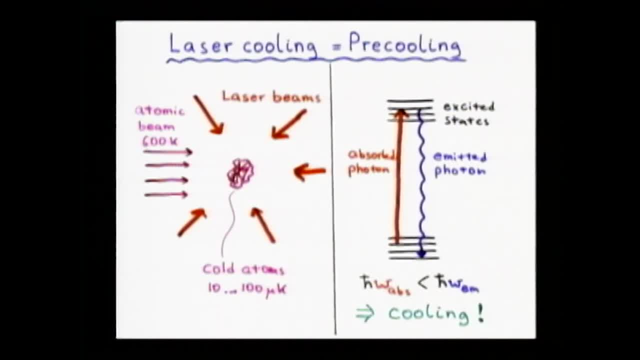 And if you play some tricks which I don't want to explain, that the light which is scattered, which is emitted, has a shorter wavelength, is more energetic than the absorbed light, then the scattering of light removes energy from the system And the system cools down. 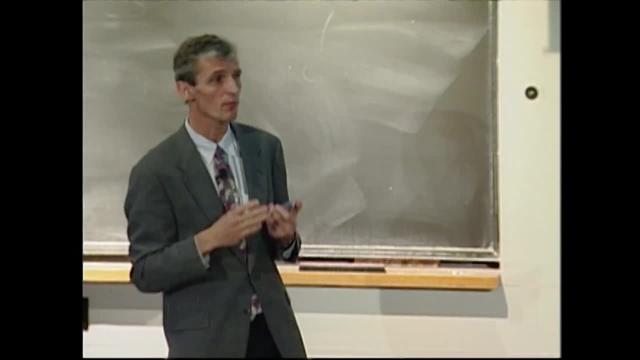 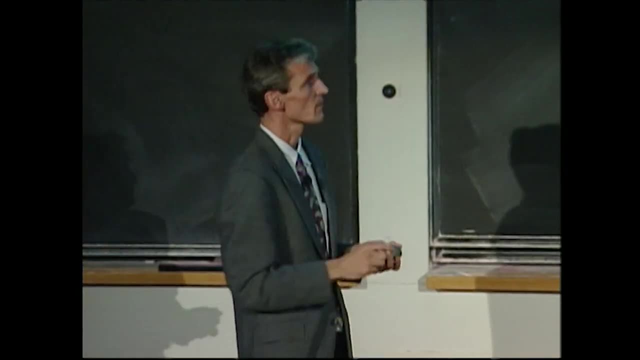 It works great. You just shine laser light on atoms and you create micro-Kelvin samples, And a very important configuration to do that is the one co-invented by Dave Pritchard, And I think this is probably one of the most important signal. 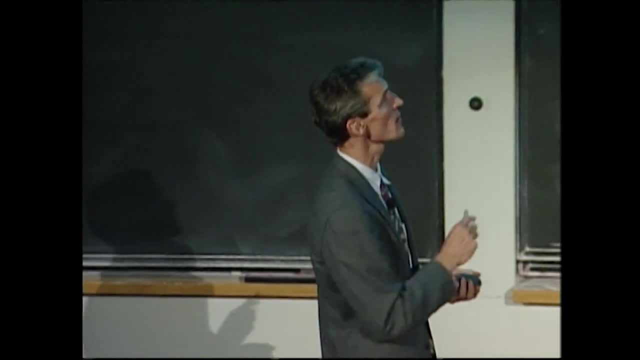 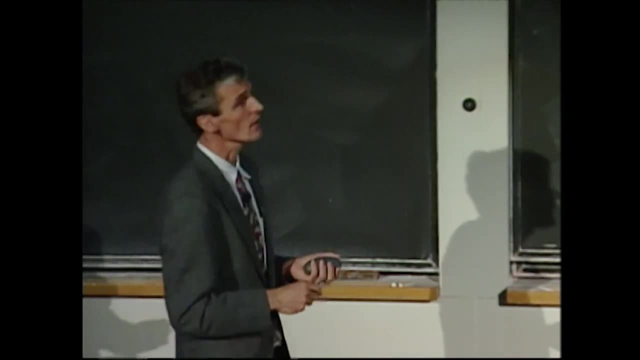 techniques which were ever introduced to the field of atomic physics: the magneto-optic trap. It is the workhorse of the whole field of ultra-cold atoms. now, So well, and if you have this configuration of laser light and shine light into a vacuum chamber and add some atoms, 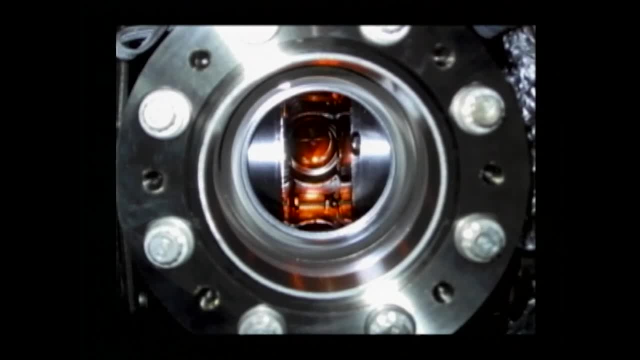 you see, this is in one of our lab. upstairs you see a small ball a few millimeter in diameter. yellow glow, So you can see with the naked eye ultra-cold sodium atoms, but at a fairly hot temperature of a fraction of a milligram. 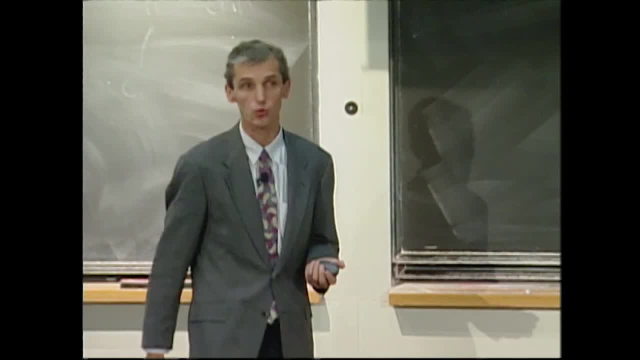 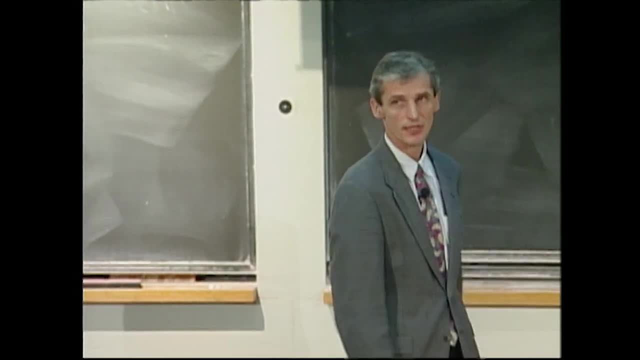 Kelvin. So this is the starting point for the next stage of cooling towards Bose-Einstein condensation. Laser cooling has so far not been able to carry atoms down to Bose-Einstein condensation because it has limitations, And some of them are very fundamental. 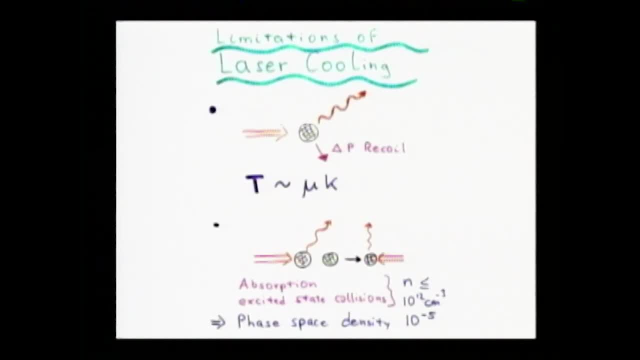 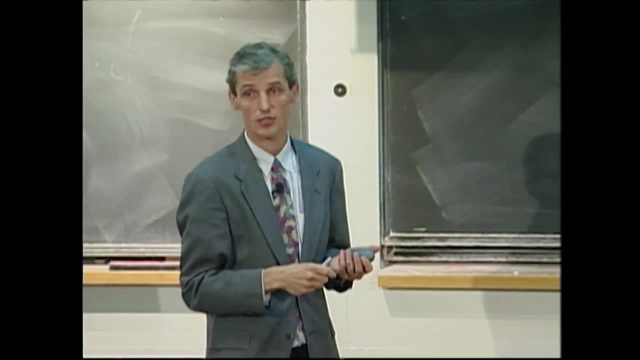 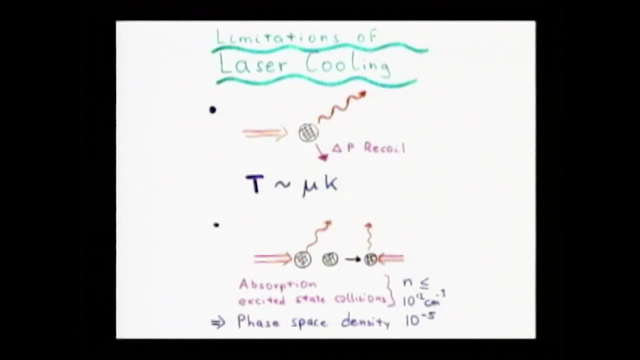 If you scatter light from atoms, each photon. the photons are grain heats like sort of scent corns which transfer a finite recoil momentum to the atoms. So therefore the temperature of the atoms and the temperature of the standard laser cooling methods is limited to micro-Kelvin. 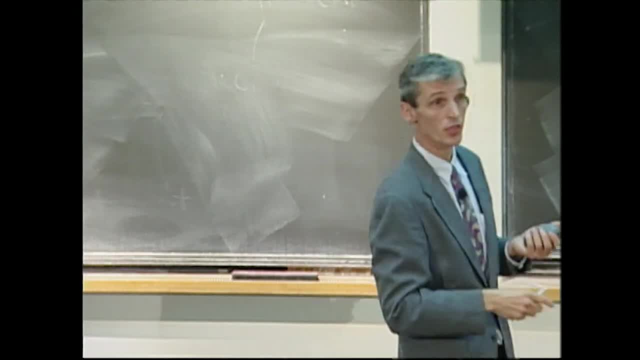 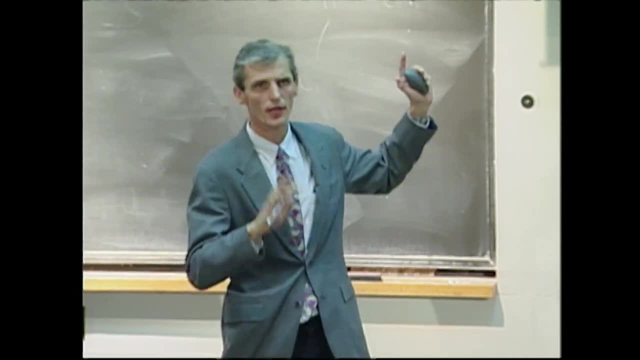 So well, if you can't get very cold, you should get very dense, because it's a density-temperature combination which makes Bose condensation happens. But unfortunately there's also a density limitation in laser cooling which, without going into details, 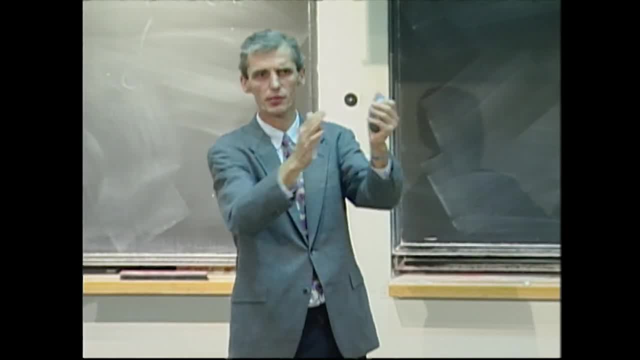 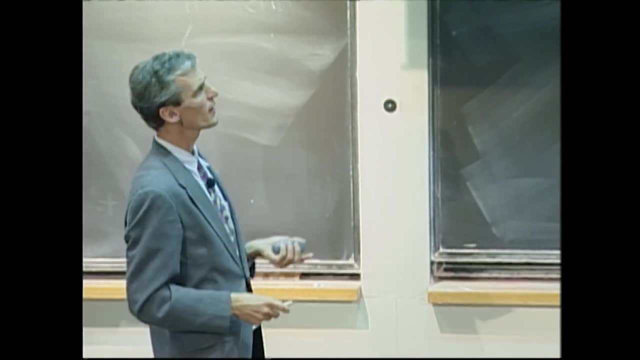 is simply set by the process. if you're a very dense sample, all the laser light is absorbed and laser cooling doesn't work. So laser cooling, at least in the beginning. in the beginning of the 90s fell short by four orders of magnitude in density. 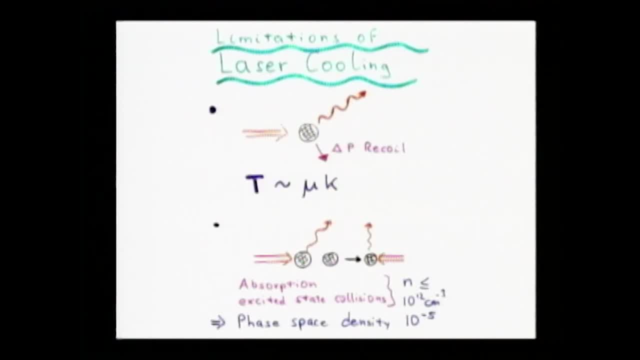 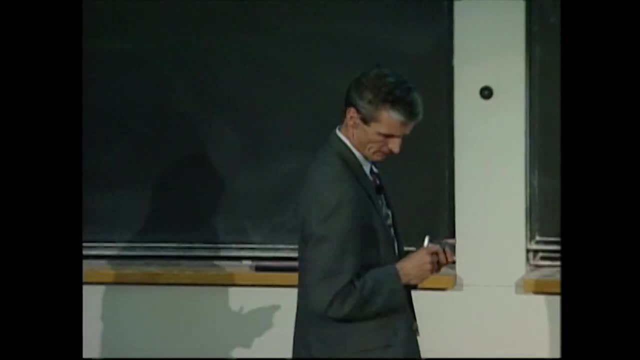 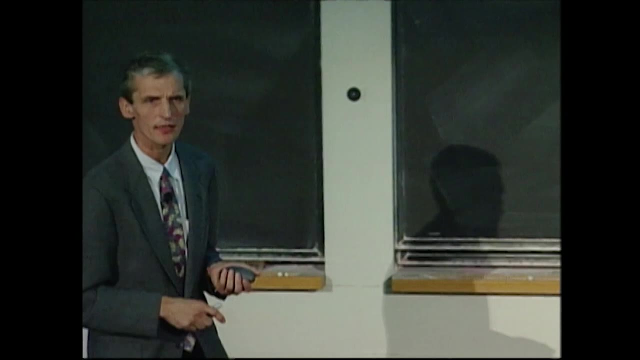 or three orders of magnitude in temperature to reach Bose-Einstein condensation. So well, this is something which Dave Pritchard developed, and I was a postdoc with him. But next door is Dan Kleppner who, together with Tom Greytek, 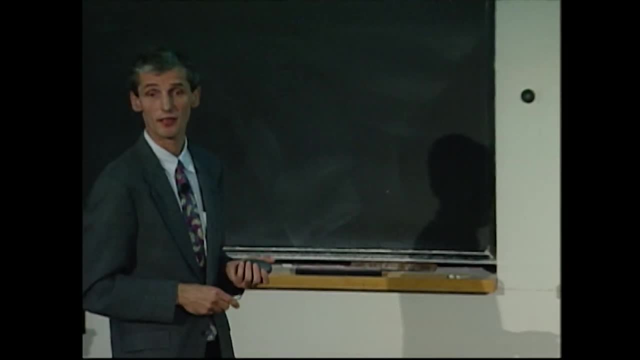 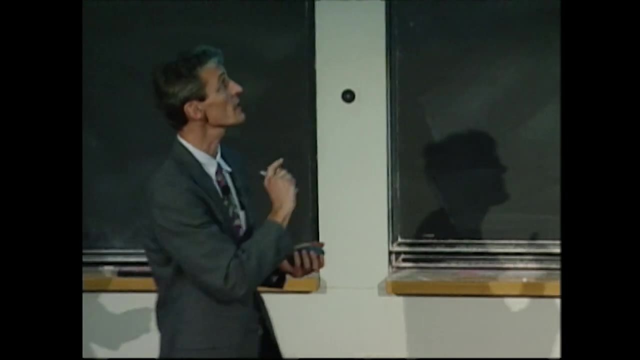 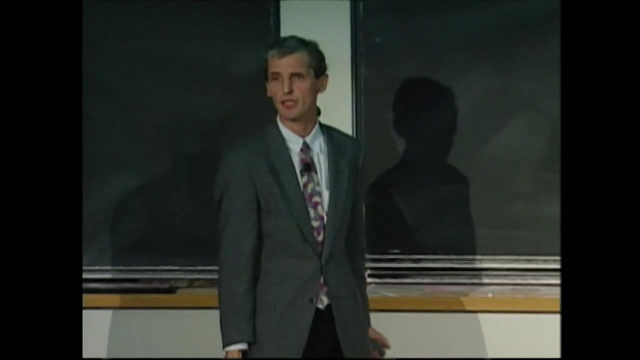 and Harold Hess developed evaporative cooling, And this is a different cooling method which is not suffering from all the limitations of laser cooling. So let me explain what evaporative cooling is Actually before I explain the slide. evaporative cooling is what happens in every day's life. 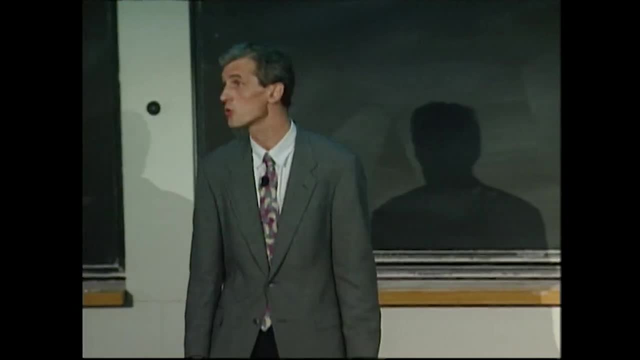 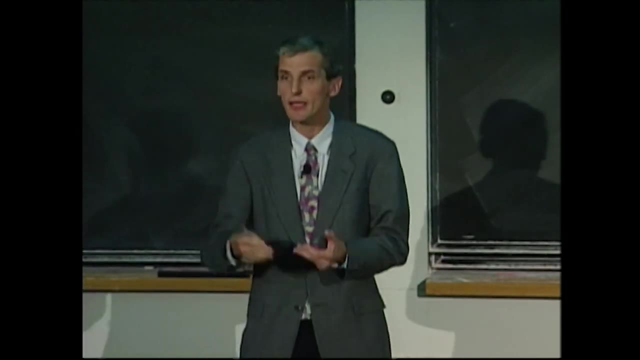 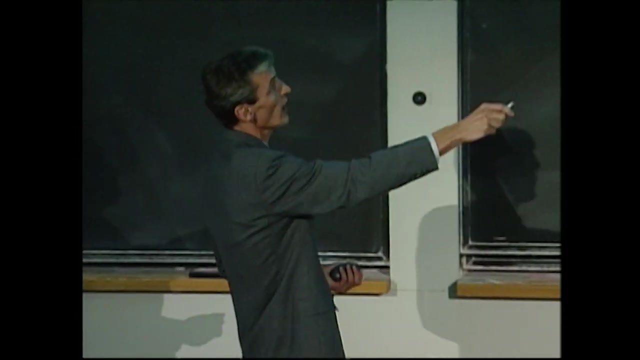 If you sit in a bathtub, the water cools down. And it cools down because the hottest particles escape as steam and what remains behind are the less energetic particles. This is called evaporation. So well, if we do it in an atom trap, if we confine atoms, 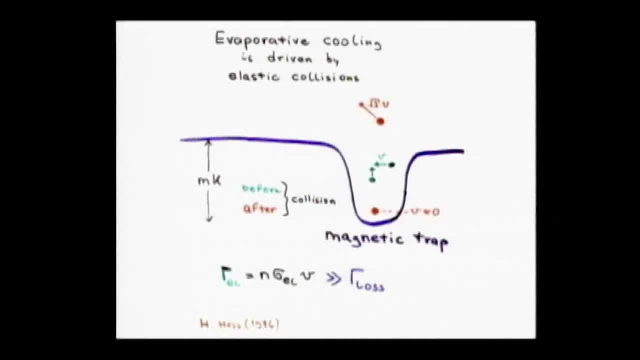 with magnetic forces, we create such a potential. It's like an invisible container, the walls of which are magnetic fields. I don't want to say more about it right now, But so you have particles in this container, And if two such particles collide? 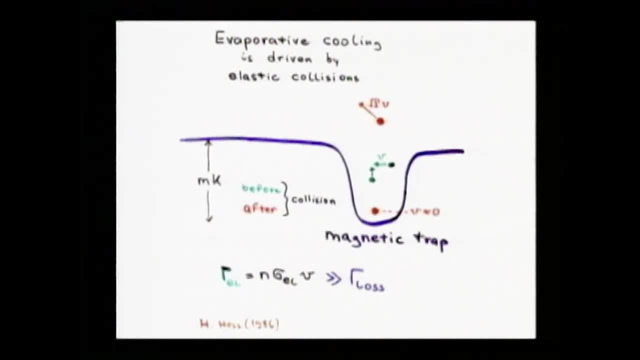 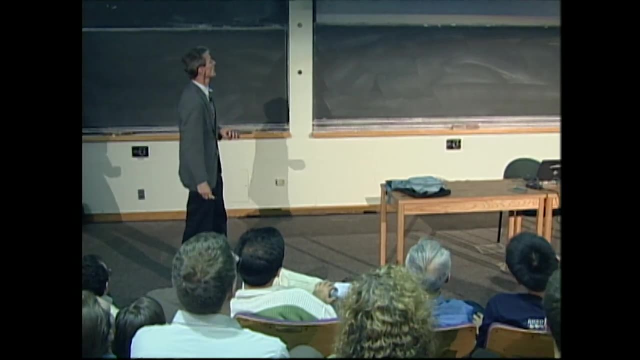 one can lower its energy, come to rest. These are the particles you want to keep. They're really cold And the more energetic one can escape. And this was suggested by Harold Hess and realized in the group of Ben Kleppner and Tom Krathek. 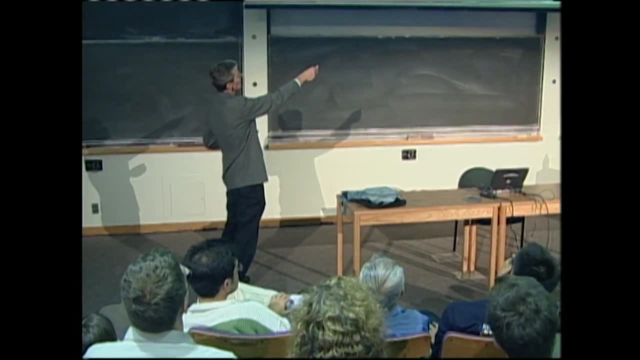 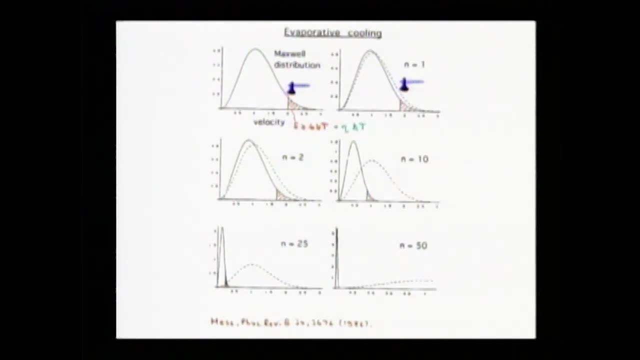 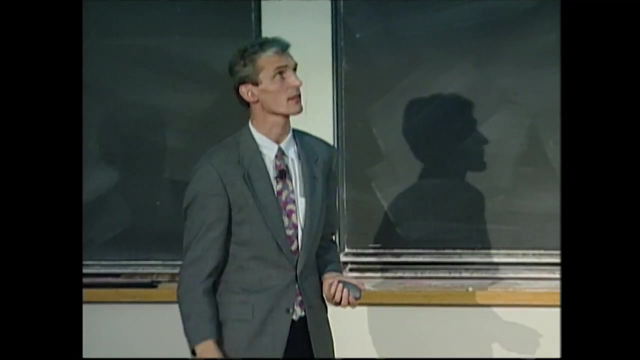 So if you have a method to kind of eliminate the hottest particles in many, many steps and the remaining particles re-thermalize, we create a thermal distribution which gets colder and colder and colder. So the question is how to implement it, And Dave Pritchard had a brilliant idea. 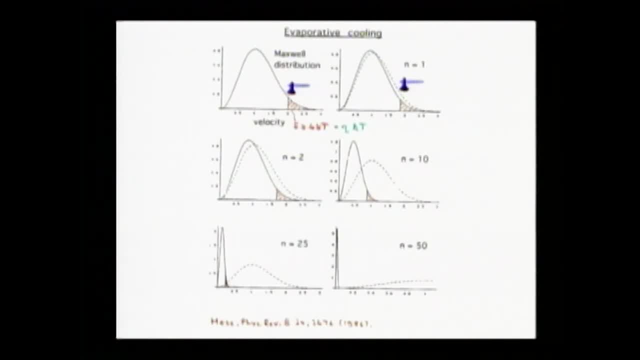 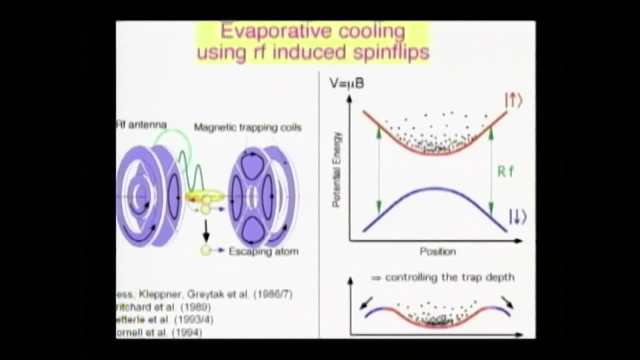 this sort of X which, so well, It's even dripping with blood here. What is a suitable X for atoms? So well, if you're in a magnetic trap, there's a very simple X, And this is just switch the magnetic moment of the atoms. 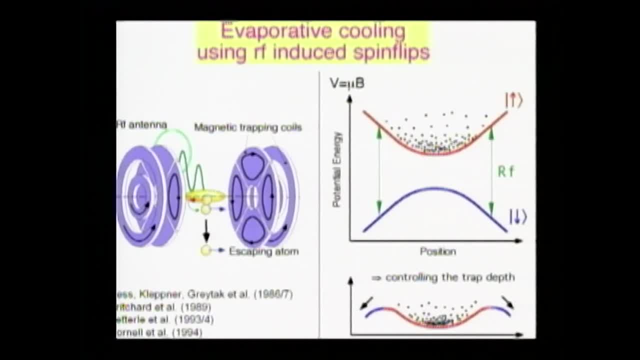 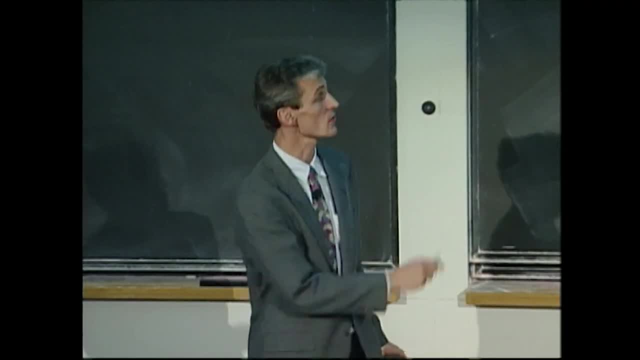 so that the attractive force, the confinement force, turns into a repulsive one. You just have to shine radio frequency onto the atoms And you have your X And you can do the cooling. So this was Dave Pritchard's suggestion in 89.. 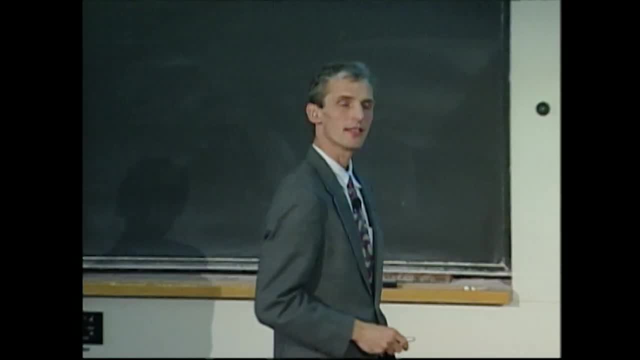 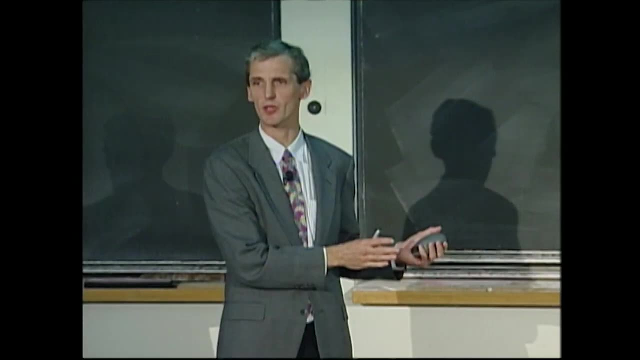 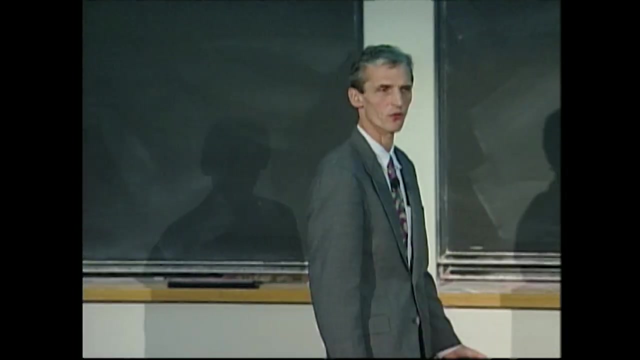 So well, here are two cooling methods developed by the people who had their office next to me: laser cooling and evaporative cooling. Laser cooling works great initially, has certain limitations, But evaporative cooling does not suffer from them, So it probably doesn't require rocket scientists to realize. 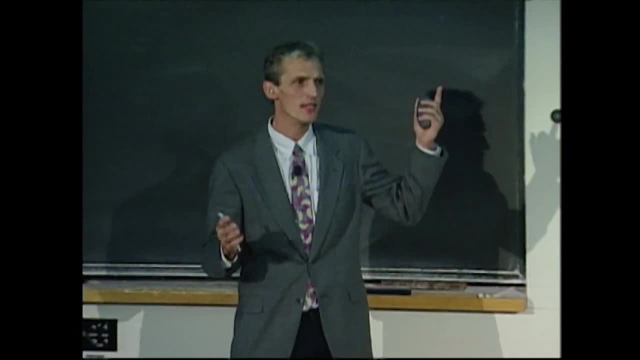 It would be a good idea to combine the best of two worlds. So this was sort of the idea in the early 90s. But there was a problem which, again, I'm going to talk about. Some people regard it as fundamental. 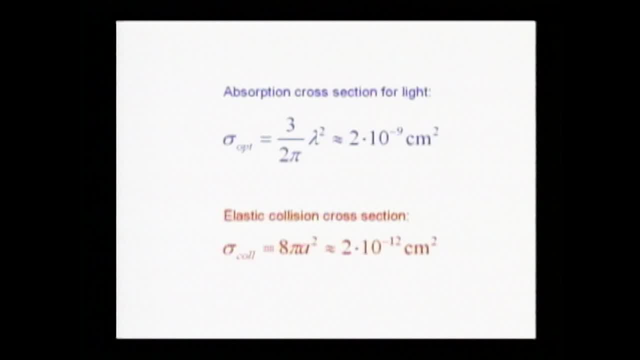 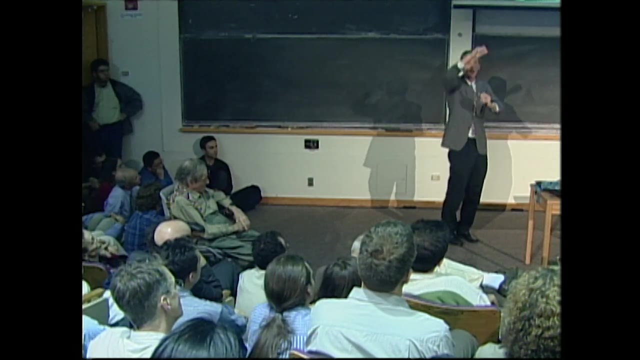 And the problem is that I mentioned that laser cooling doesn't work when the sample becomes opaque, when the light gets absorbed. On the other hand, evaporative cooling requires collisions between particles. One particle gets colder and one particle gets hotter. And now, if you look at the collision cross-section, 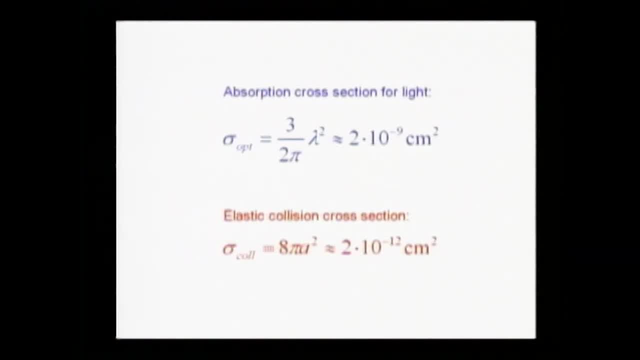 you face a dilemma. We don't want light to be absorbed, but we want collisions to happen, And the difference, the ratio of those collision cross-sections, is a factor of 1,000. So it seemed absolutely impossible to have many collisions for evaporative cooling. 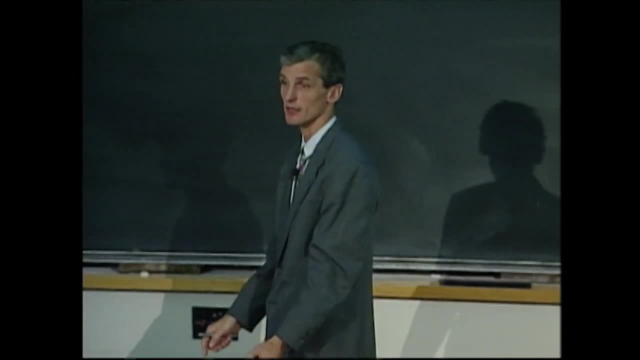 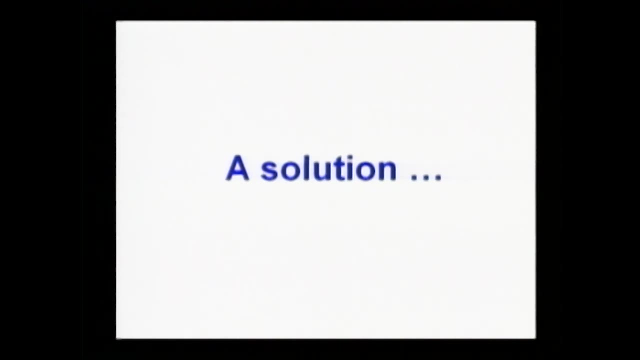 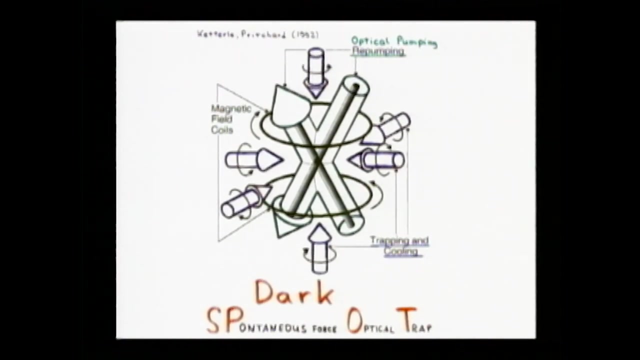 and at the same time avoid the complete absorption of laser light, A solution which Dave Pritchard, developed together with me, was so well. we can modify, We can push optical cooling to higher densities by just playing a simple trick. 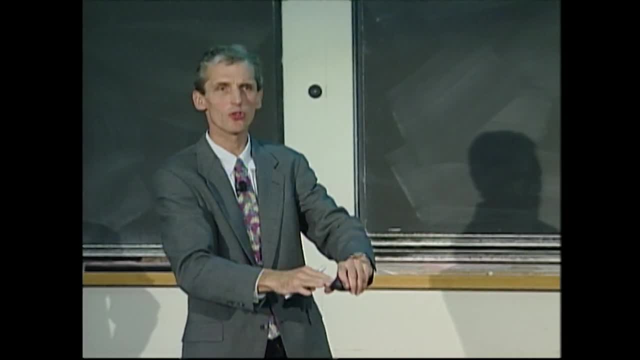 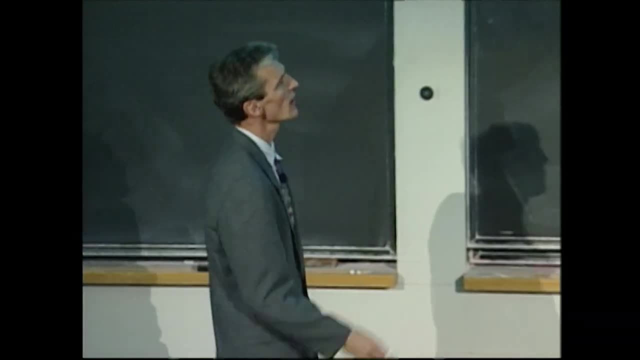 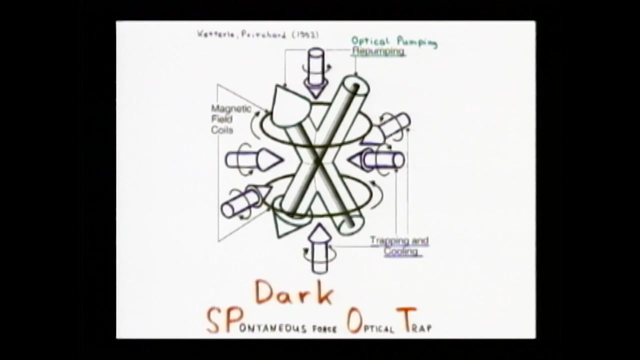 If we hide the cold atoms in a different quantum state so that the light is not absorbed, we can push laser cooling to higher densities. I don't want to go into details, but by modifying the standard mod, which Dave co-invented, we realized something. 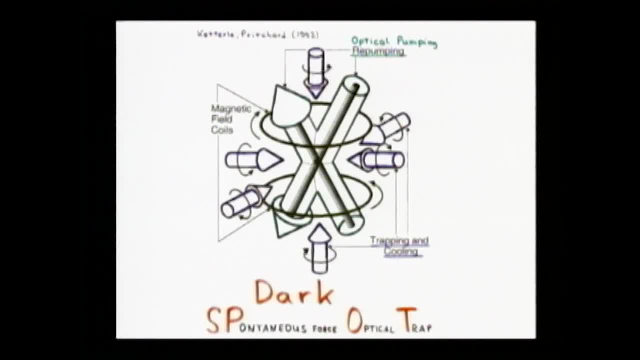 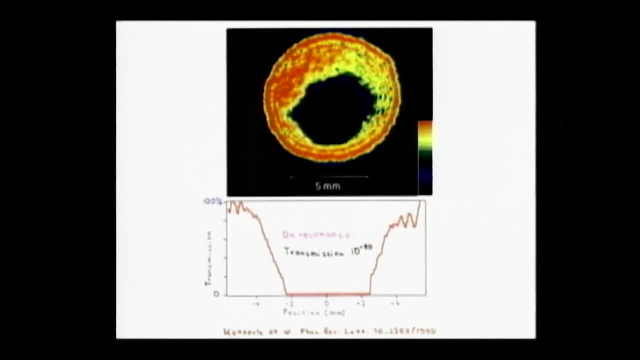 which is called the dark spot, And it was a key technique to achieve Bose condensation, both at MIT and at Boulder, And I just show you the result which at that point in 90,, two published in 93, was fairly impressive. 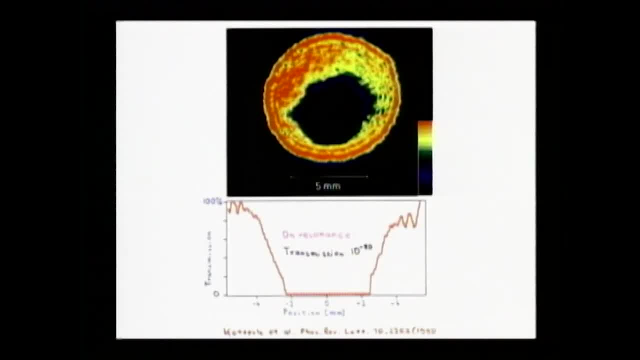 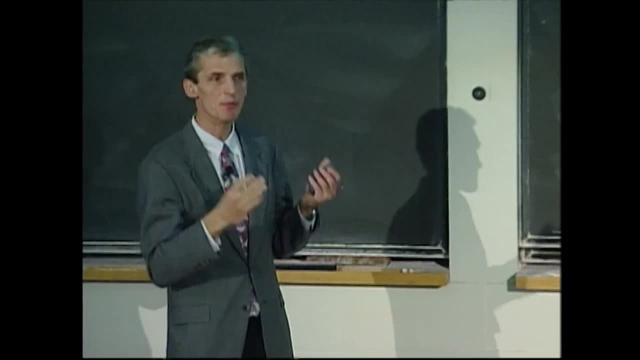 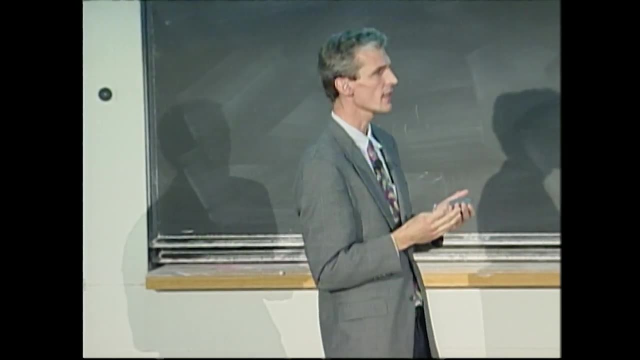 We were shining light at a cloud of atoms, and the shadow was really black. We could infer that the transmitted light was 10 to the minus 80. This was absolutely black, And so, in 92,, what we had in our hands was an unprecedented combination of high density. 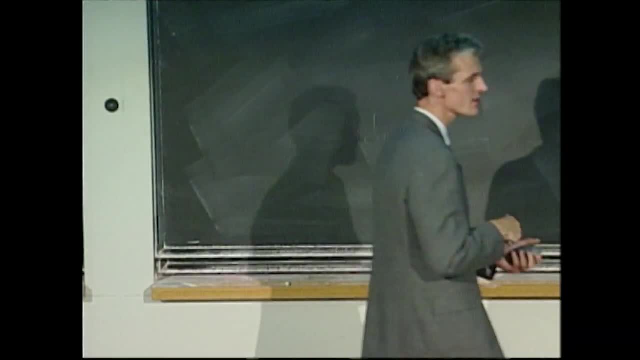 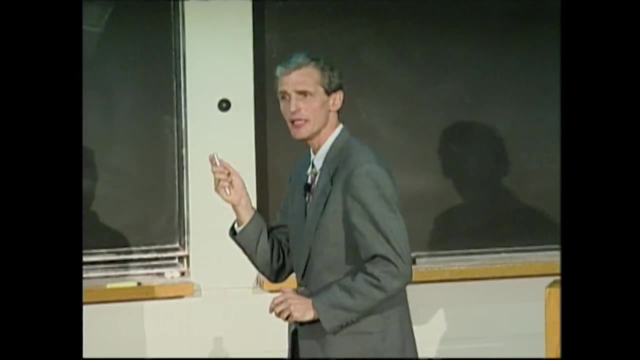 and large number of atoms. And then you told stories about me, Dave. now I have to tell a story about you, namely, I still- I mean, I remember those dramatic days. This was the summer of 92, and Dave Pritchard. 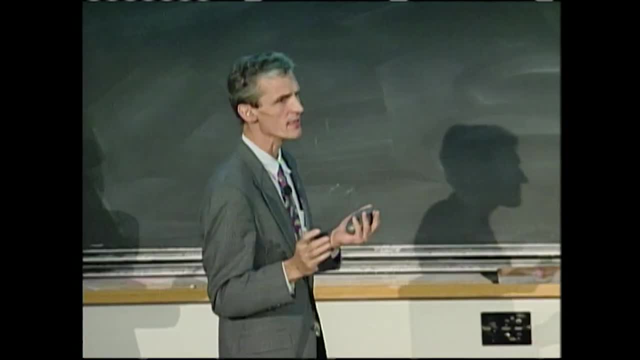 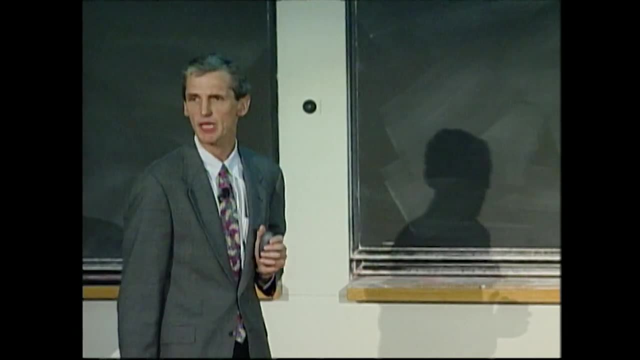 he had funded work, funded proposals, and he had great ideas to study cold collisions, to study cold molecule formation And eventually many people got a lot of credit for that, But we had. so this was the agenda and this was the proposed work and this 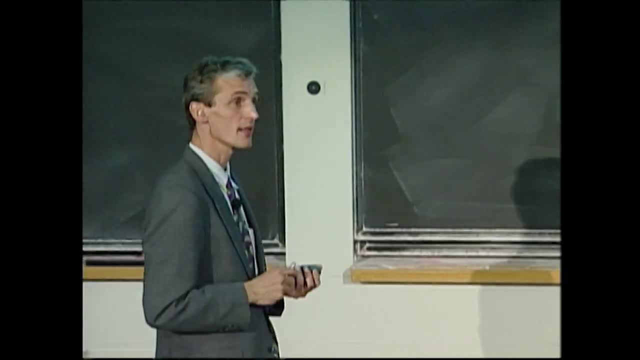 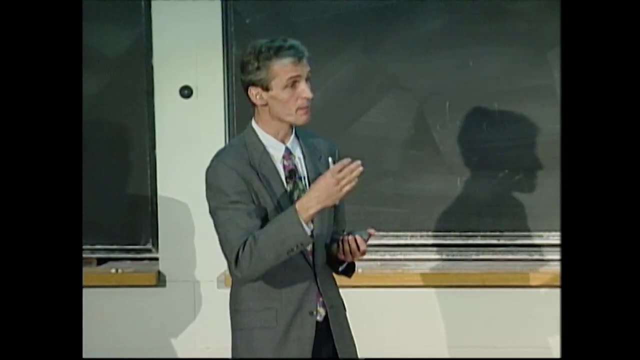 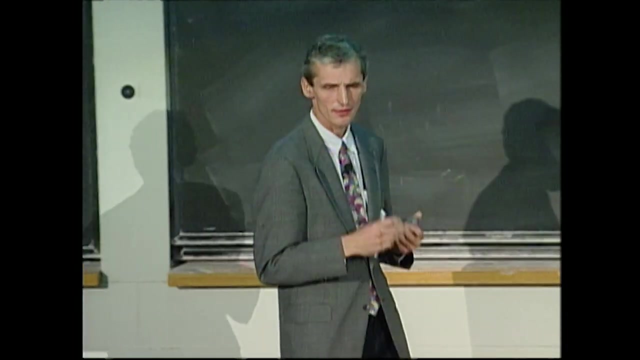 is what the funding agencies had supported. But then we sat together and decided maybe we can do something else with those high density sample, Maybe we can go for the very speculative and challenging goal of Bose-Einstein condensation. And it was for me just the signature of a great scientist. 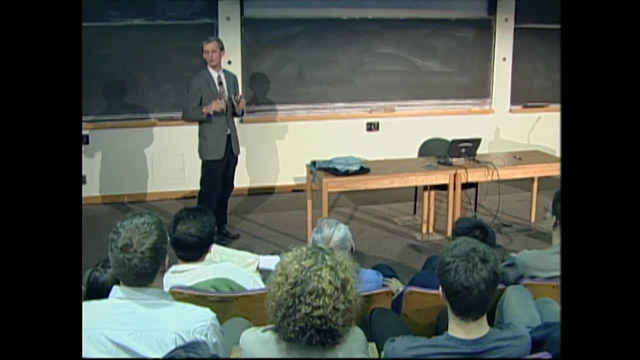 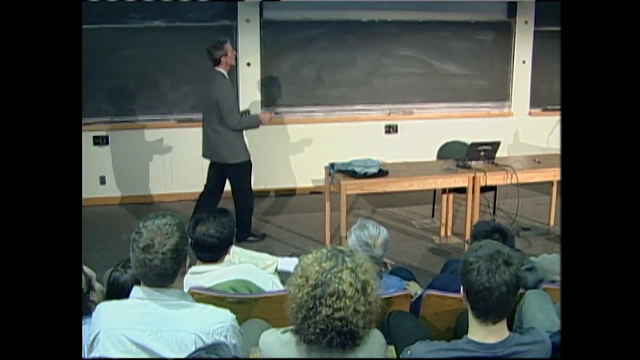 that Dave said: OK, I give up all my ideas, which were really great and which other people got enormous credit for that. Let's do what you suggest. Let's go for the long haul. Let's try to go further and use this as a starting point. 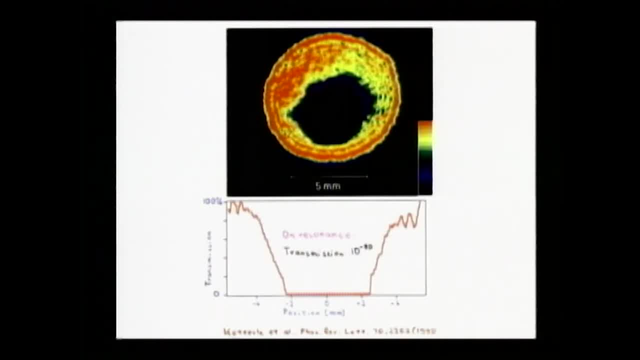 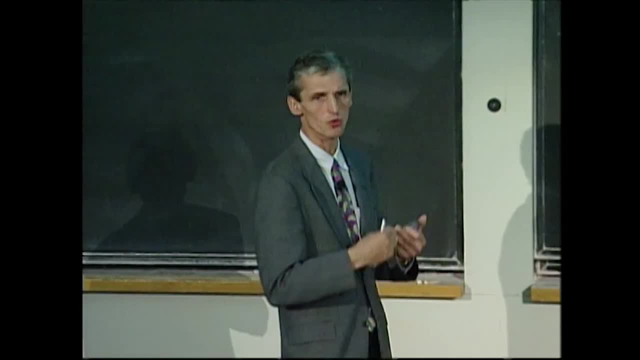 for the quest for Bose-Einstein condensation, And it was very dramatic. Within a few weeks, even before publishing the paper, we placed all the orders for additional equipment necessary to do the next step, to combine laser cooling with evaporative cooling. 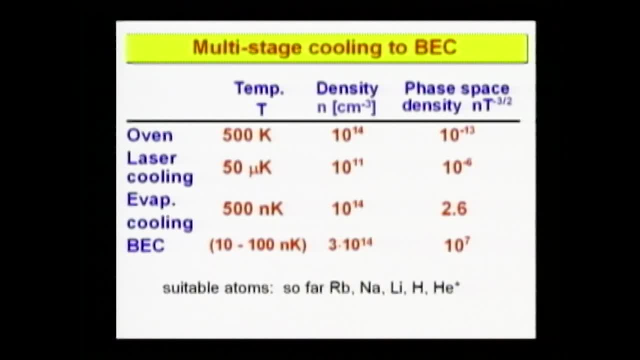 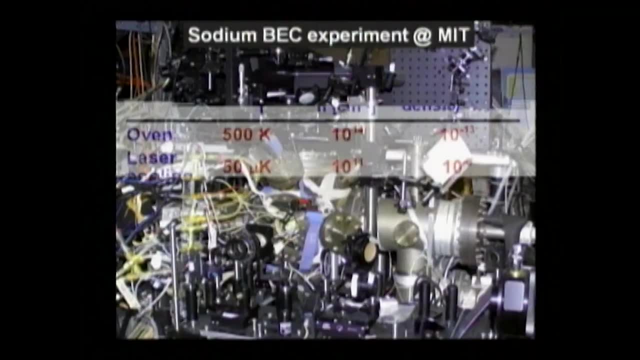 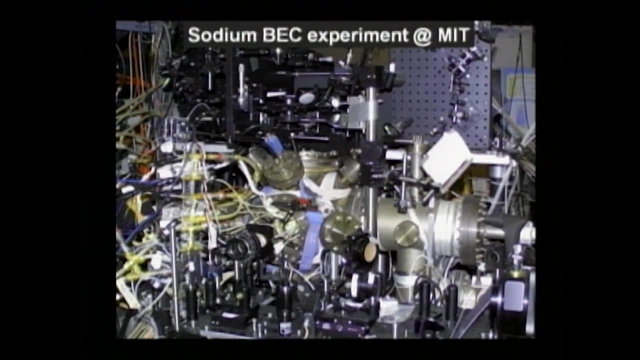 So eventually we wanted to embark on the agenda to use laser cooling as the first step and then lower the temperature by evaporative cooling and get to Bose-Einstein condensation. So well, We had to build a complete machinery for that And it took one or two years to assemble it. 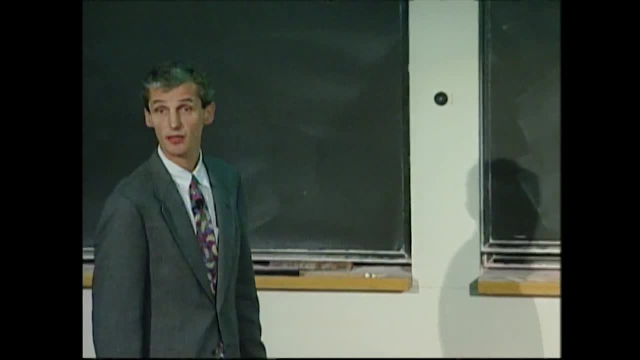 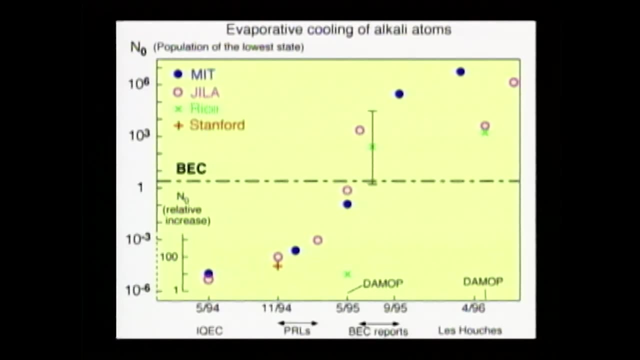 And then we were sort of ready and tried to see evaporative cooling And this- actually May of 94, was an important step. I went to a meeting and announced for the first time that laser cooling and evaporative cooling had been combined. 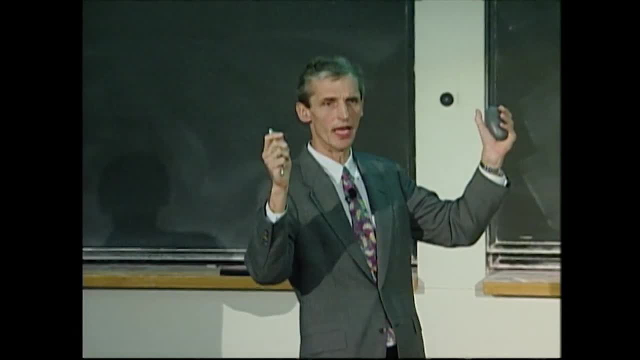 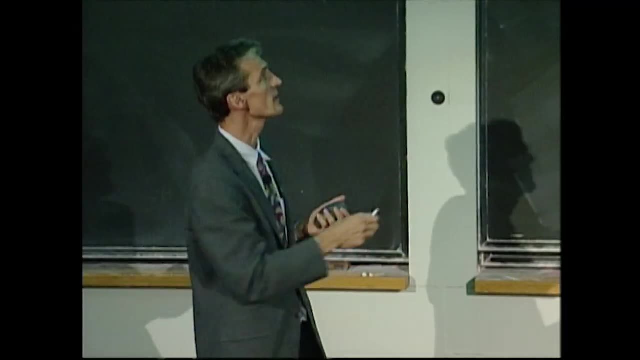 By using this high-density sample of atoms, we could bridge the gap between this factor of 1,000 difference in cross-section of light absorption, elastic collision. We had seen evaporative cooling And now we were hoping to push further to lower temperature. 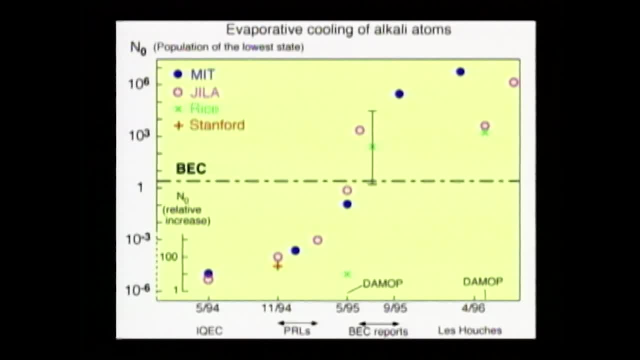 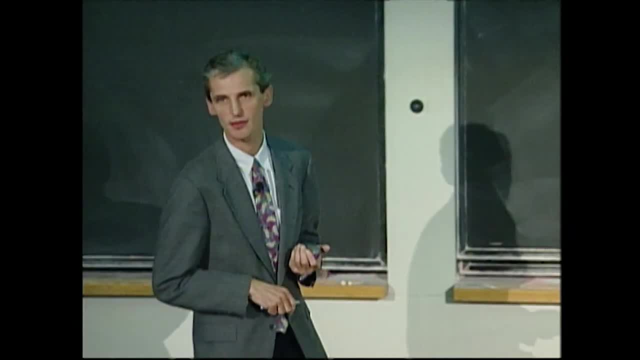 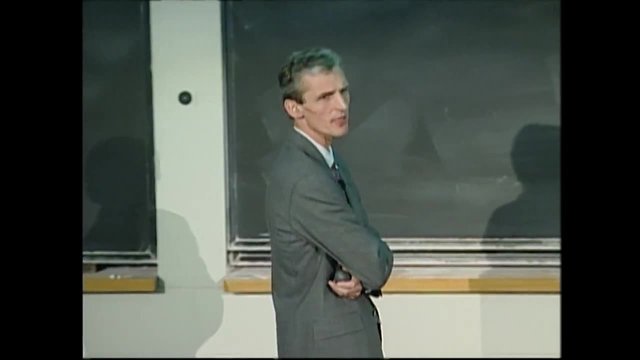 But still we were five orders of magnitude away from BEC. At the same meeting, the Boulder group announced that they had accomplished something similar, So the race went on, And it was one of the most exciting races of my lifetime, And Eric Cornell, Carl Wyman and myself- we remained friends. 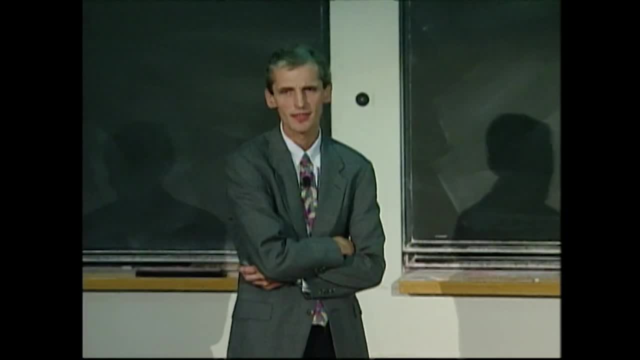 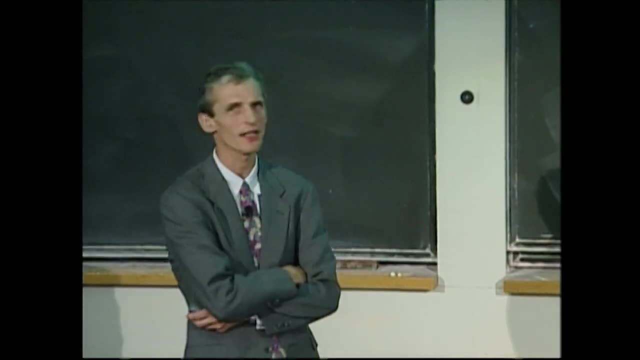 And we talked to each other on the phone on Tuesday And we both said to each other: you got the best out of me, Because if you have competition, you work harder, you think harder and you do better work. Actually, at that point I thought: 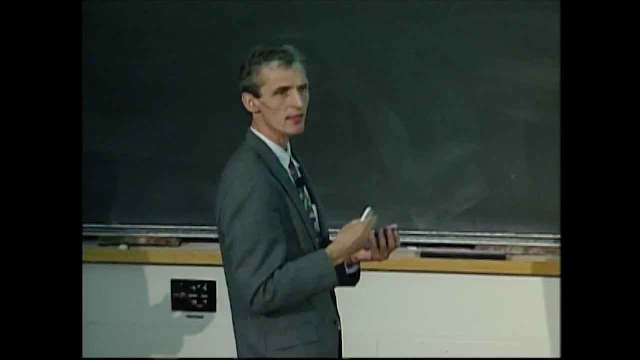 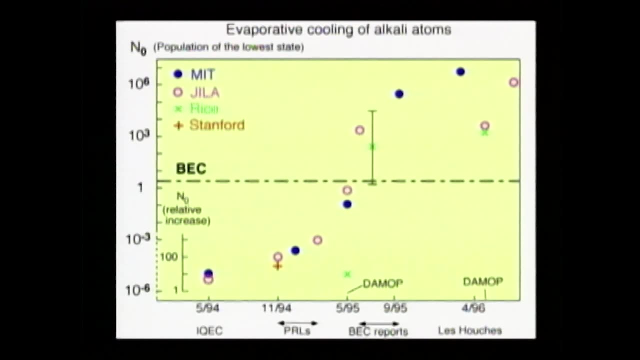 it could take the rest of my life to push further incrementally and explore the new physics which would come about at higher densities and lower temperatures, And I knew that the quest for Bose-Einstein condensation in Tom Greatex and in Kleppner's lab had already lasted. 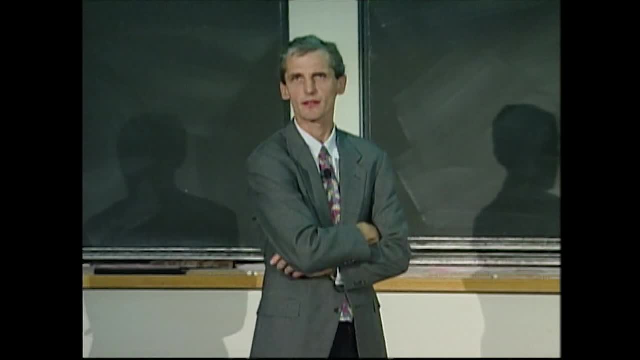 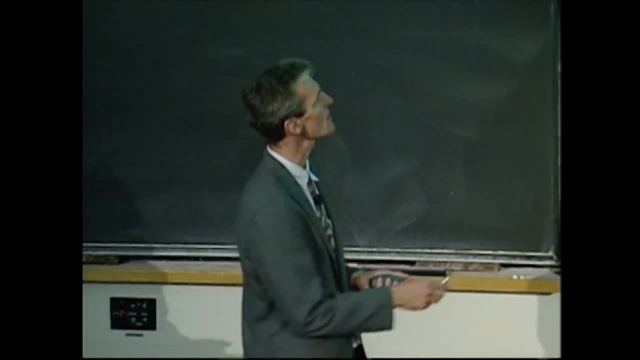 It lasted 15 years And I was expecting so well, we try now something alternative And let's see which method works better. And to the big, big surprise- and it came completely unexpected- just one year later, Bose-Einstein condensation. 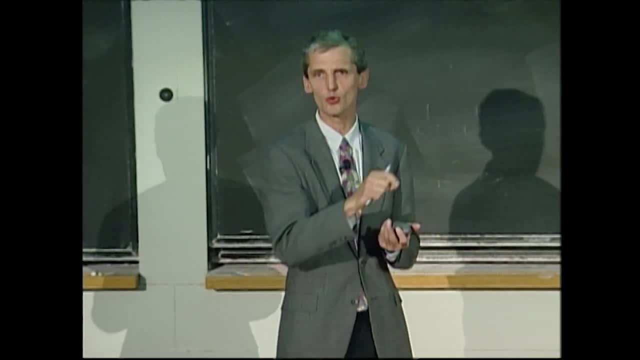 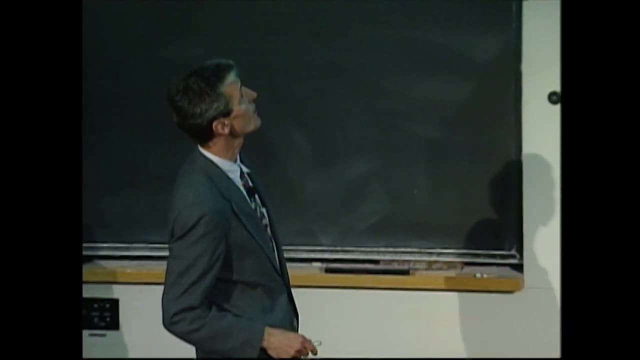 was achieved. It's one of the rare examples, I think, where you think you do an incremental step and you step forward by effect of a million. So these were very dramatic moments. Let me mention a little bit about the last obstacles on the finish line to Bose-Einstein condensation. 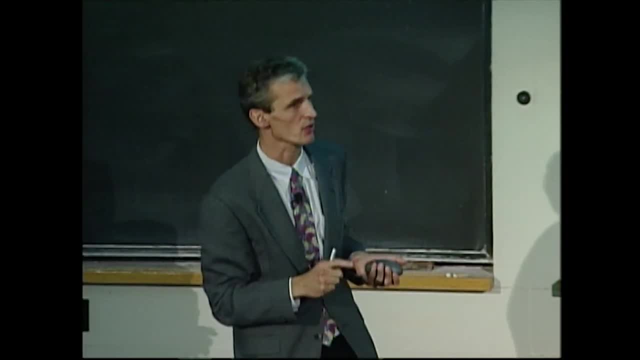 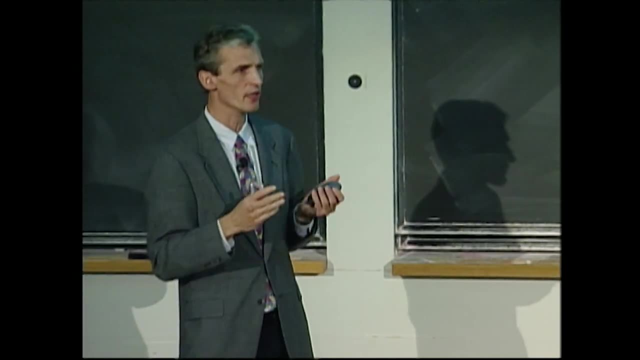 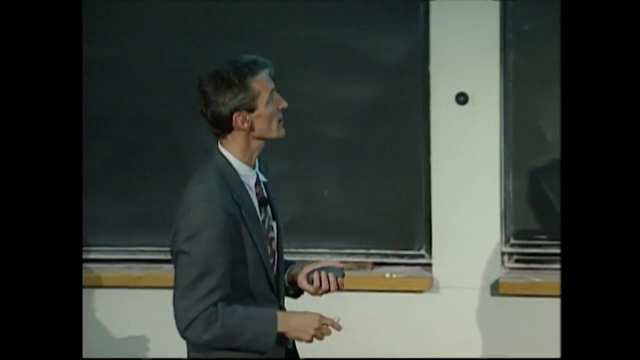 So the combination of evaporative cooling and laser cooling was accomplished. But in order to have enough collisions between the atoms to have good evaporation, we had to keep the gas tightly confined. So we needed tightly confining containers or magnetic traps. Now this may be a little bit technical. 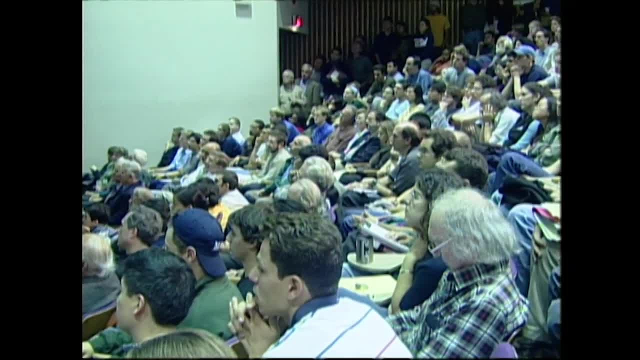 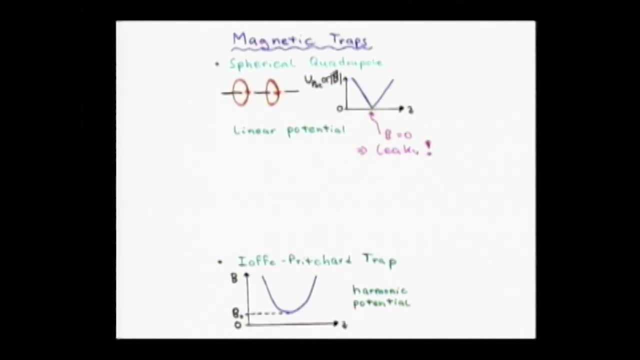 but some people are in the audience who probably are interested in that. There are two types of magnetic traps. Some have a pointy potential, a linear V-shaped potential, and others have a round potential. at the bottom. Those traps are more tightly confining. 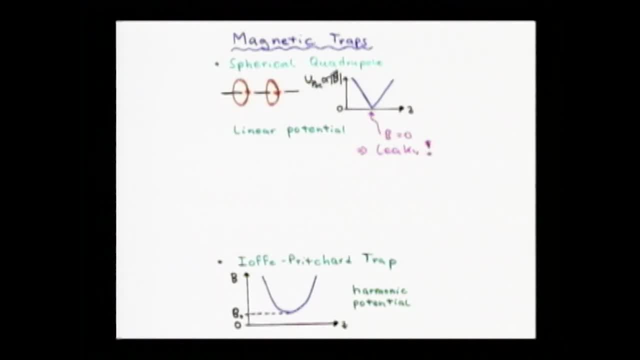 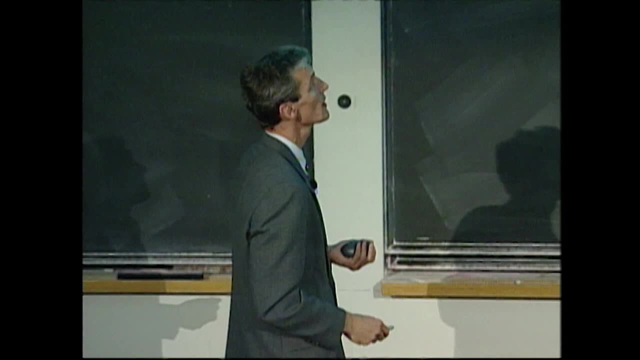 and that's what both the group in Boulder and at MIT used to demonstrate. initially evaporative cooling, because it makes it easier to get many collisions and see evaporation. But they have a problem: There's a point of zero magnetic field in the center. 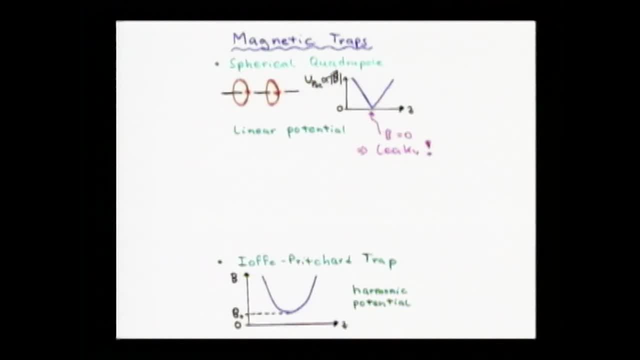 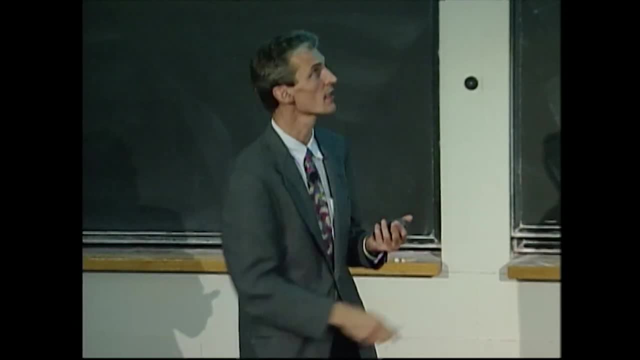 and if the field is zero, the atoms don't know what is spin up and spin down. They lose their orientation and virtually flip out of the trap. So we lost the atoms. It's like a hole where atoms leak out, And the months before BEC was achieved. 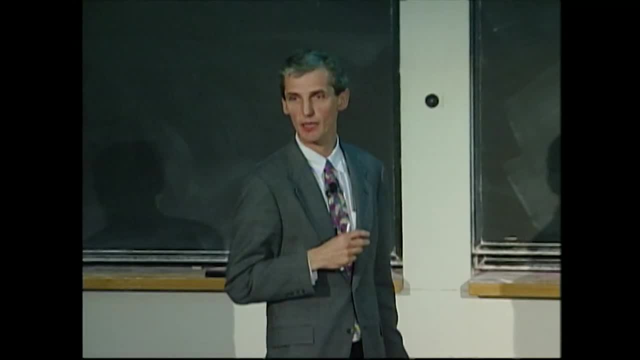 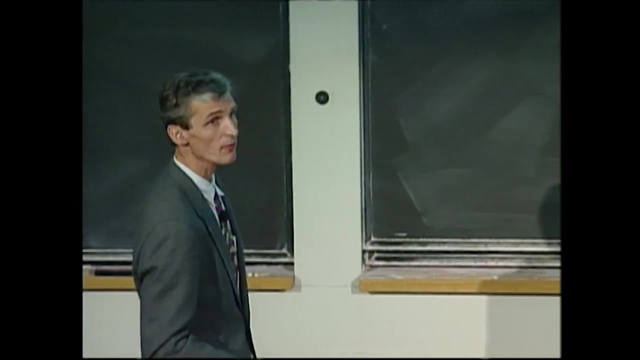 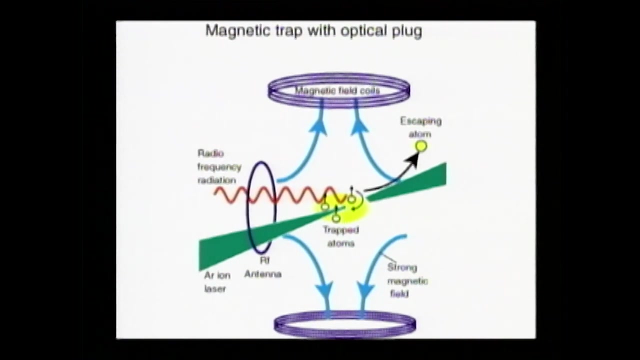 Bose groups had to invent methods- and this is how it was dubbed- how to plug the hole. Eric Cornell's group in Boulder used an ingenious method with rotating magnetic fields, and we decided To use a different method. we wanted to plug the hole with a laser beam, which 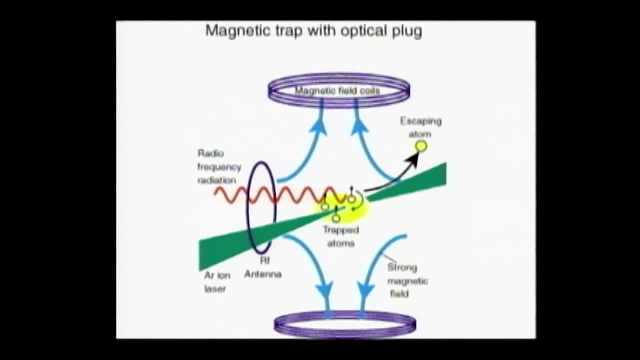 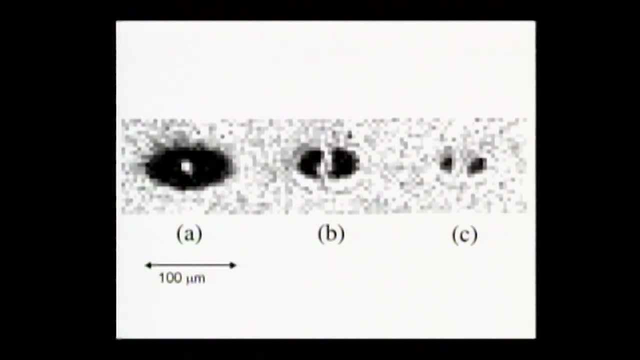 was keeping the atoms away from this dangerous region, where they would just fall out of the magnetic trap. So what we created was a potential which has a hole in the middle, And you see here the shape of our clouds, And it worked great. It was really dramatic. 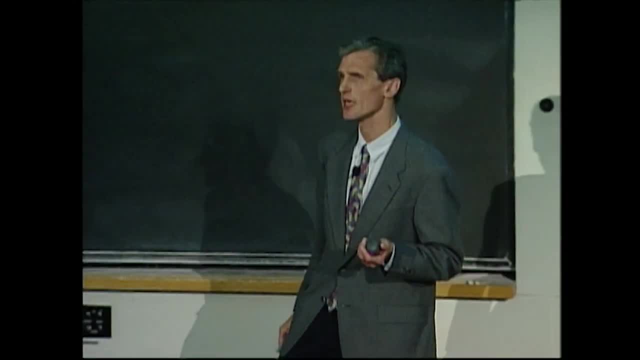 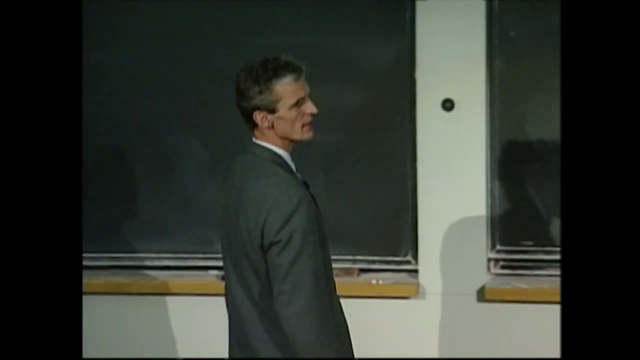 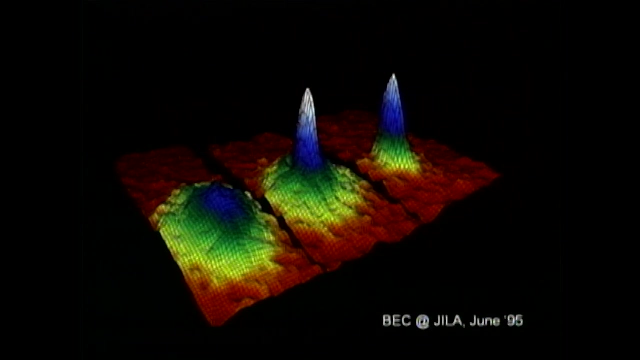 We could push forward orders of magnitude towards Bose-Einstein condensation. And then- this was in June of 95, we heard about the BOLDA results. They had succeeded to get Bose-Einstein condensation, And that's maybe something I don't know if I've shared it. 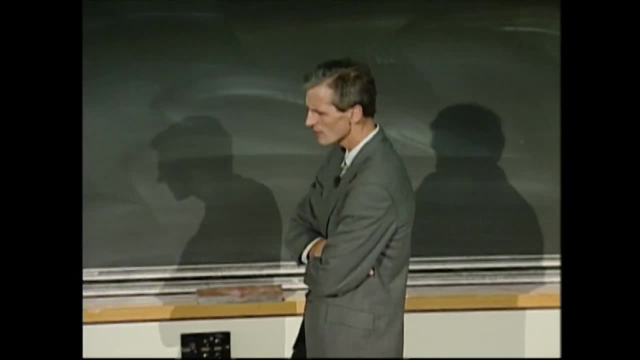 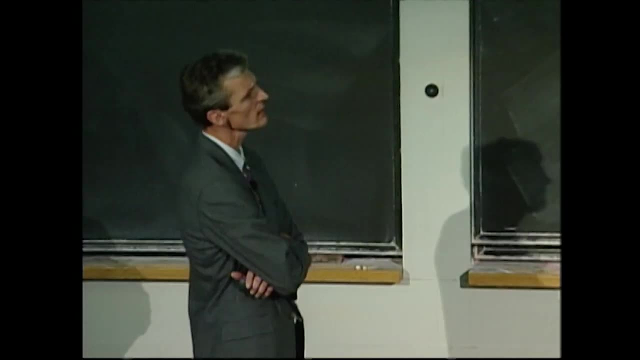 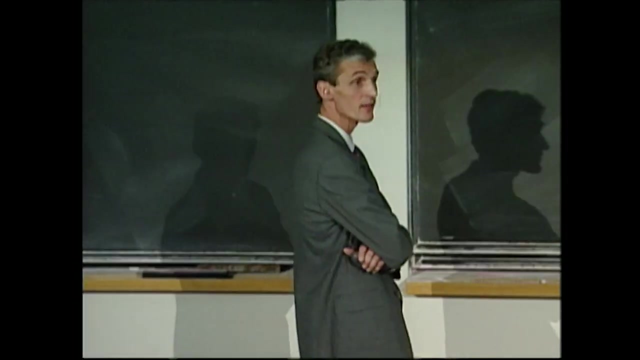 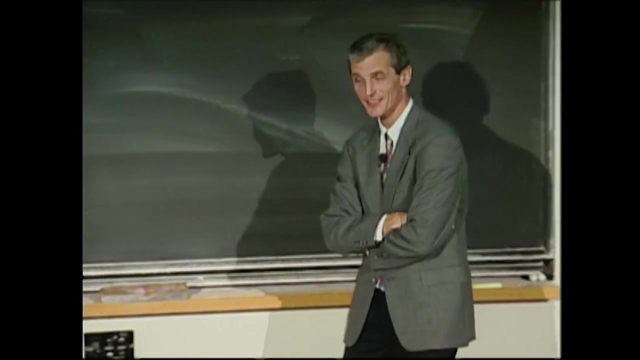 publicly. if you're an assistant professor, you put all your money, all your resources, all your efforts on one goal, and then you're notified that somebody else has accomplished this. This is a difficult situation. You wonder about promotion, You wonder about your scientific career. 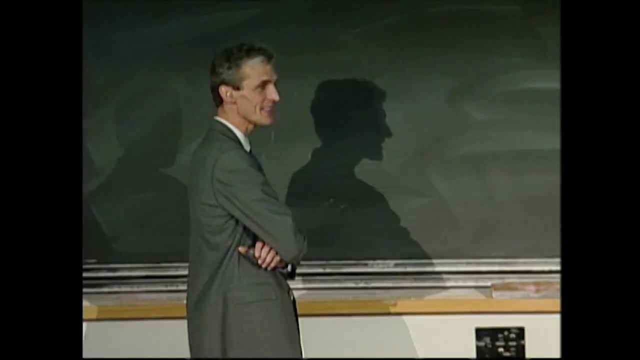 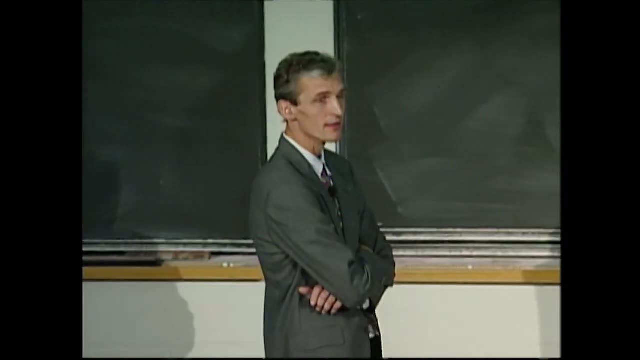 And of course I know at MIT the bar is very high. MIT is not keeping losers, So I was really scratching my head. I woke up early in the morning what to do And people asked me: why don't you just? 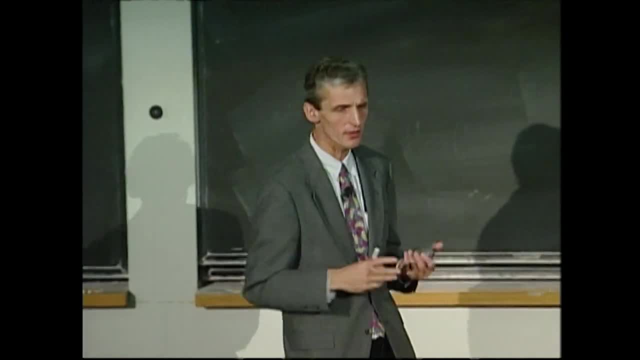 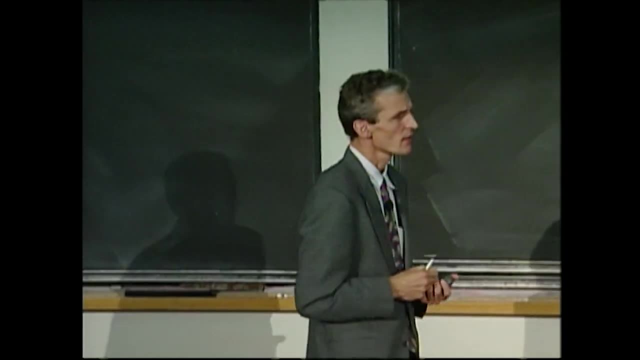 copy the design in BOLDA And I mean this seems to be a successful way to do it. And then a whole new field opens up And we had fierce discussion in my group And what we did, What we did, is actually a two-fold strategy. 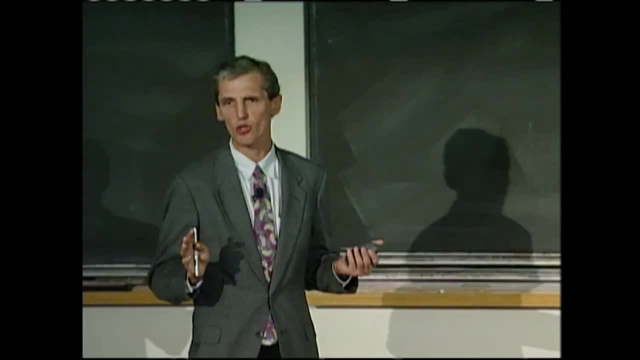 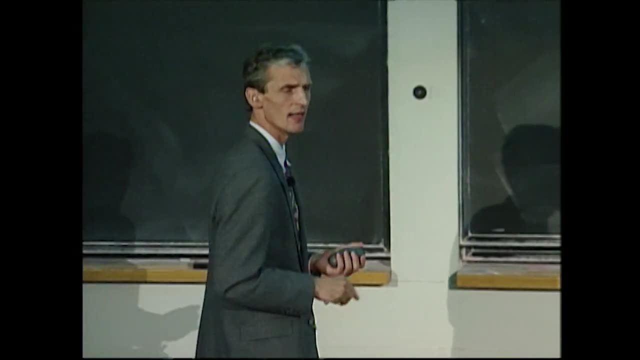 We designed a new magnetic trap- I will talk about it- And this turned into the workhorse of the field And this has given us an enormous productivity over the last few years And I was sort of willing to say: let's just put all our eggs into this basket. 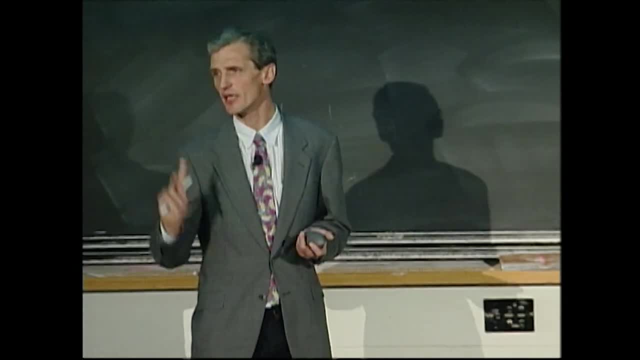 Let's pursue that, because this new magnetic trap is a really good idea And indeed it turned out to be a good idea. But I worked with a good group of people And they told me so well, this trap with the people. 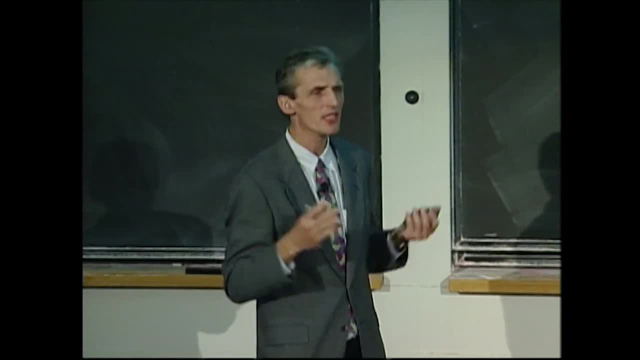 it's not going to work. It's not going to work, This trap with the plug. maybe it will work. Or even if it doesn't work, because maybe the laser beam is jittering and heating up the atoms, let's just give it one or two more tries. 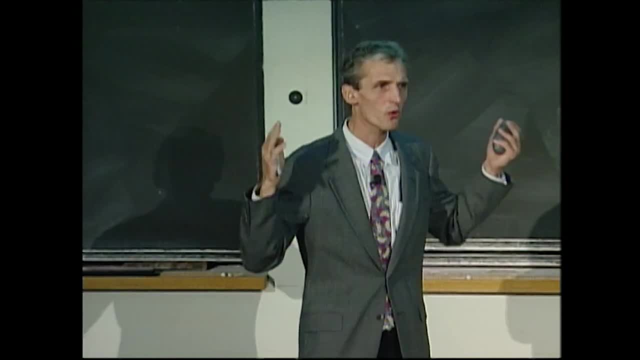 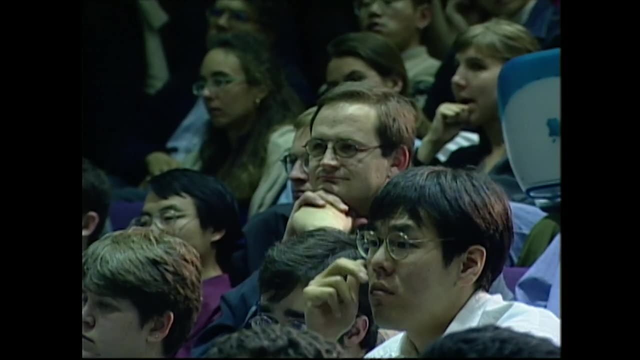 And let's just figure out how far we have come, because the BOLDA group has a big success And we should at least document how close we came. So well, I tried to listen to my collaborators and said, OK, but just a few times. 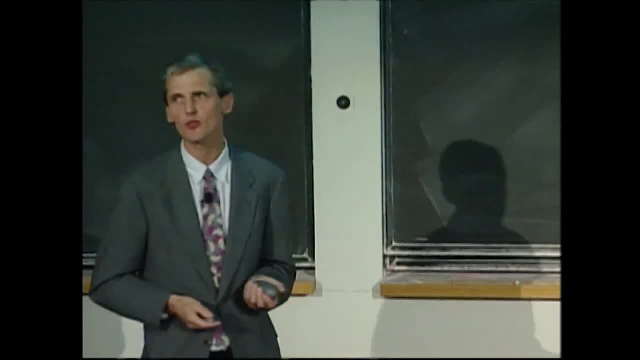 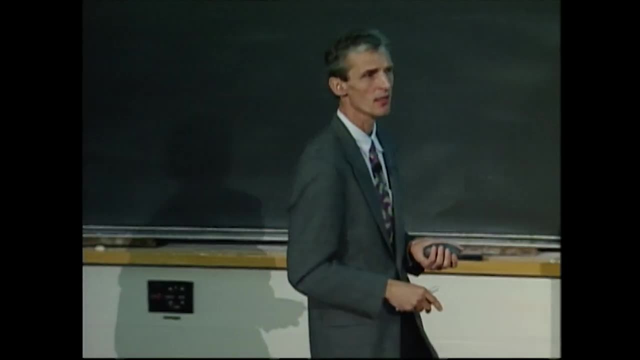 We can't waste time, We don't want to miss the boat, And it was one of the very last attempts to see how far we could push with our original idea of this optical plug trap that we saw Bose-Einstein condensation. This is a picture which doesn't look nice. 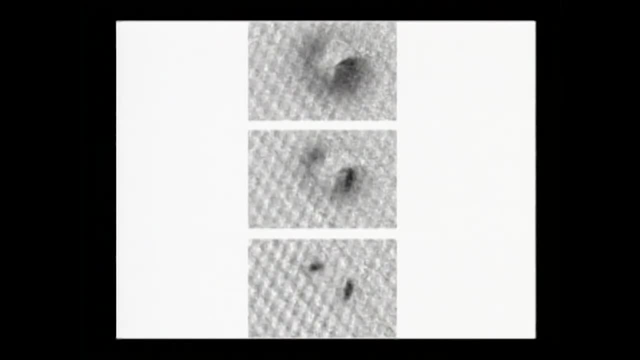 but I want to show it to sort of the experts. This was our first signal of Bose-Einstein condensation on September 30th in 95. We were not really ready to observe it. We just wanted to see where are the limits of the plug trap. 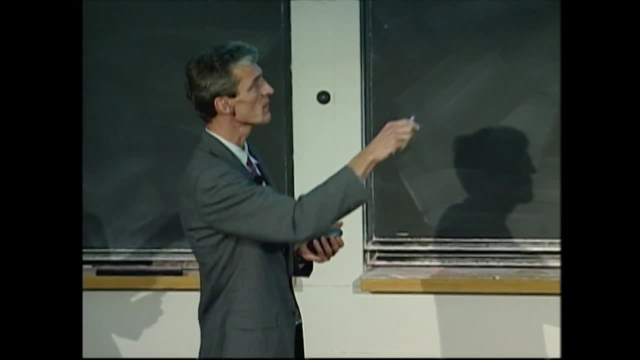 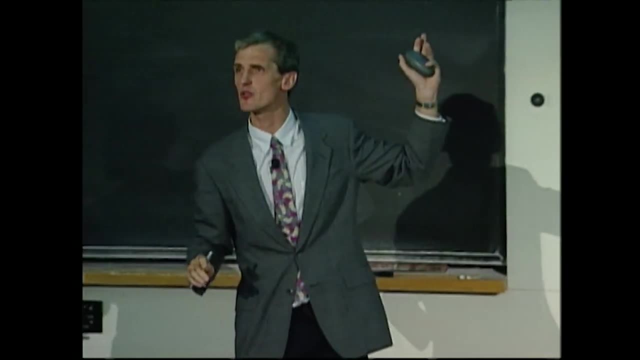 And for the experts, we couldn't switch off the laser beam, So in time of flight the atoms were just pushed away by the laser beam. So it's not a pretty time of flight picture. It doesn't look as pretty as the other ones. 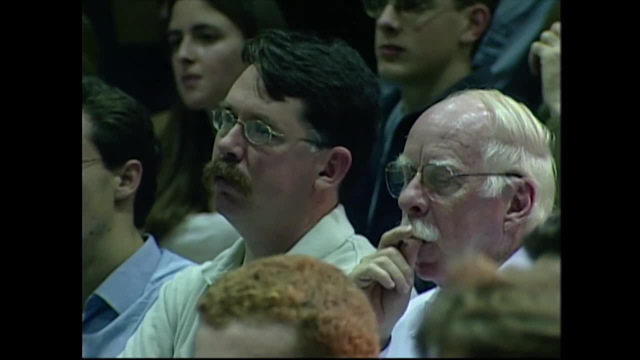 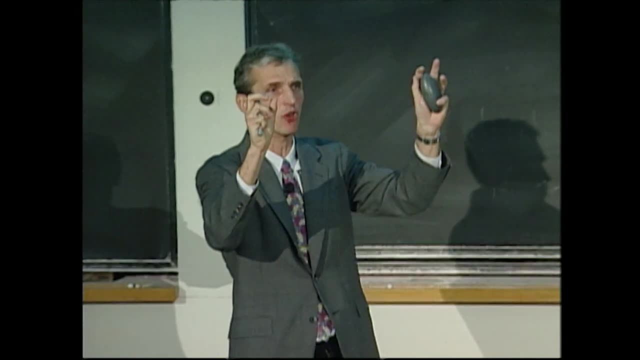 But we saw something black, sharp black spots on the screen, And if a cloud expands ballistically and stays compact, that means there's very little velocity, There's very little motion, It's very, very cold And we got enormously excited. 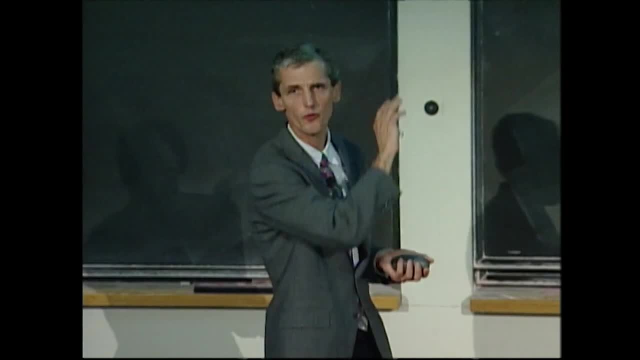 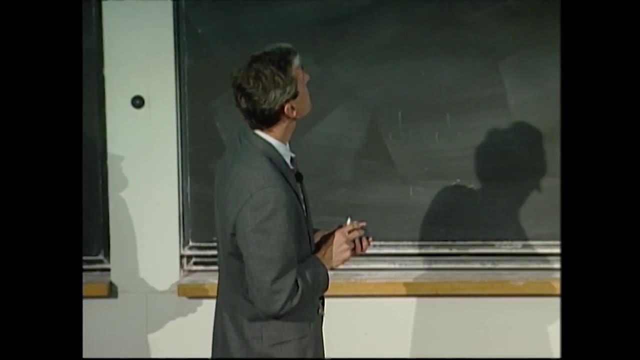 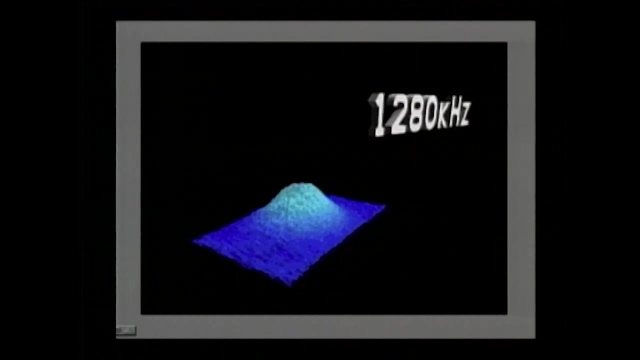 And within a few hours, we worked throughout the whole night, We improved the setup And we got clear evidence that we had observed Bose-Einstein condensation. We were running the experiment only one more time to get final data, And this is actually, for me, still amazing. 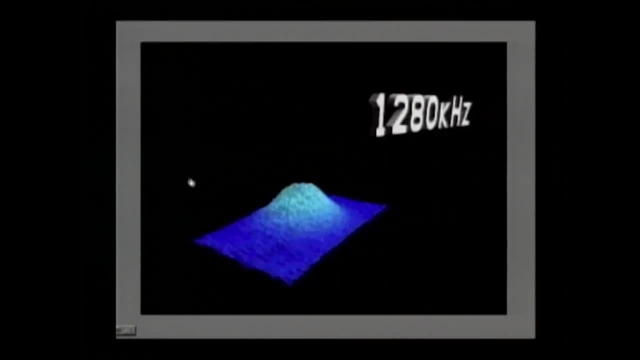 This is the quality of the data which was obtained the second time we were ever running the machine for Bose-Einstein condensation. Let me just explain what it means. We let the gas go and it expands out, And then we take a snapshot. 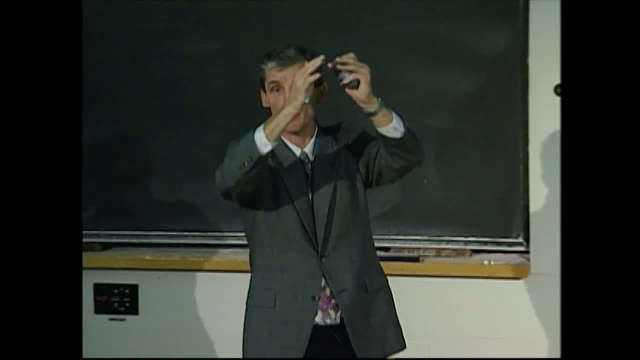 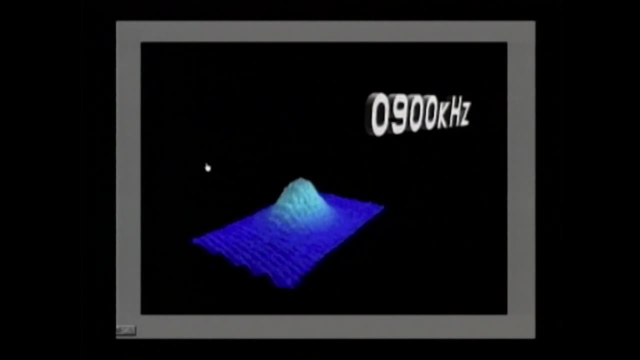 And the larger the cloud is, the faster is the velocity, the hotter are the atoms. And now you see what happens when we cool down. You see how this cloud is sort of shrinking because the atoms slow down. And this is sort of the last factor of two. 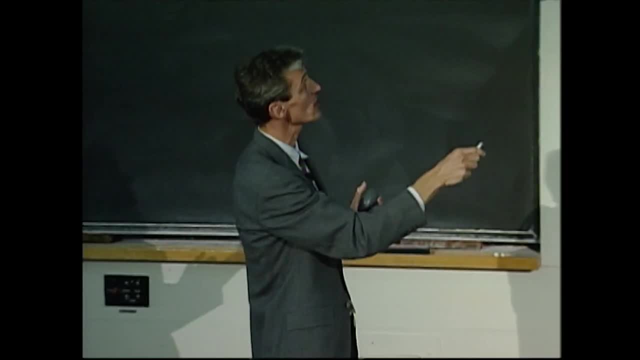 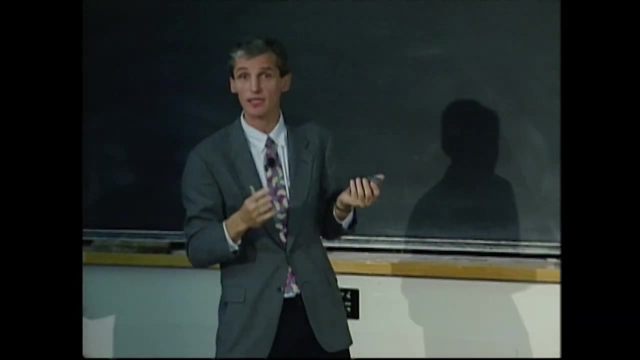 the last fraction of a second to achieve Bose-Einstein condensation. And then this new form of matter, this ultra-cold gas, which is the Bose-Einstein condensate forms. It's very visual, It's very dramatic, And we obtained that without really optimizing our machine. 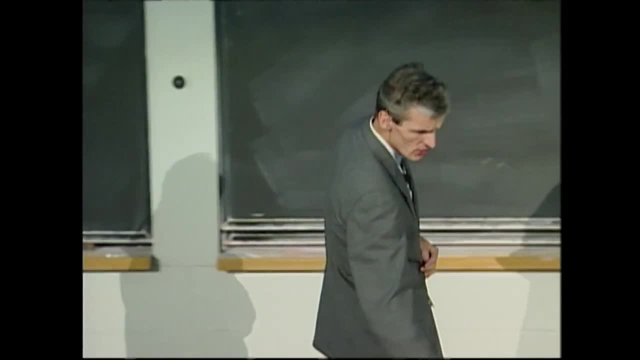 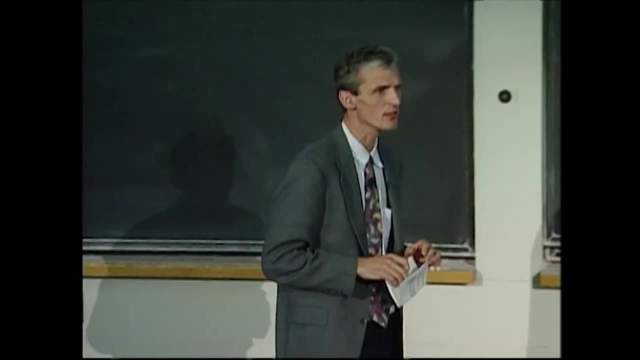 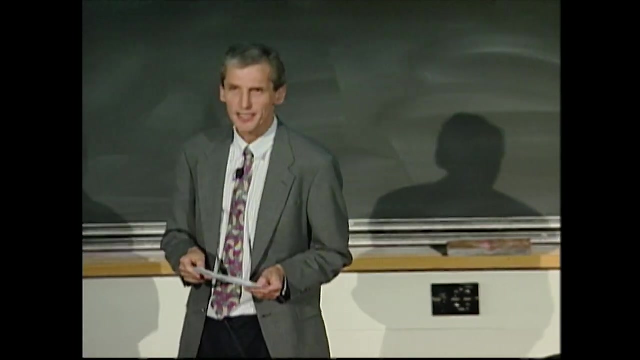 OK, So I mentioned that this was a night on September 30th And so well, at MIT you have to teach, And October 1st I had to teach 8012.. I received an email message from one of my students now. 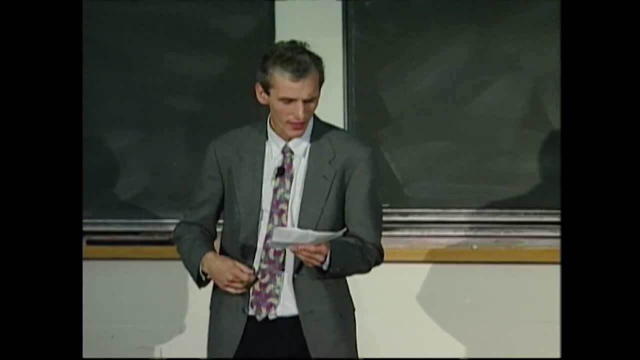 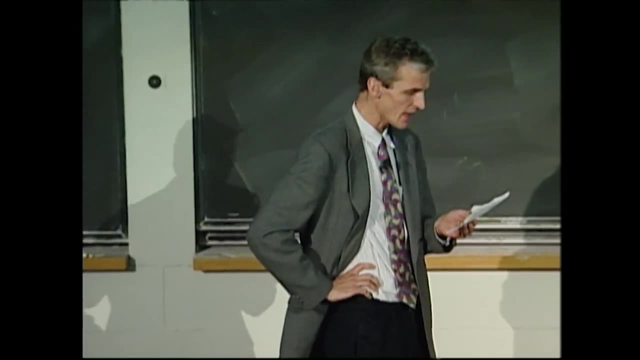 Six years later, as a freshman, in the fall of 95,, I took your 8012 class. I remember one day when you were unusually late for your lesson. You had a lecture And you came rushing in very excited, yet very tired. 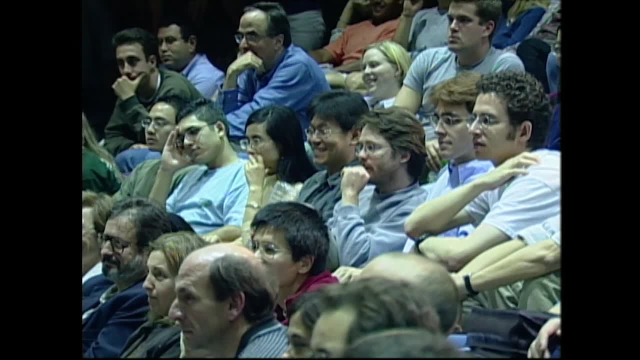 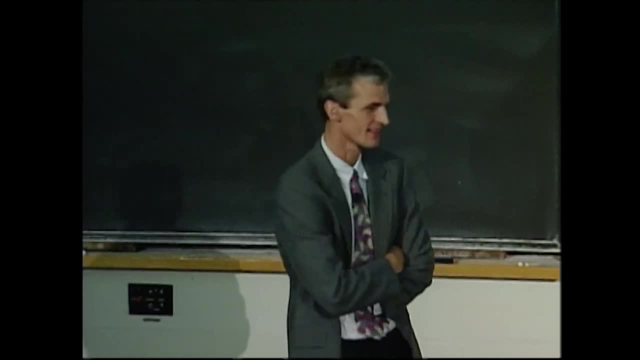 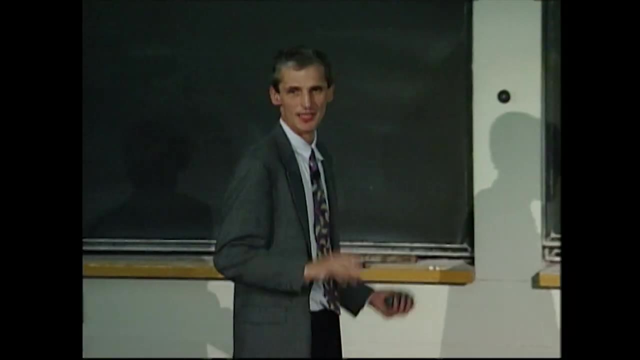 from the previous night's experiment. I think I told the students I didn't get any sleep at all And please, if I fall asleep during my class, ask me a question. So well, a few weeks later there was some short report in Tech Talk. 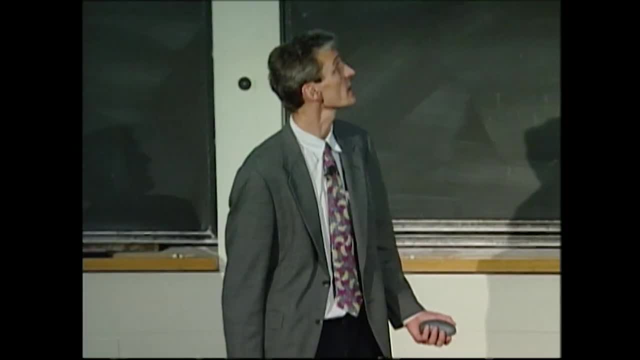 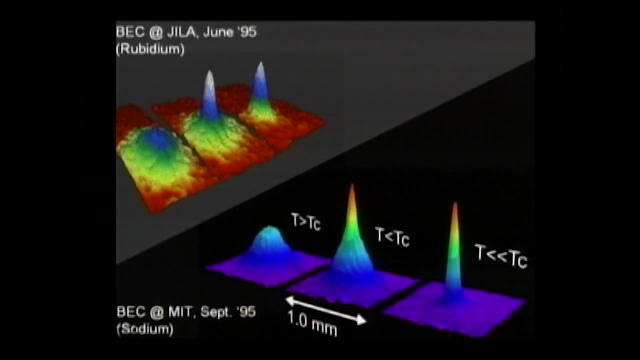 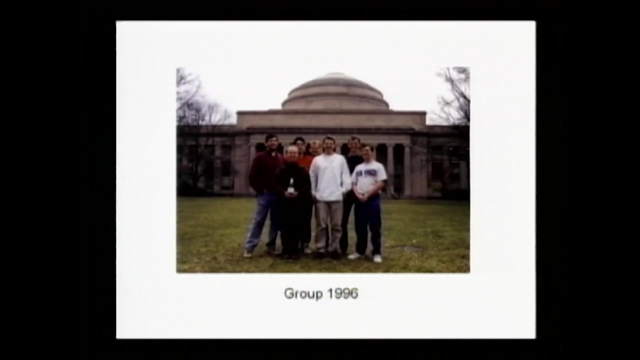 But this was the night where Bose-Einstein condensation was realized at MIT. OK, But immediately with our approach, we had 100 times more atoms And we had a system which was more versatile to pursue the new physics of Bose-Einstein condensation. 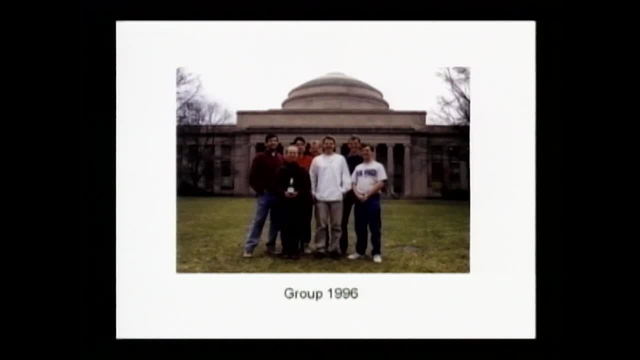 This is a picture of the group a few months earlier. It doesn't show Ken Davis, But it shows the people, the other people who were on board: Darlene Durfee, Mark Mavis, Michael Andrews, Dan Stamper-Kern, Klaas-Jan van Druten as a postdoc. 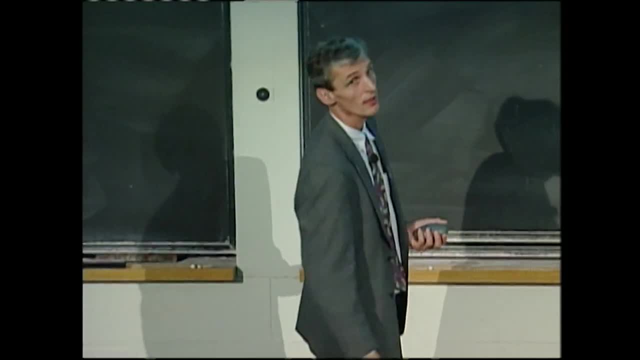 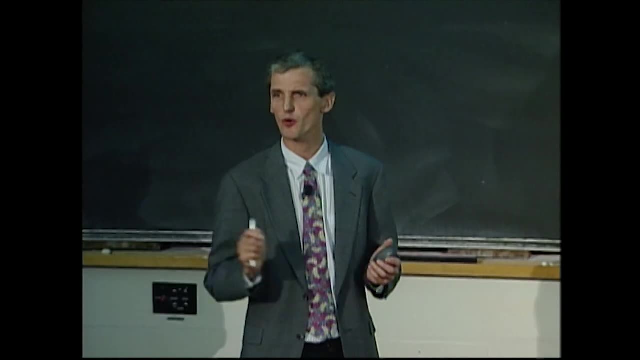 and Chris Townsend joined a few months after we saw BEC. Anyway, We were playing and I'll tell you a story of sometimes you do the right thing for the wrong reason, And this is when we changed our magnetic trap, which is really 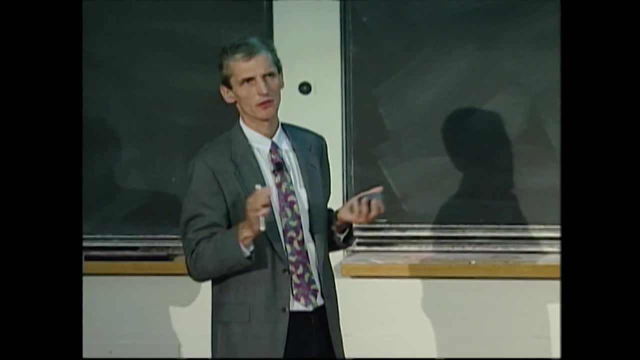 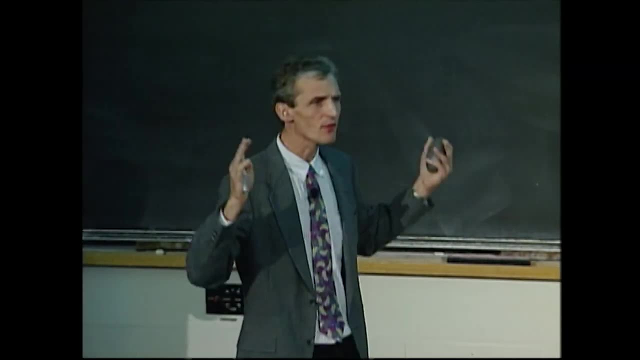 the core of the apparatus. We were one of the two or three groups. There was a little bit ambiguous observation by a third group who had seen Bose-Einstein condensation And everybody was brimming with excitement And I made a wrong assessment. 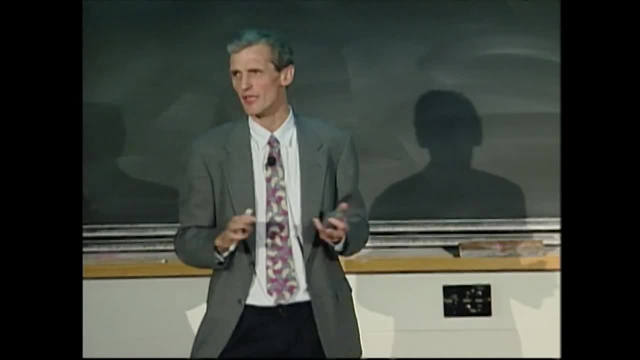 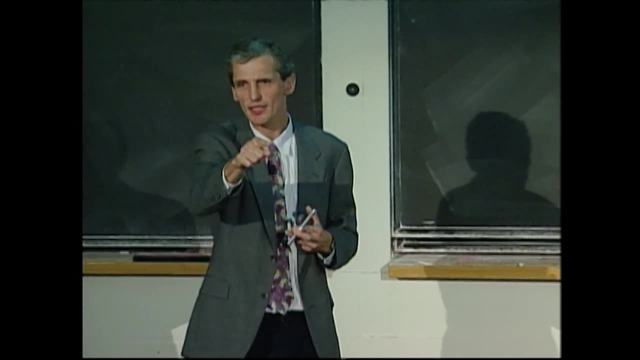 I said, hey, it wasn't really so complicated what we did. In the next few months many groups around the world will repeat it, And now we have to be really careful. Maybe with our jittery laser beam we're not competitive. 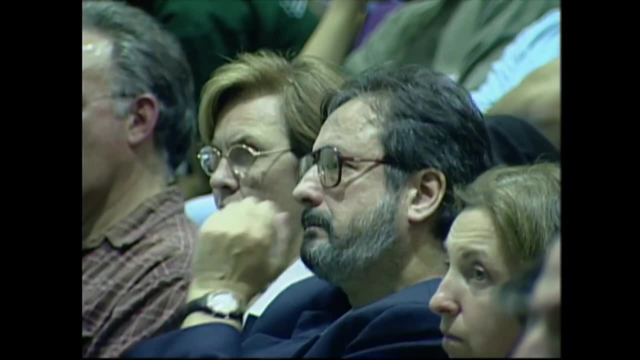 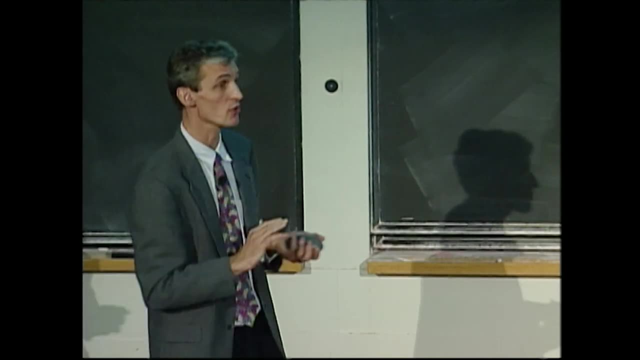 We really have to go forward and make an improvement And we thought: let's build a new magnetic trap. What happened actually is it took us five months to build it. We couldn't get any Bose condensation for the next five months. 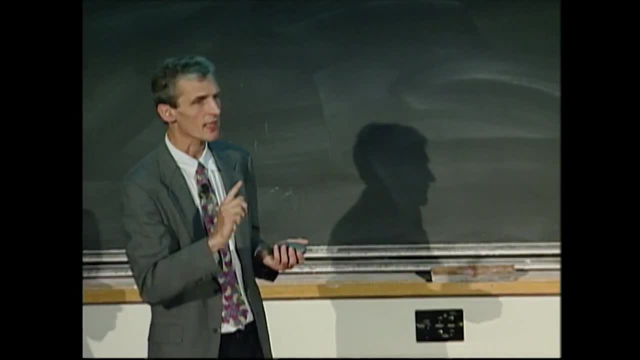 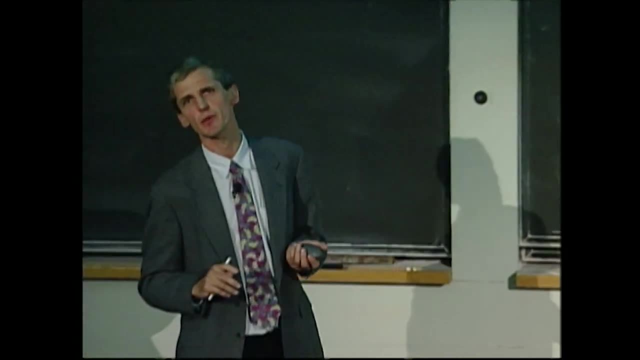 But when we got it we were really going like gangbusters. But my assessment was wrong, because nobody else got Bose condensation in the meantime. Indeed, to build such a complex apparatus it took two years for all the other groups. So if we had known that we would have probably just 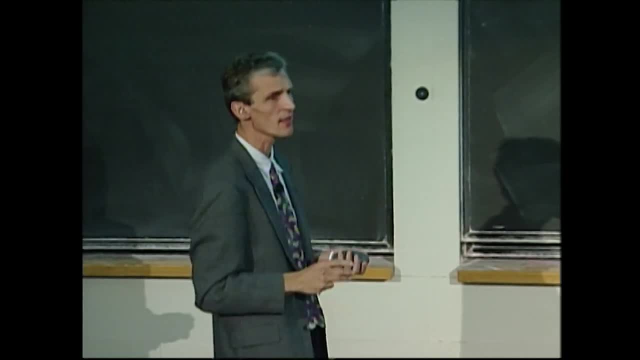 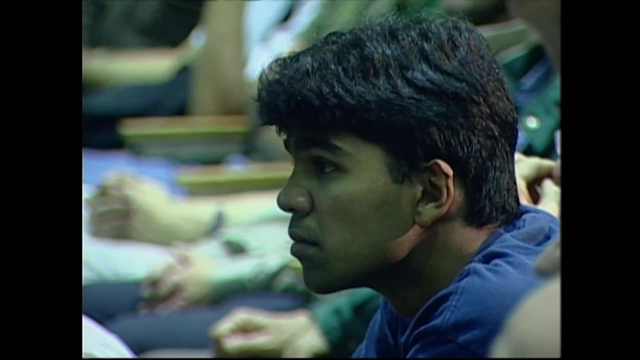 stuck to our original setup, But we went forward and created what turned out to be a really good trap and which gave us enormous productivity. So we realized this trapping configuration, which is not suffering from this leak. It's sort of a round bottom trap. 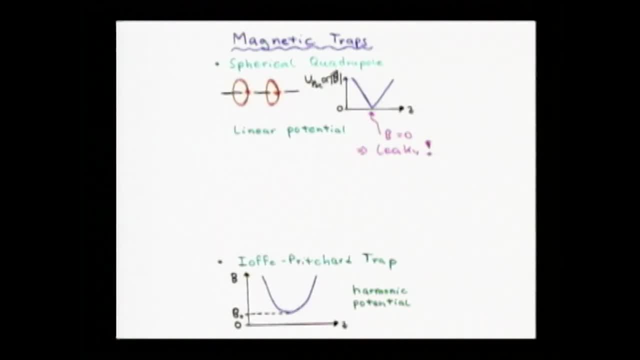 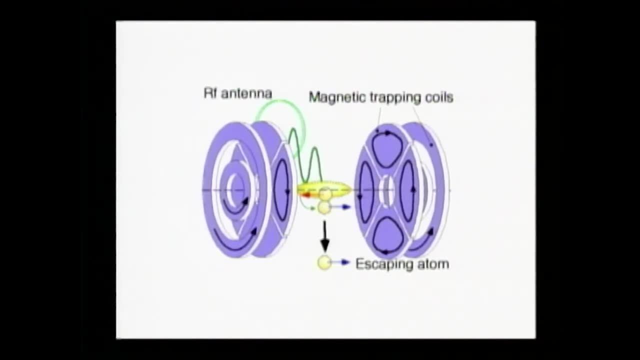 It actually carries the name Joffe Pritchard because Dave Pritchard suggested that in the mid-'80s And we found a new way to wind a trap. It's now referred to as a cloverleaf trap, And so well, this is how we have produced Bose condensates. 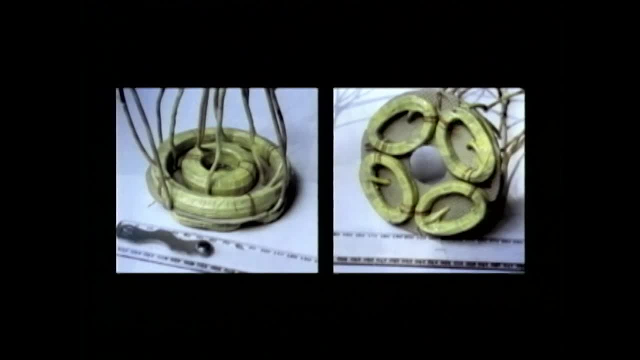 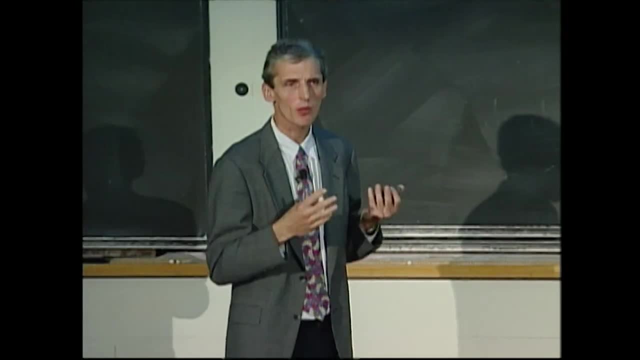 ever since. This shows you the actual winding pattern, And now I'll show you a few examples of what we were able to do in this trap. It was an enormously productive time, And one of my graduate students who was with me between 95- 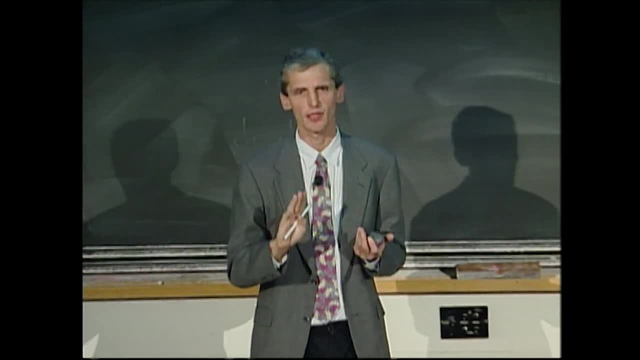 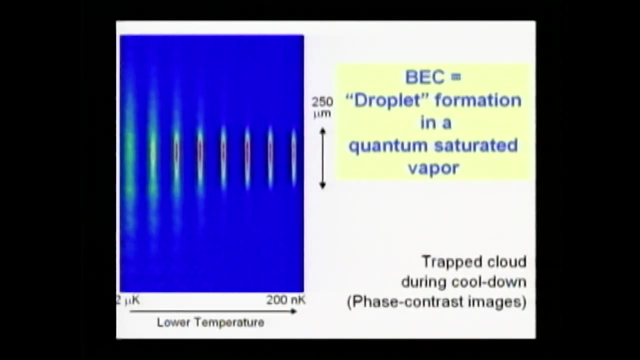 and 99, he graduated. He graduated with 20 papers in Fusrev Letter Nature or Science. So these were one of the first experiments we did in this novel trap. We could now visualize the condensate inside the trap using a novel light scattering technique. 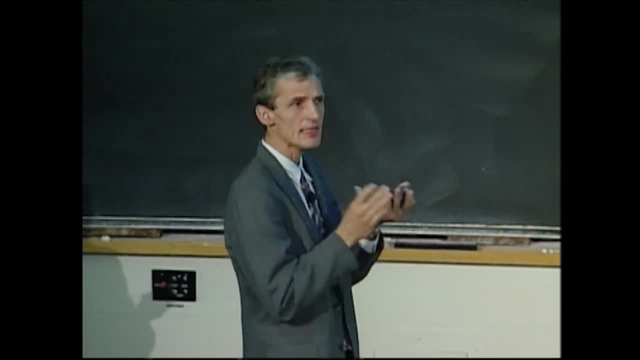 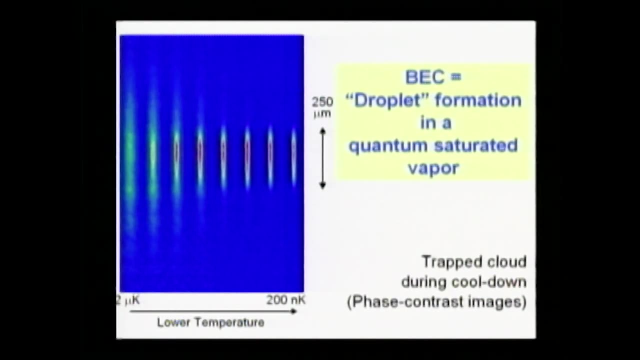 And now we could really observe what was going on inside the condensate. And here you see the cool down. Our magnetic container was elongated, So it's an elongated cloud and it shrinks as we cool And when we reach the phase transition. 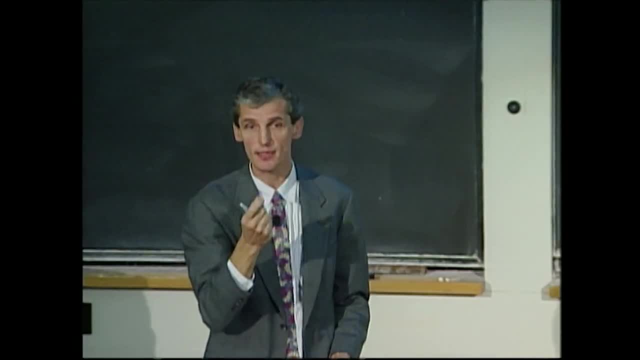 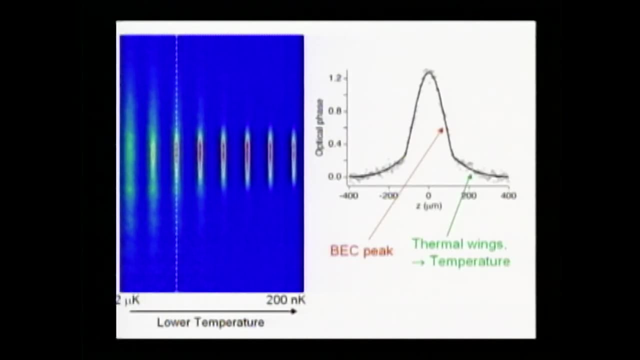 in the middle of the trap we see this formation of a dense core, the Bose-Einstein condensate, And if you just take a cut through this cloud, you can see. you know this. You remember the blue guys who march in lockstep. 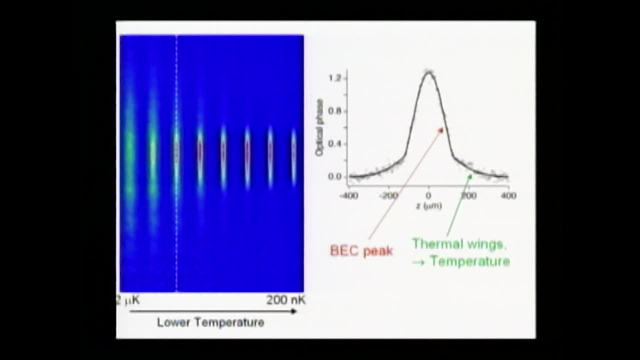 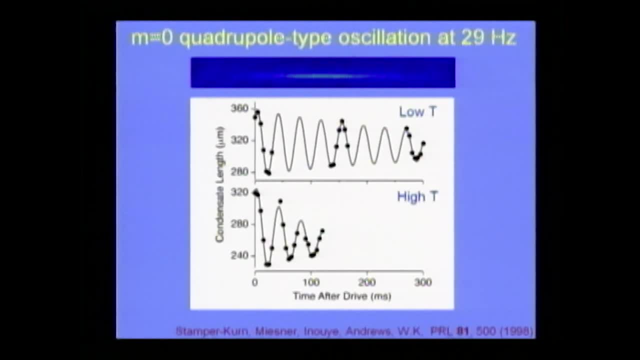 This is this peak, And then you have a thermal component. These were the colorful guys which were moving and whizzing around in all directions, And we did a series of experiments. Here you see a condensate set in oscillation. People call it the study of sub-condensate. 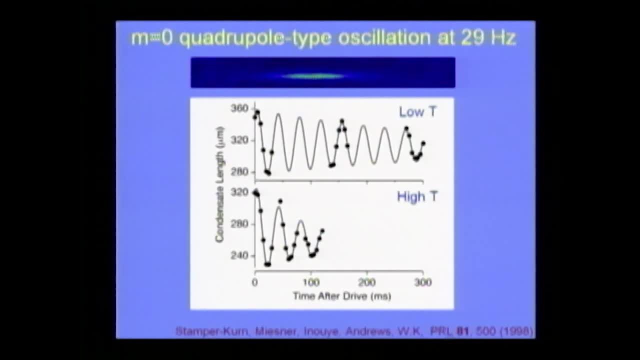 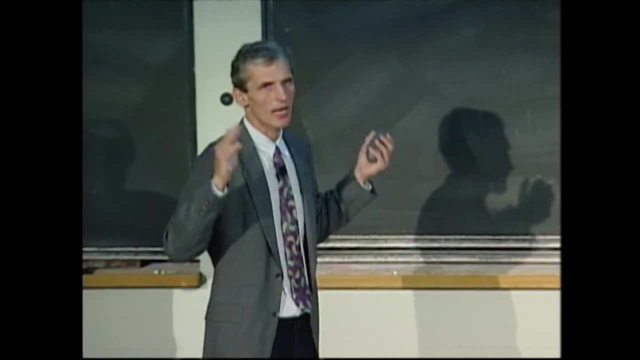 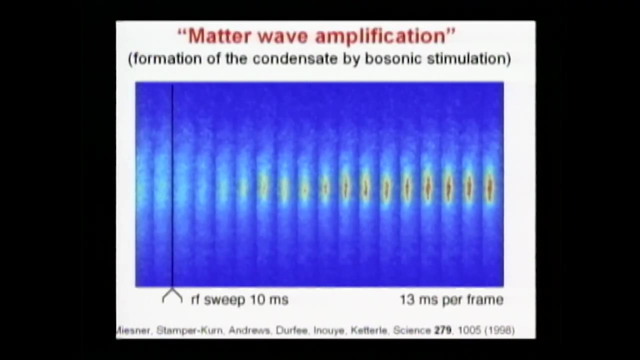 It's the sound and some of those results. what is the frequency of oscillation? what is its damping was really posing major challenges to many body theory and led to hundreds of theoretical papers. Or, something which I felt was very dramatic, Those nano Kelvin atoms. you think they're so fragile. 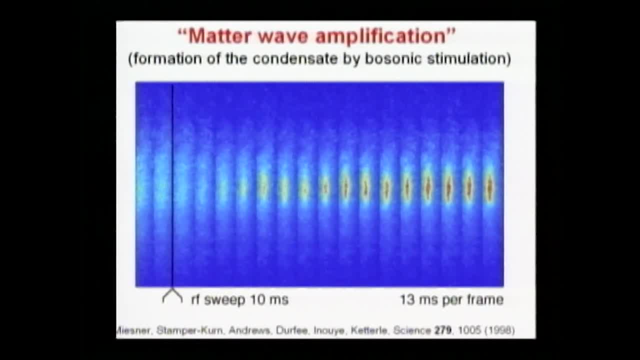 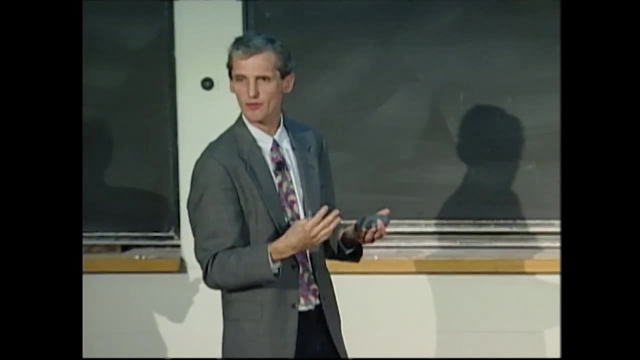 It's colder than anything else, But by using this light scattering technique and just troposcopic illumination, we could really see how color coded in red, how condensate formed. It was for me like watching how nature is giving birth to something which is very fragile. 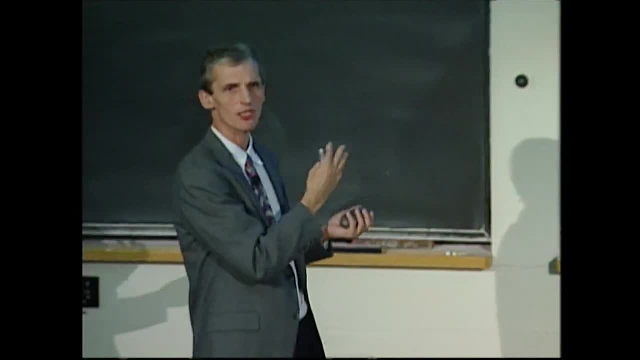 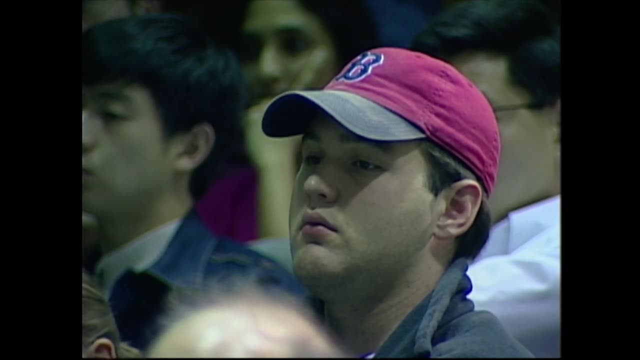 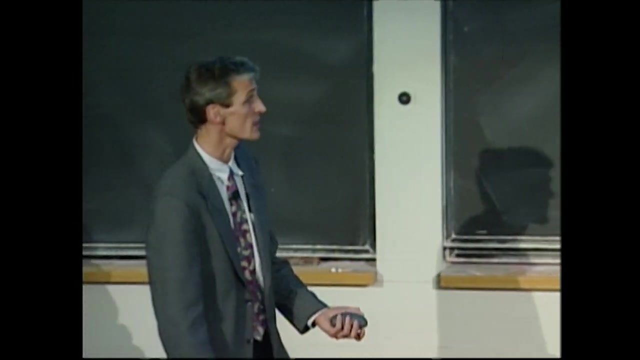 but nevertheless we were able to observe it in its natural environment And actually the way how the condensate forms was challenging theory And over many, many years now, quantum kinetic theory has been developed to some extent to explain the dynamics of the formation of the condensate. 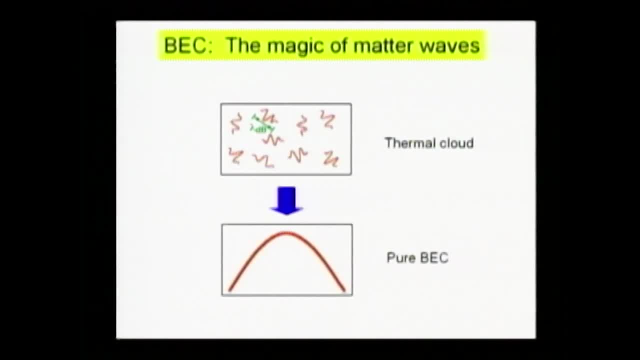 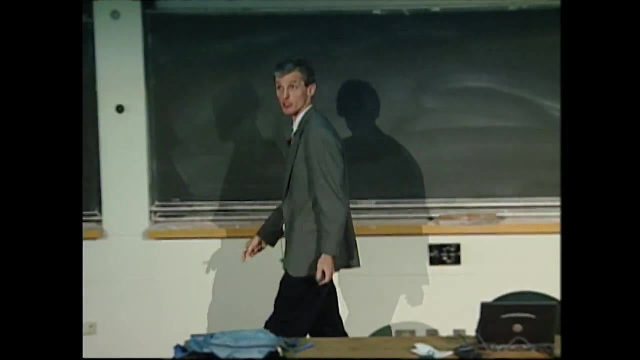 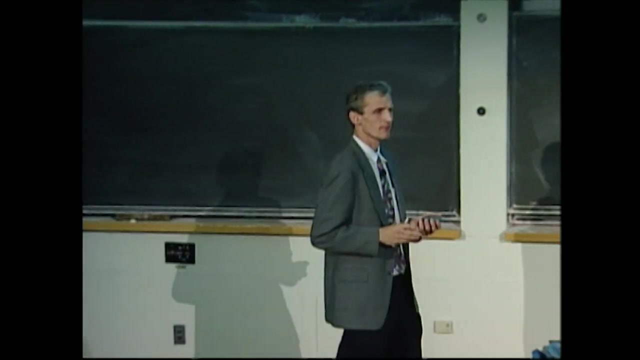 But let me now use talk about Two examples of our research which really demonstrates what makes Bose condensates so special. Now, if I talk to a lay audience or if I want to help you, if you meet your friends and you want to tell them what is really special about Bose, 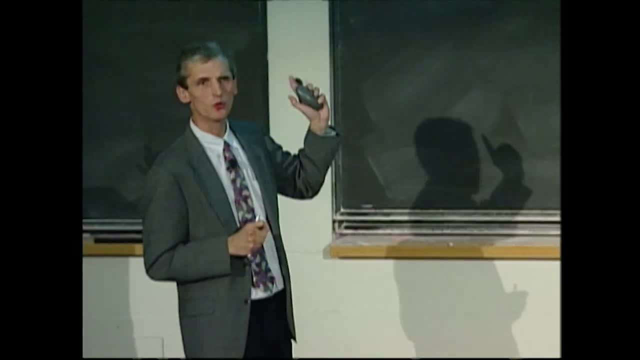 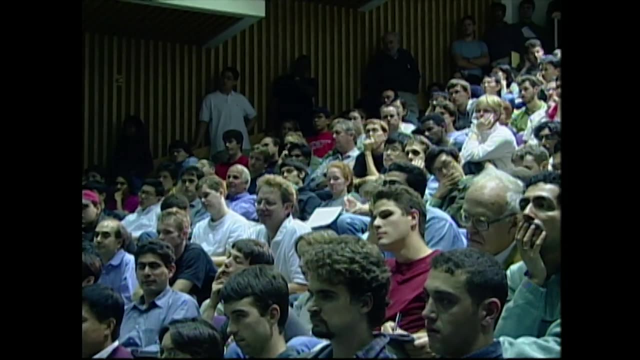 Einstein condensates. I want to know what is really special about Bose Einstein condensates. I want to know what is really special about Bose Einstein condensates. Now give you two examples how you can convince people that this is something which has unusual properties. 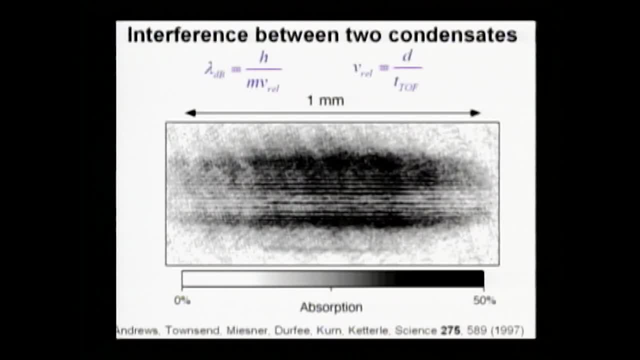 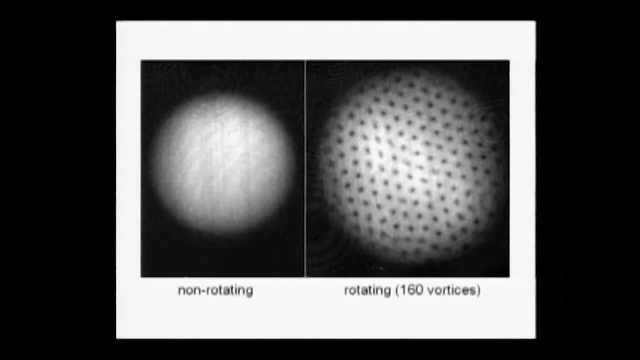 And it's really related to what I called here the magic of meta waves. And I want to show you two examples: the interference of condensates which allow you to directly photograph meta waves, And I want to show you the example of rotating condensates which have 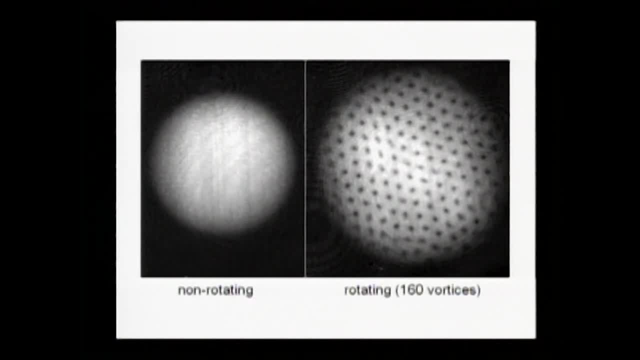 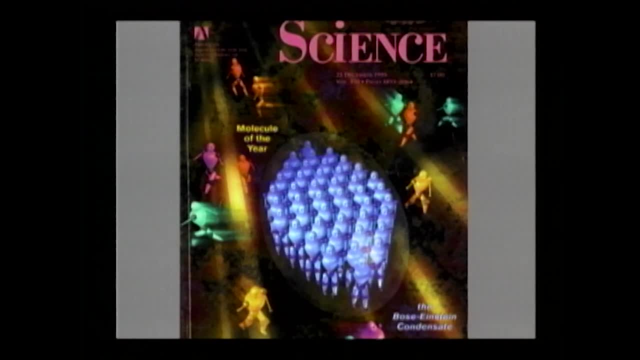 a Swiss cheese-like appearance. This is Very different from how any ordinary meta behaves. OK, What I want to explain you now, the interference between condensates was actually a key experiment which we did, And it was also actually one of our key contributions. 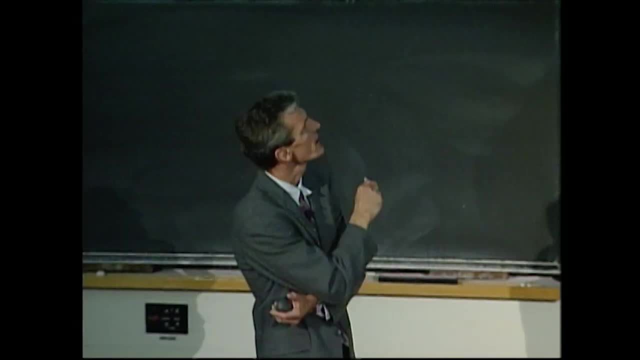 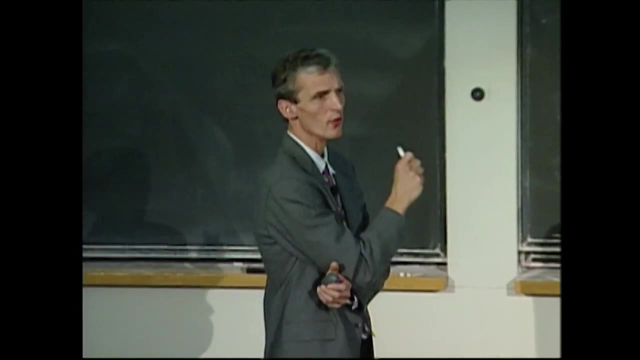 which was emphasized by the Swedish Academy, Because what we could do in 96- and publishing in 97, was we could show for the first time that the condensate is not really cold, So while coldness is relative, but that it. 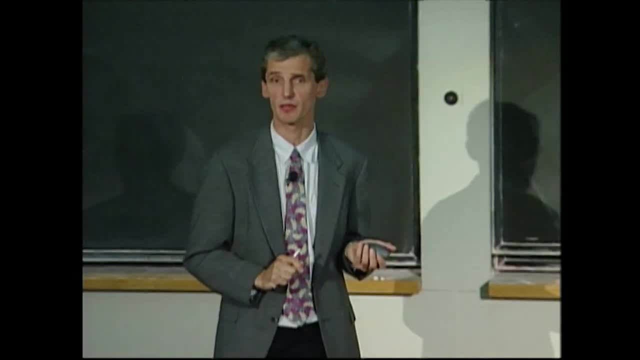 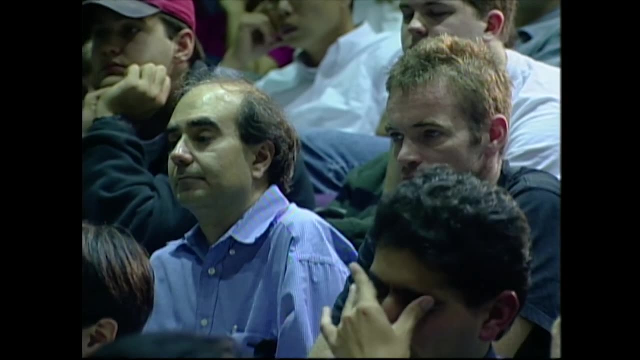 has these special properties, that all the atoms march in lockstep, That they are just one quantum mechanical meta wave. OK, If you want to show that something, if you want to show, for instance, that this laser beam is an electromagnetic wave, the best way to do it. 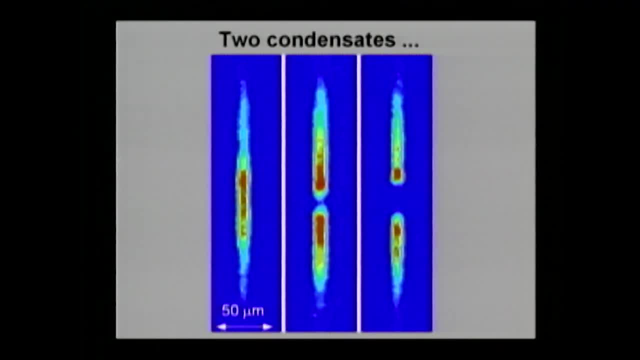 is, you take two laser beams and interfere them, And then you see an interference pattern. The interference is the clear evidence for the wave nature. So we needed two condensates. And so well, by using a laser knife and cutting a condensate into two pieces, 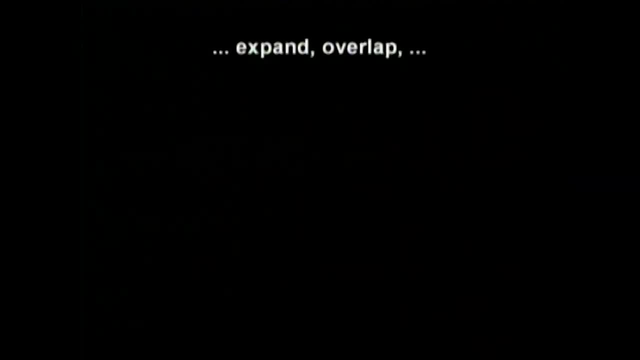 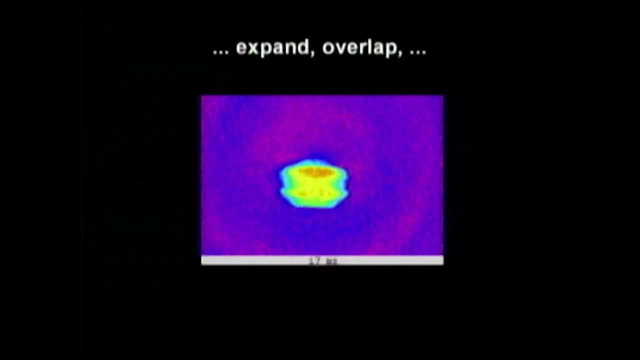 forgoing all the details, we created two condensates, And so now we had two condensates And we switched off our magnetic container And the condensates. well, if you switch it off, the condensates fall down due to gravity. 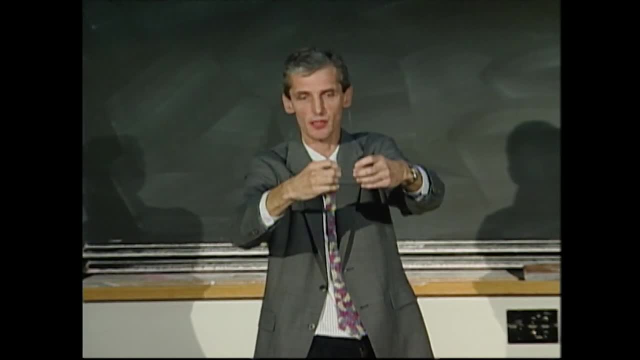 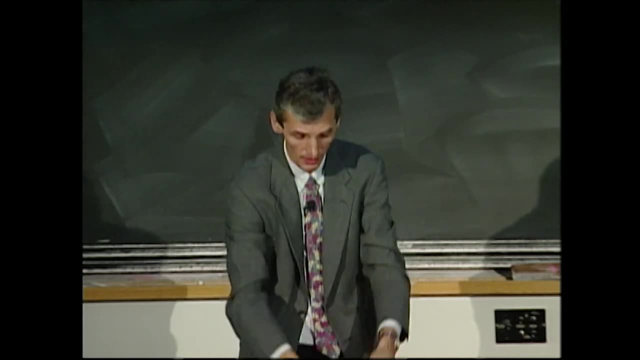 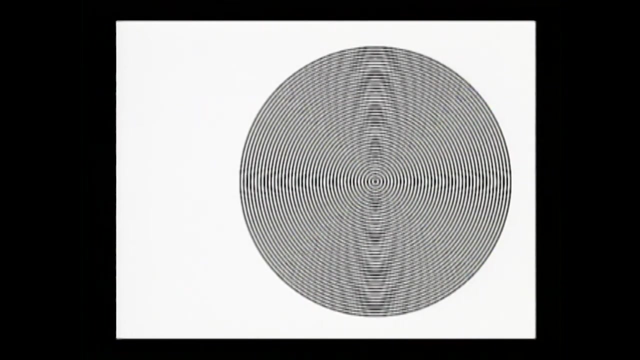 But they also expand because of zero point motion and atomic repulsion. So what we are hoping for is, as the two condensates expand into each other and overlap, to see the wave nature of those atoms. So let me show you what we expected to see. 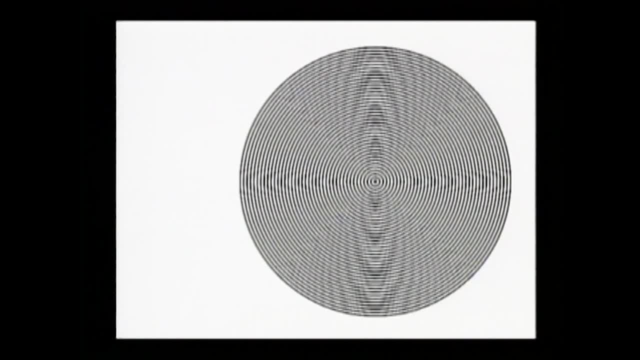 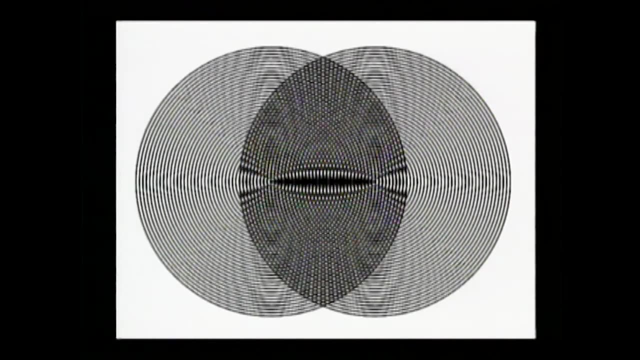 So let me just give you an example for the interference between two sources. So assume that this is the antenna of our favorite radio station in Boston And it radiates radio waves, And now we bring in a second radio station, and now the waves of the two radio stations. 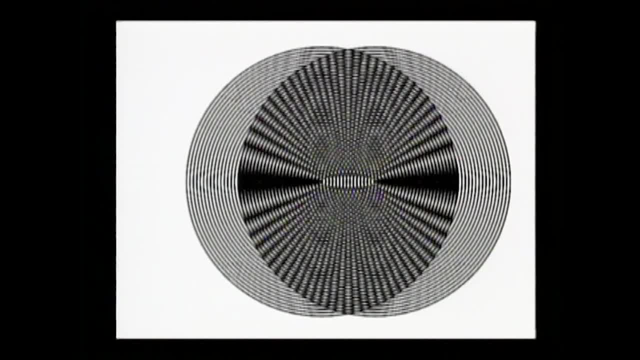 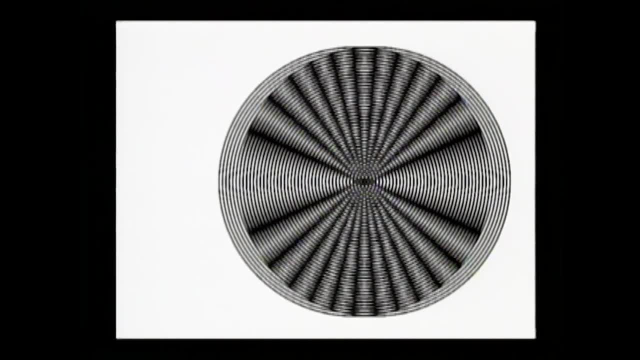 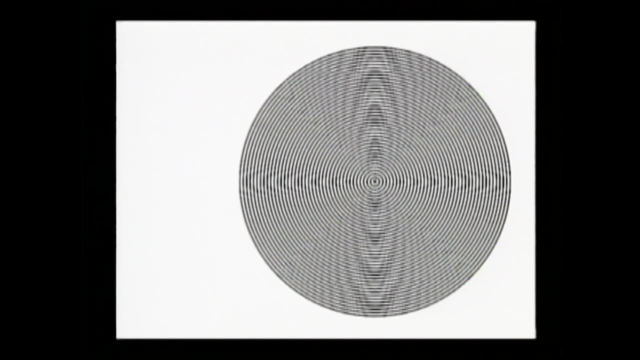 interfere. And now you see the interference pattern. And of course the interference pattern becomes more macroscopic the closer the distance is. And at least those who took 803, they should realize that this interference pattern has the form of parabola. 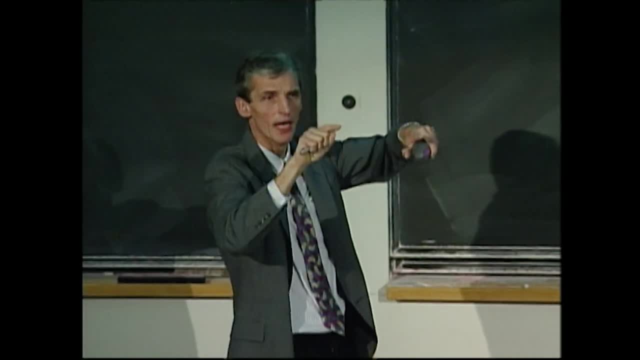 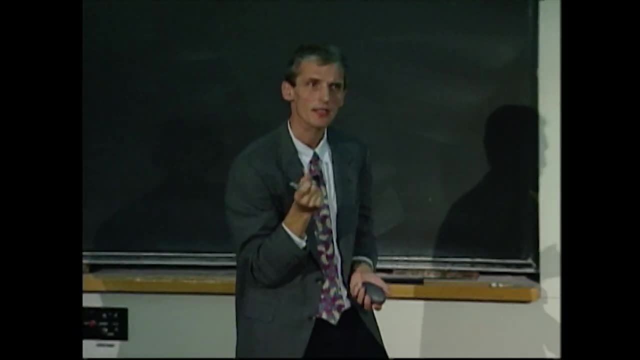 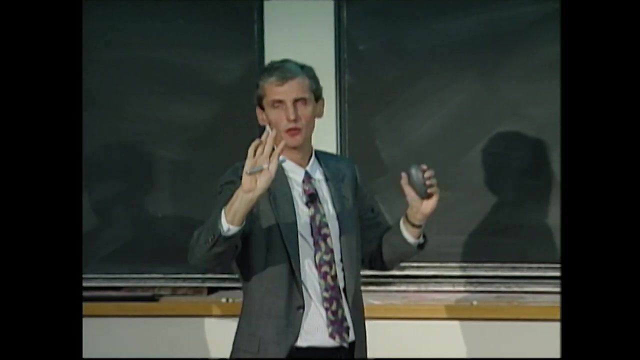 Because a parabola is a mathematical curve for which the path length difference to the two origins is constant. So well, we are not interfering radio waves, We are interfering matter waves. So we have our container, the atoms spread out. And now I have to remind you, probably, 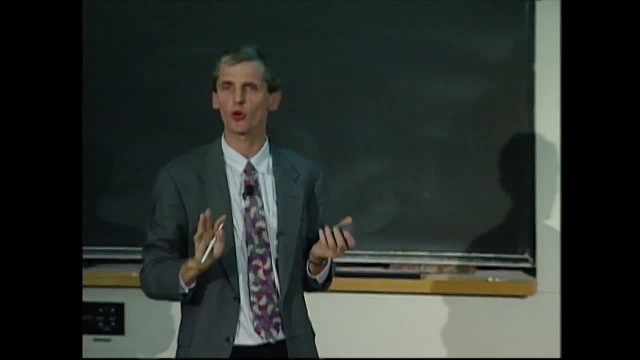 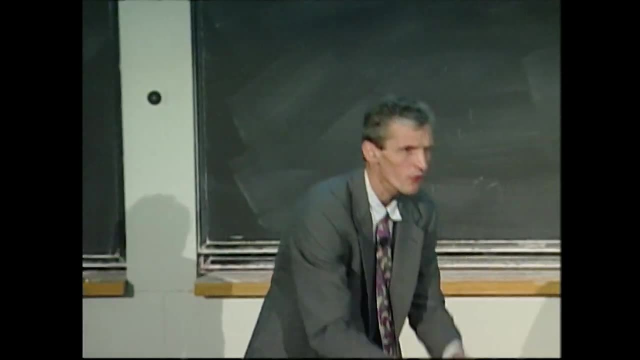 of pretty much the signal equation. I showed you the de Broglie relation. The faster the atoms are, the shorter is the de Broglie wavelength. So if we have a puff of gas and let it go and then take a snapshot, the atoms which are further out. 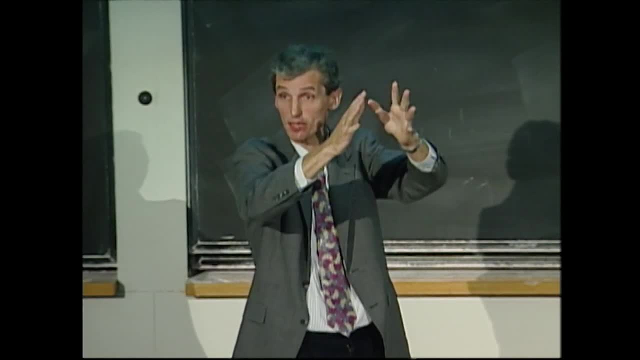 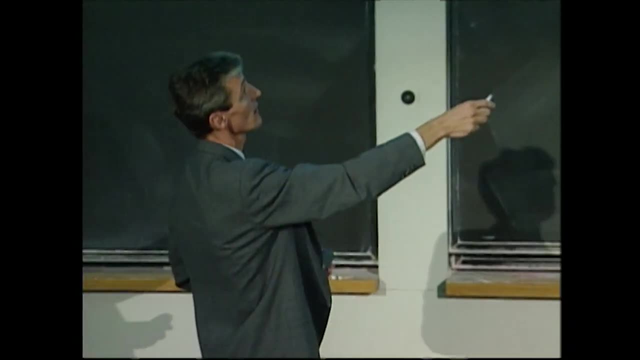 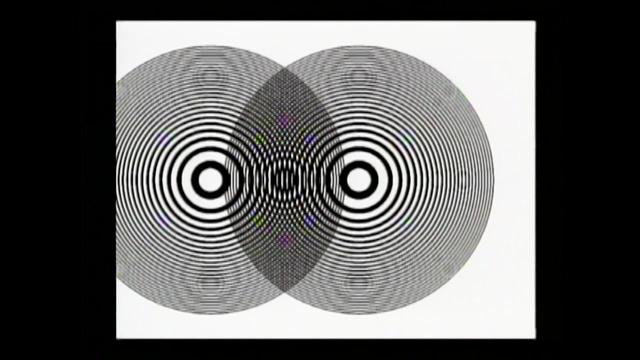 they have moved, They're faster, And the atoms which are closer in they are slower. So the wave pattern of such a pulsed matter wave looks like this: The matter wavelength is longer where the atoms haven't traveled so far and it is shorter where they have traveled further. 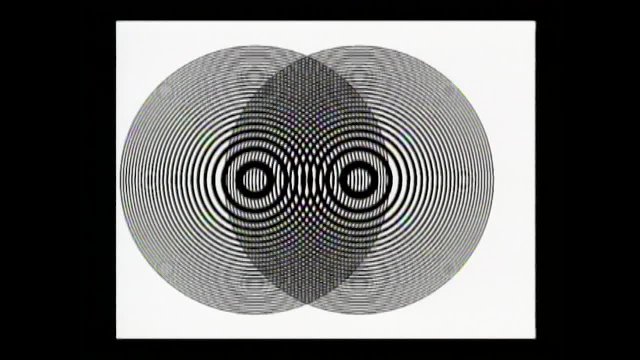 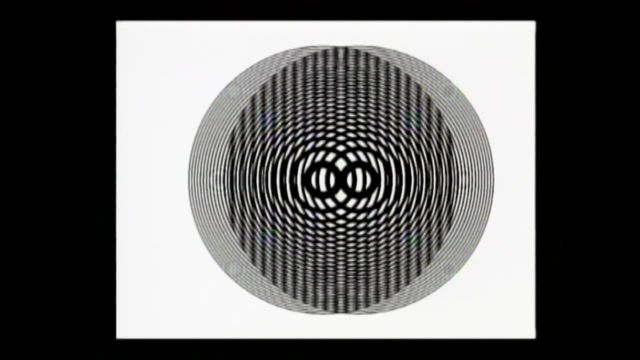 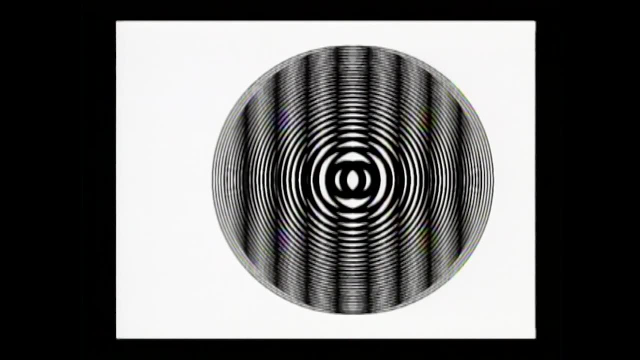 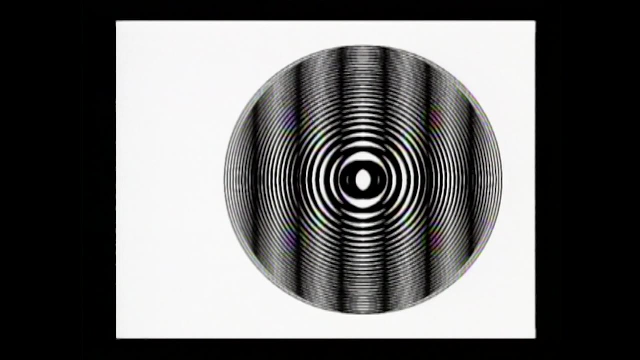 So now we interfere our two Bose-Einstein condensates And you again see now, as we bring them closer together, that there is a distinct interference pattern. But in contrast to the two radio stations, this interference pattern consists of perfectly straight lines. And when we observe the overlap of the two condensates, 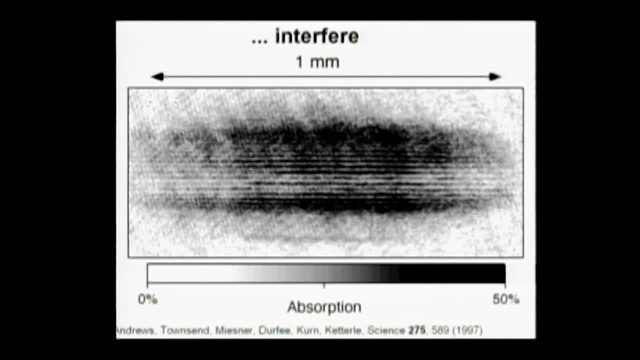 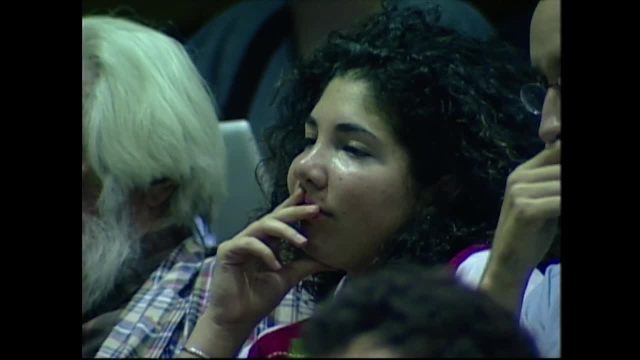 and we saw that we were really jumping up from our chairs And I think I remember the first night we saw that again, we had worked until the wee hours in the morning. I think it was you, Dan. you came in at 8 or 9 o'clock. 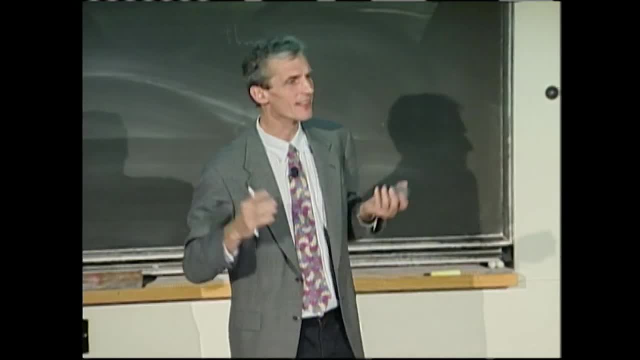 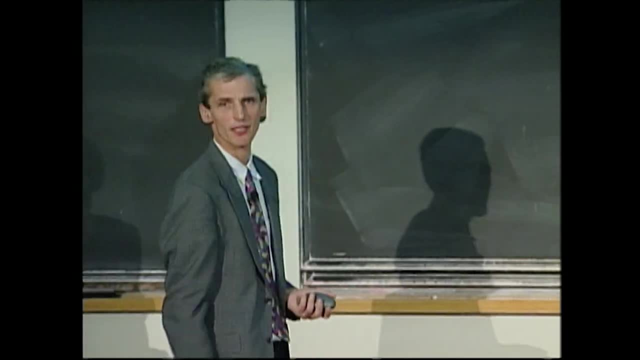 And I was almost drunken And I came to Dan's office- Dan, I have to show you something. And Dan came to the office, Dan came to the lab And we had this pattern on the screen. So we knew the Bose condensate is a coherent form of matter. 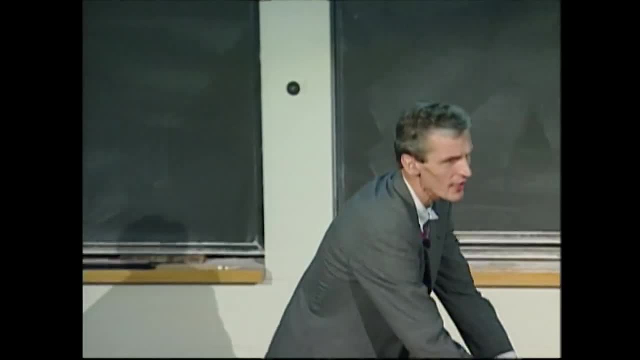 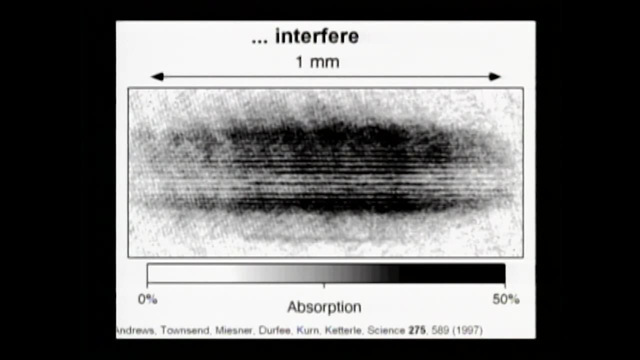 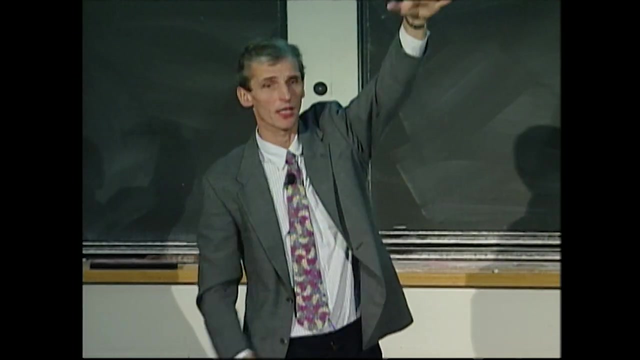 Actually just to talk in terms of layperson, what you actually see here is two things. One is- this is a direct observation of the wave nature of matter- We simply take two puffs of atoms- They overlap- And then we illuminate the atoms with a laser beam. 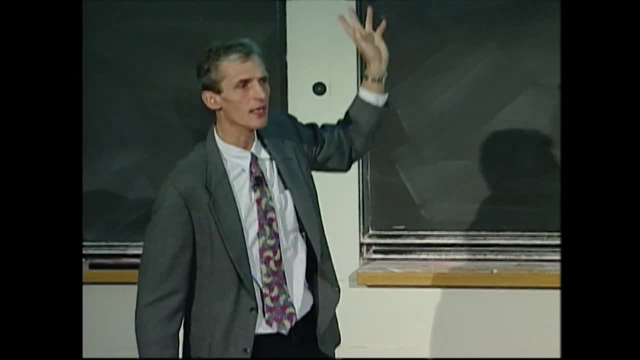 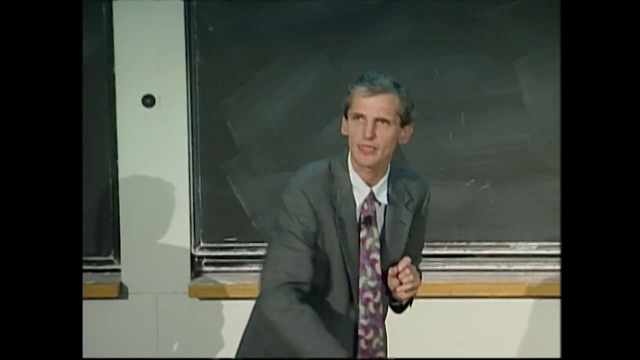 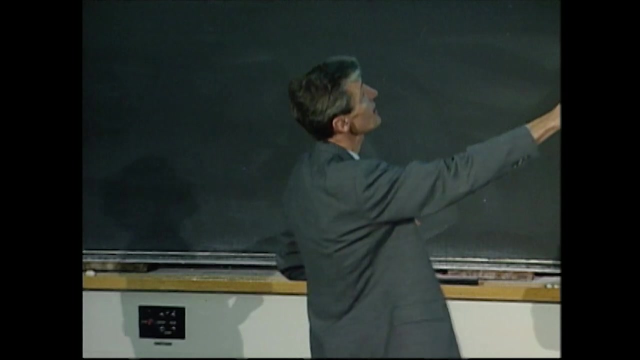 And we take a shadow image. It's the most direct observation of the wave nature of matter. But secondly, this is also demonstrating in a fairly dramatic way this equation that atoms plus atoms gives vacuum, Because where there is no shadow, there are no atoms. 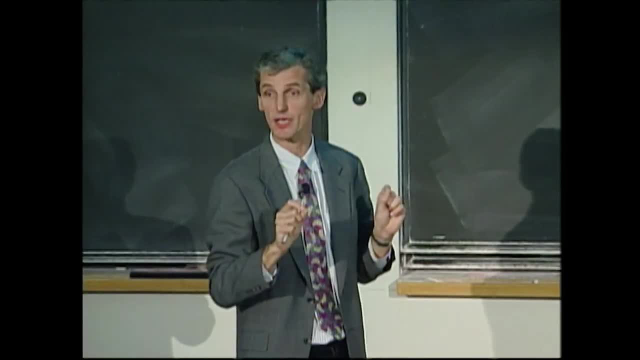 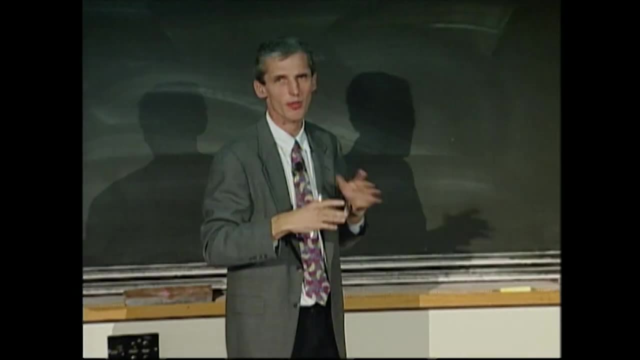 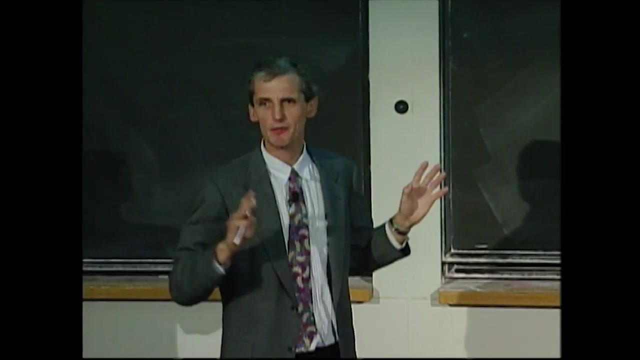 So the two matter waves have interfered each other away. Atoms plus atoms gives vacuum. I mean, I sometimes get fan mail from people who have their own theories of physics And I got some questions about: yeah, what happens if you annihilate atoms by interference? 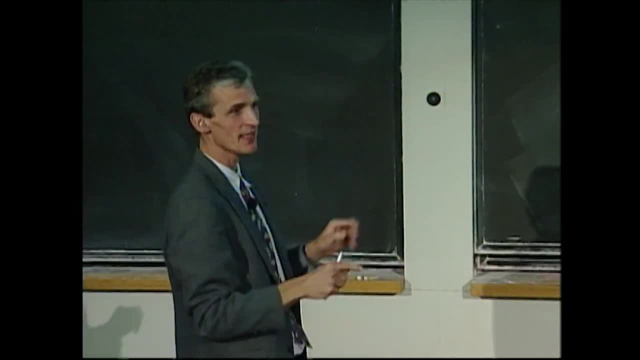 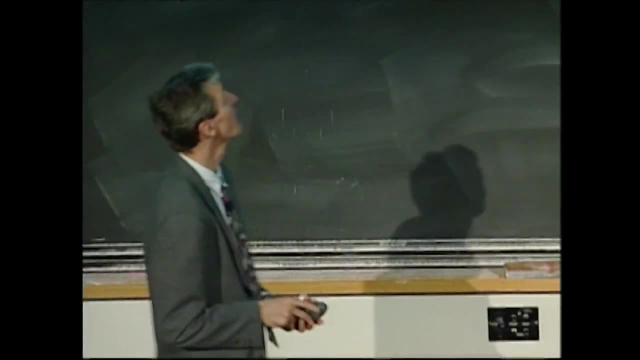 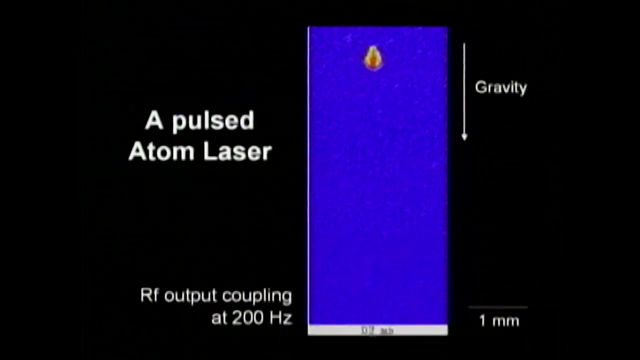 But I think you all know the atoms which are missing. here. they appear in the dark fringes Because atom plus atom equals four atoms if you have coherent interference. So this is just a different, more fancy representation of that. At about the same time we found a trick. 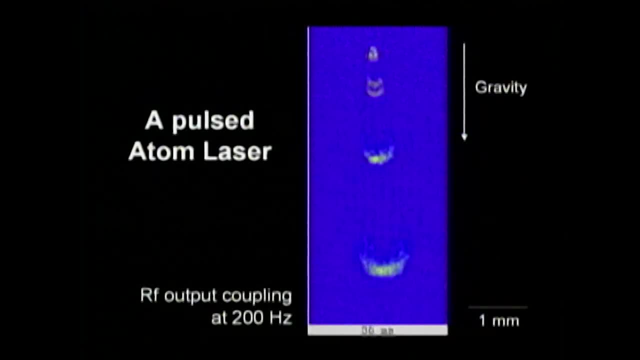 to release atoms out of the magnetic trap. We were just sort of spin-flipping atoms. They were accelerated down by gravity, And so within a few months we had done two things: We had shown that the atoms are laser-like, And secondly, we were able to create pulsed beams of atoms. 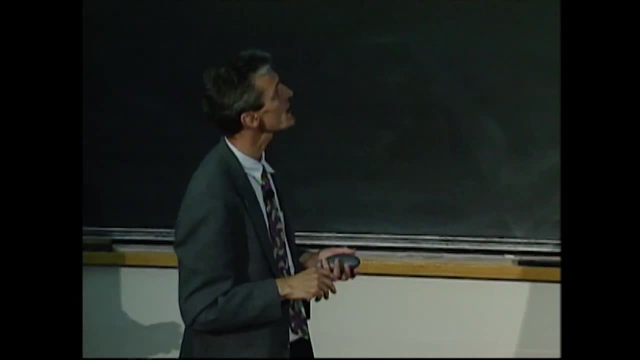 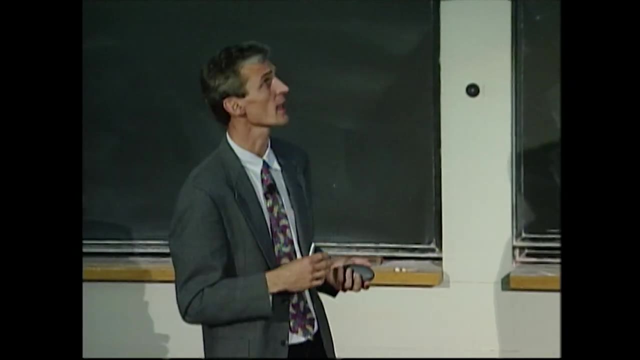 And this together is now recognized as the first realization of an atom laser: An atom laser, An atom laser which emits atomic matter with laser-like properties, And other groups have followed and improved on that. So this is sort of an atom laser gallery. 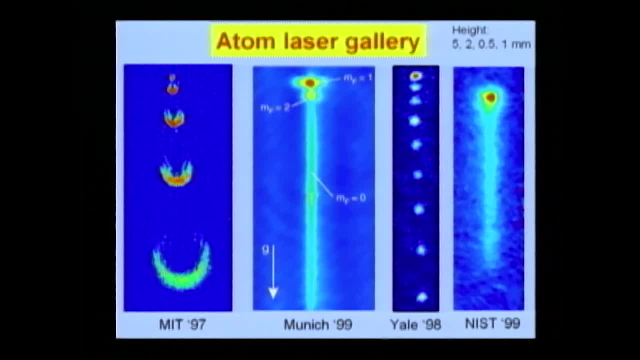 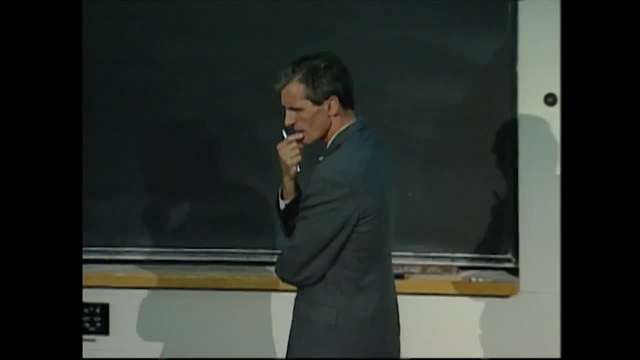 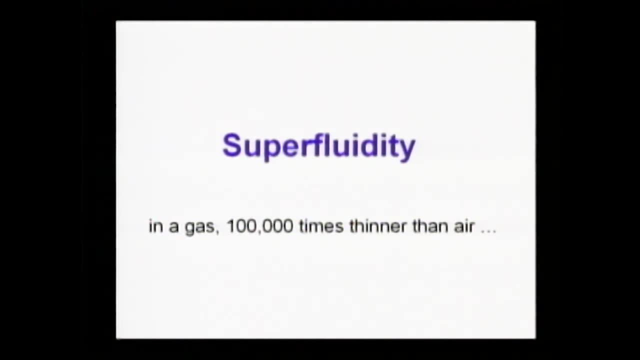 continuous atom lasers and different ways. It's a rich field and there is a lot to be done. Let me now talk about this other example where the wave nature of matter really becomes manifest, And this is actually related to a very 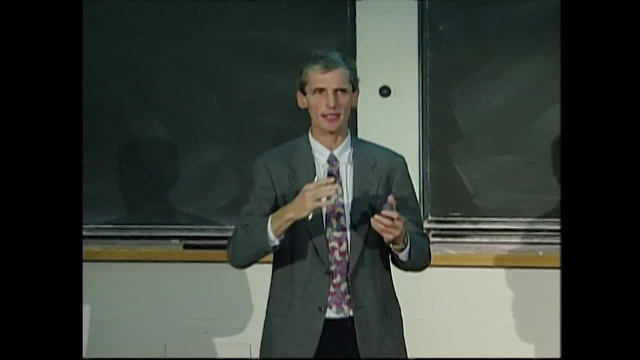 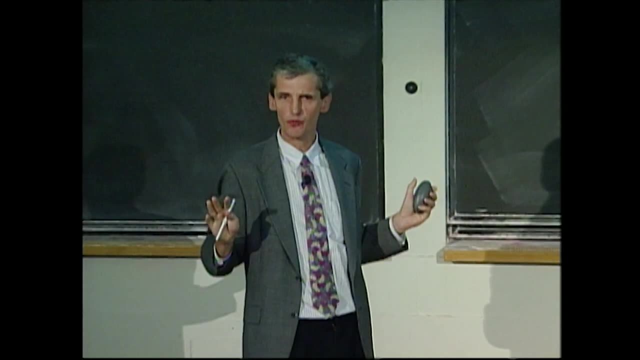 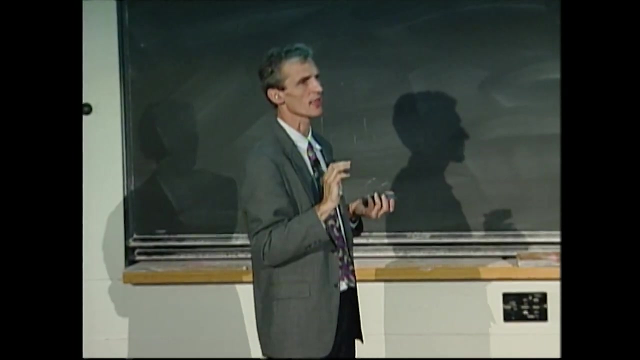 very special property of the Bose condensate. The Bose condensate is sort of one giant matter wave And it's possible for a wave-like matter to move, to propagate without any friction. There's one similar system which has enormous technical importance, and these are superconductors. In superconductors, electricity can flow without any dissipation. You can switch on a ring current and you can go home, and months later the ring current still flows without any active power. Those phenomena are usually dubbed super superconductivity, for electrons superfluidity. 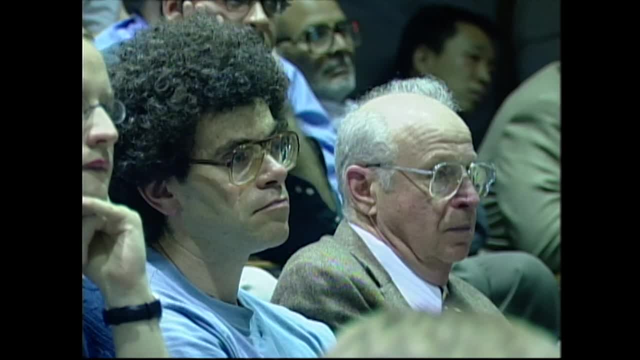 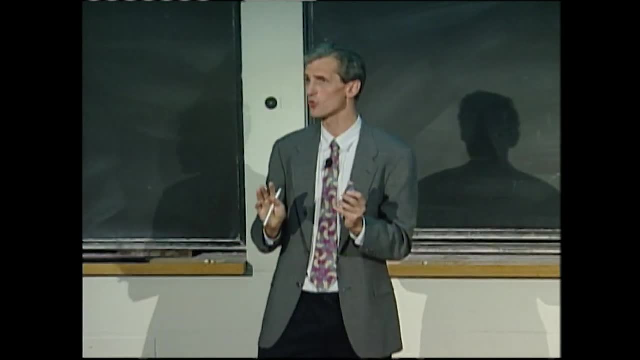 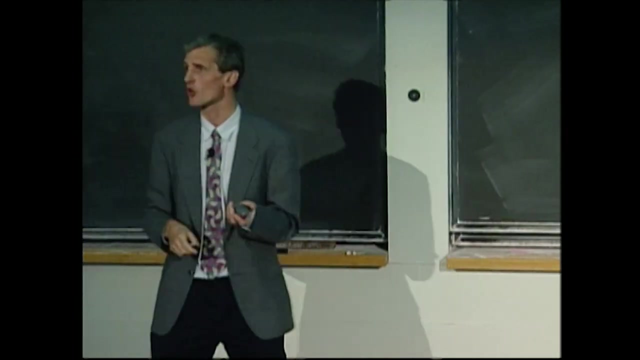 for liquid helium. And here we have a system which was predicted to be superfluid. but it's a gas. It's eight orders of magnitude more dilute than liquid helium. So we have the most fundamental system in our hands to understand details of superfluidity. 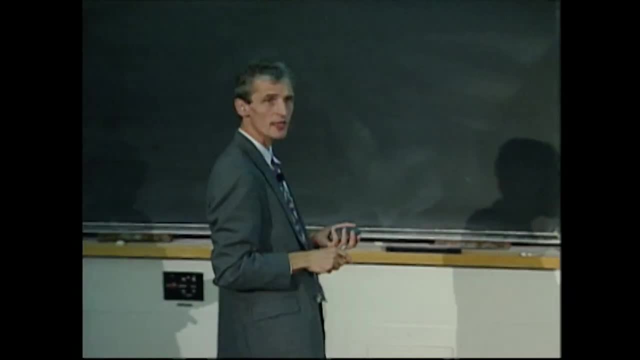 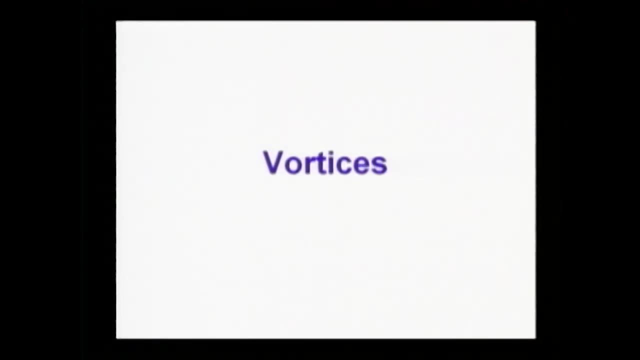 or macroscopic random phenomena. I don't want to talk. I want to go into details and rather emphasize one aspect which is fairly directly connected to superfluidity, but I'm not really explaining it- And this is the physics of vortices. 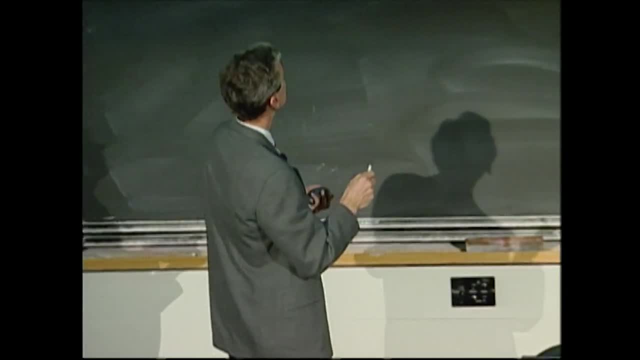 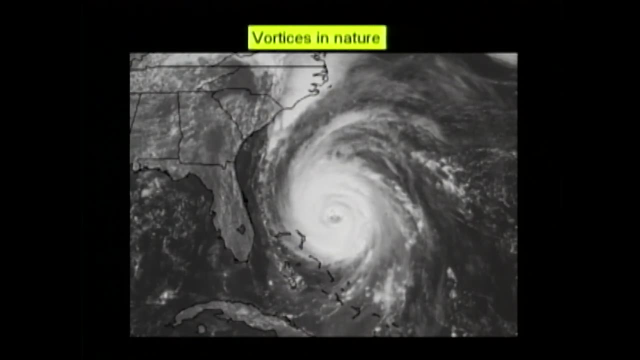 Now, I think you're all familiar with vortices. This is a vortex on a very large scale. You see a hurricane off the coast of Florida. I think we also encounter vortices in our everyday life. At least, I produced one today. 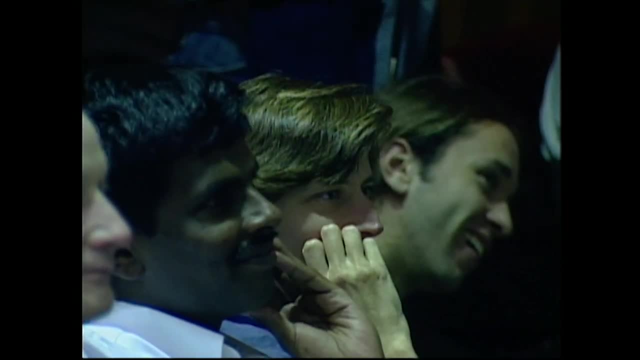 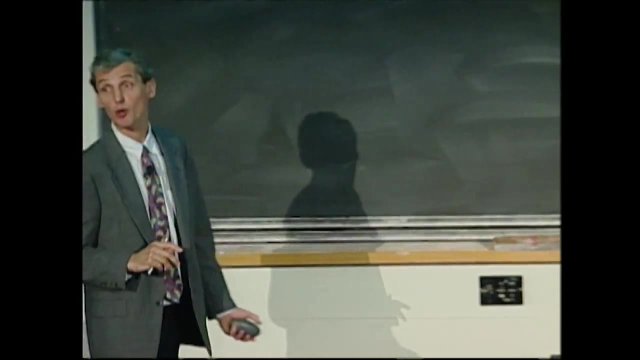 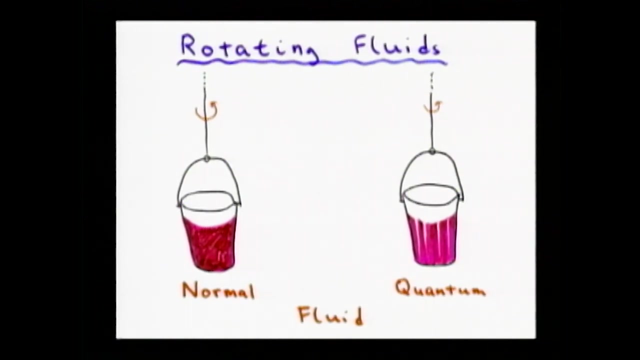 You simply push the button and you create a vortex. So what is special about vortex physics? OK, there's something important difference And that's what I want to explain. Let's consider this rotating bucket experiment And I want to show you that there. 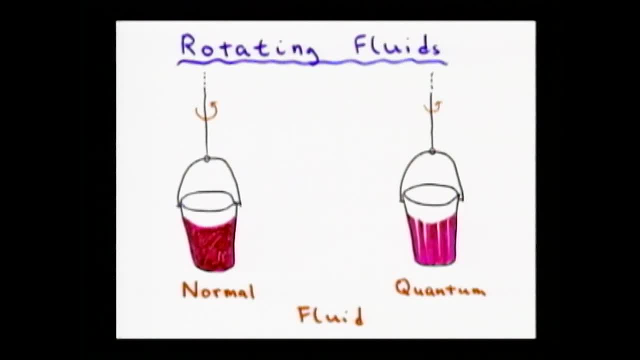 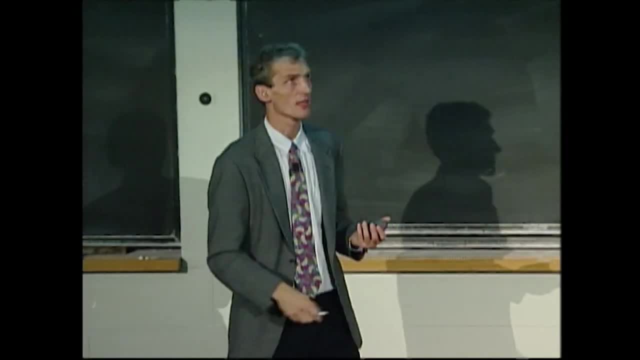 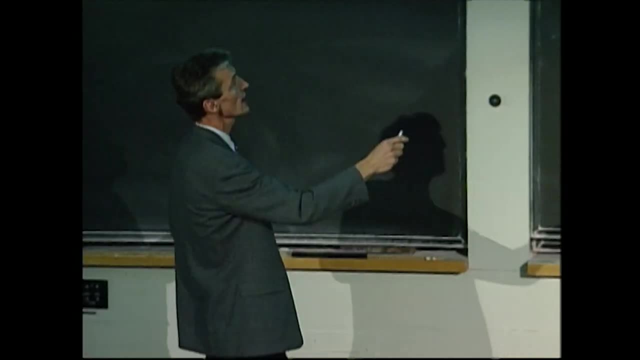 is a dramatic difference between rotating an ordinary fluid- let's say a bucket full of water- and rotating what I call a quantum fluid. And this is a system. This is a system where all the particles are just one big wave. First of all, if you rotate a normal fluid, 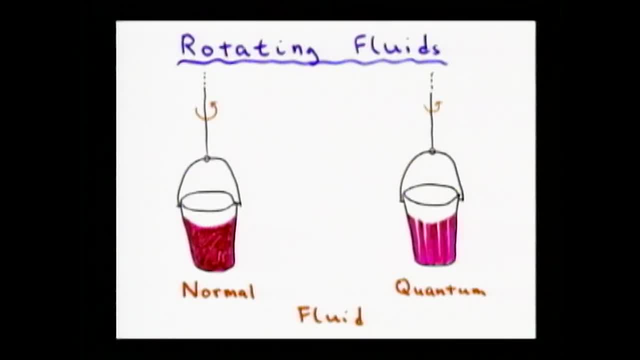 you know that upon rotation it forms this parabolic surface because of centrifugal forces. If you take, for instance, superfluid helium and you do the same I just told you there's a big difference, But the same happens: It's a parabolic surface. 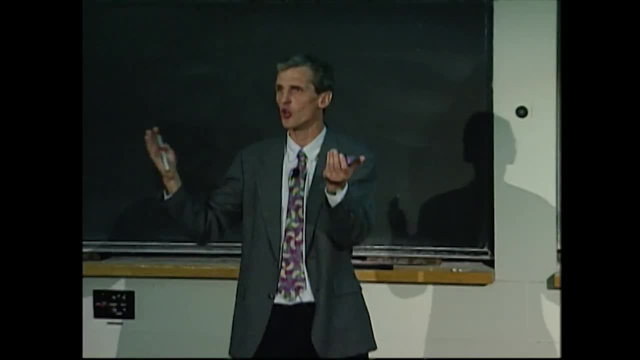 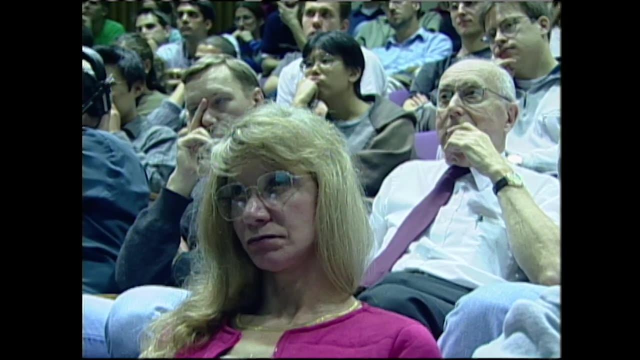 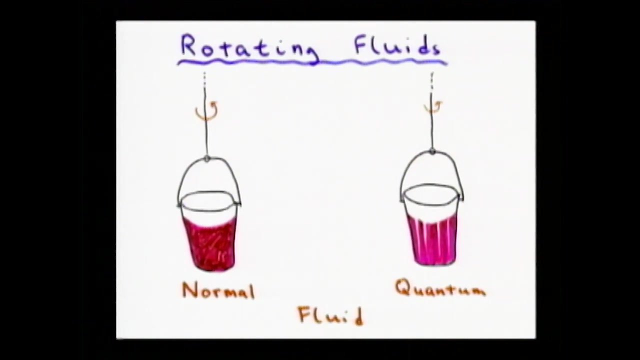 And it has to be like this because on large scales there's a correspondence, equivalence between a classical system and a quantum system. But if you now look a little bit closer onto the quantum system, you will find that the system is riddled with tiny little holes, tiny little vortices. 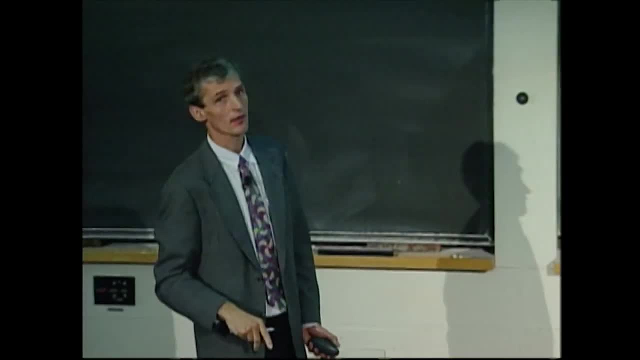 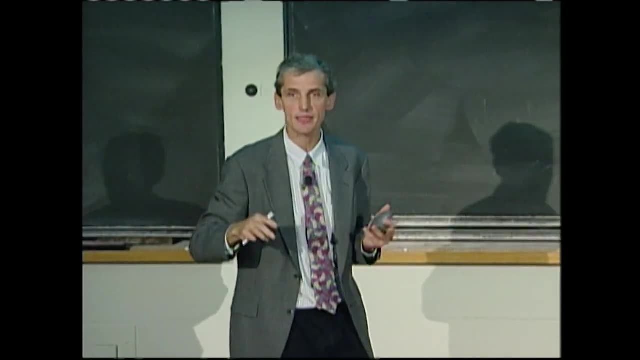 So there's a big difference And I want to explain that to you. The reason is the magic of matter waves. We're not asking particles to go around and go around. We are asking waves to go around And due to the laws of quantum mechanics. 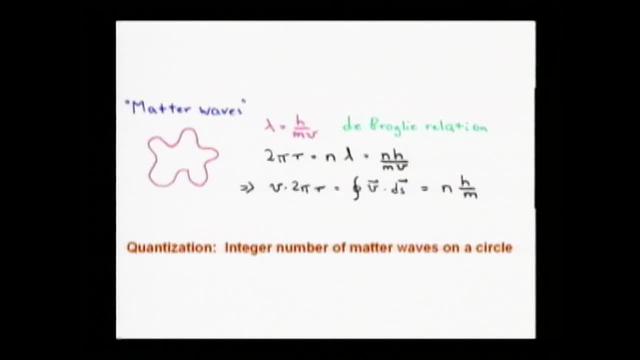 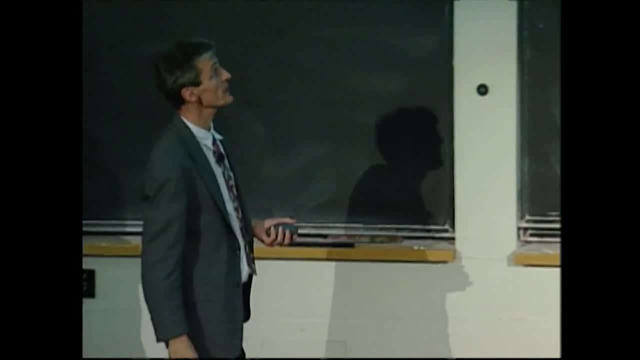 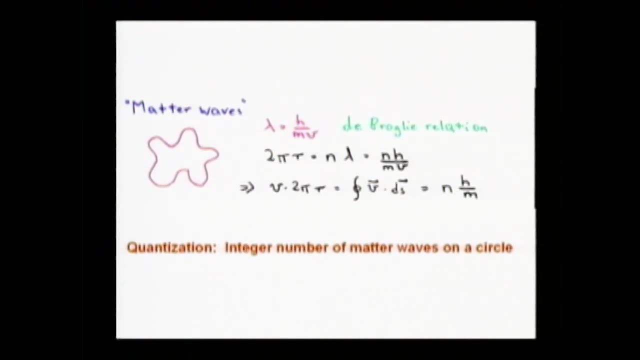 we have a snake of waves, And the snake has to bite into its tail, It has to form a closed wave. So therefore we have the quantization condition that we need an integer number of de Broglie wavelengths around the circumference. So that means now, if you rotate the bucket, 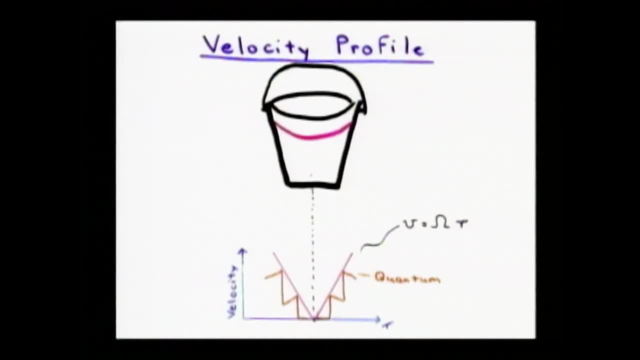 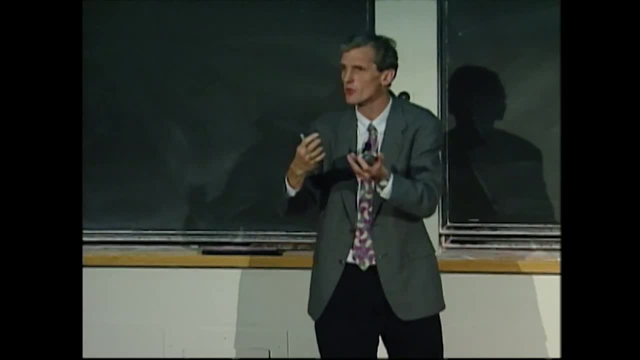 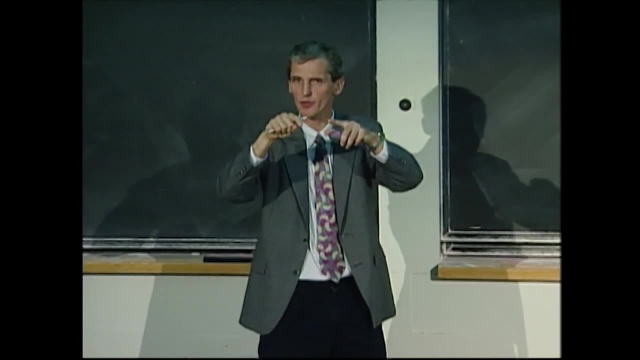 the classical system, just rigid body rotation has a velocity which increases linearly with distance. But the quantum system is not the same. The quantum fluid, the quantum gas cannot do it Because it has sort of to make a decision. Zero matter waves around the circumference one, two, three. 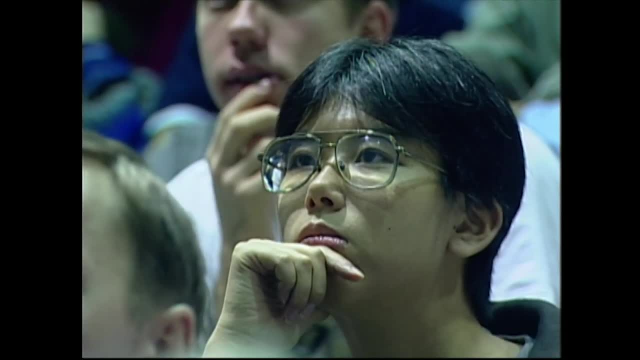 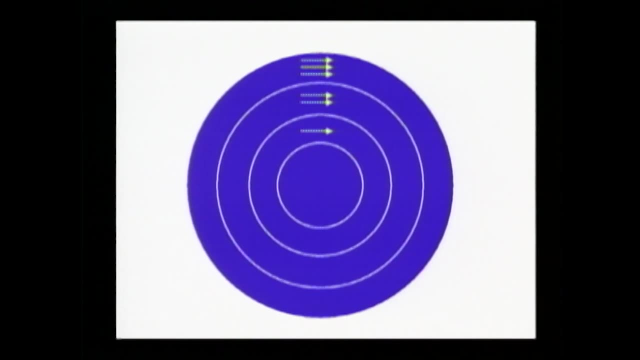 So something has to go in jumps. One possibility would be that we have a region where the system is not moving. This means zero matter waves: Here we have one de Broglie waves, here two and here three, But a little bit more detailed consideration. 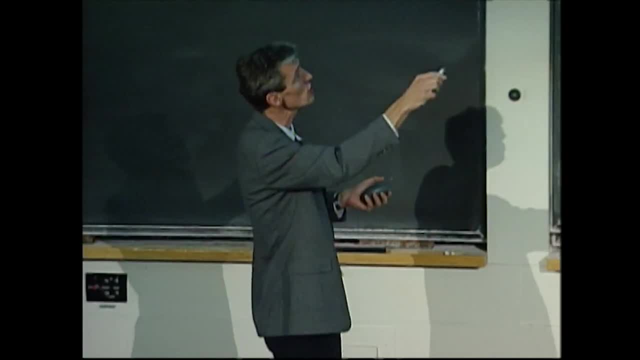 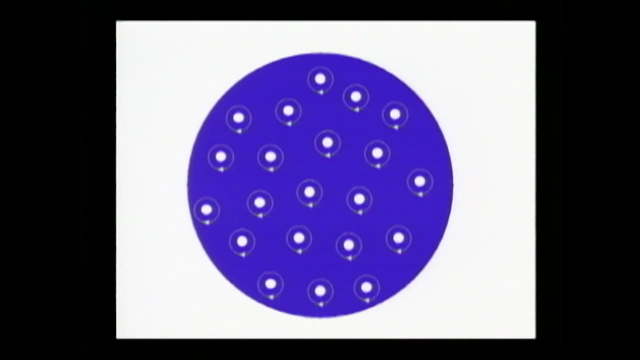 tells us that instead of forming this kind of ring-shaped geometry, it rather the system rather breaks up into little whirlpools, little vortices, And around each vortices we have one full de Broglie wavelength. Now this is a very universal consequence. 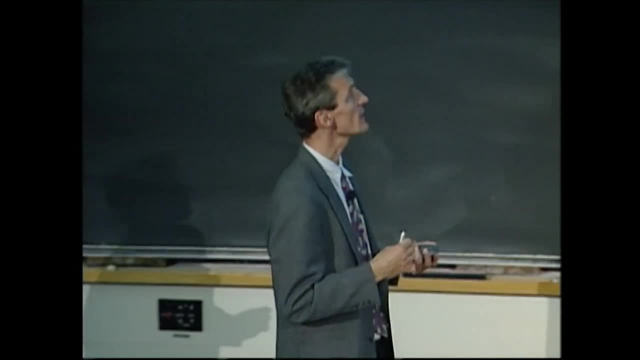 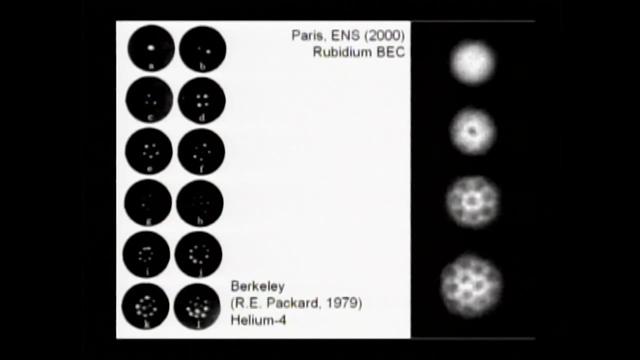 if we have matter, which is a single wave, And indeed there's a very important experiment done 20 years ago at Berkeley where this phenomenon was demonstrated with liquid helium And also with Bose condensate. It's recently a group in Paris showed this effect. 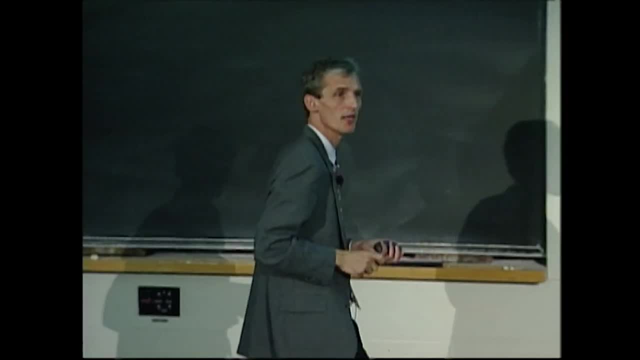 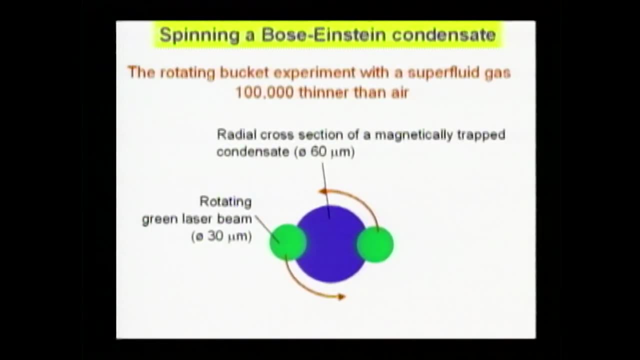 I'm now talking about recent work, So I want to talk now about things which were done in our laboratory less than a year ago. So we tried to sort of go further and study further aspects of it. So what we did is- and this gives you- 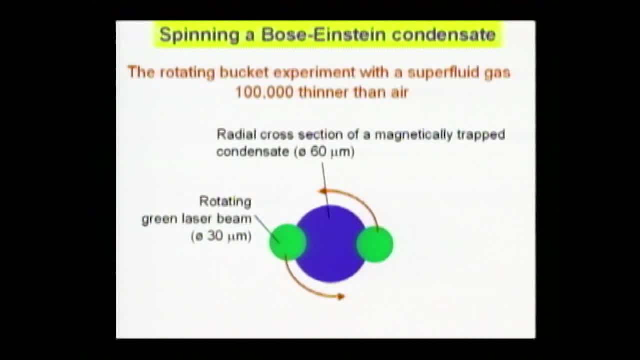 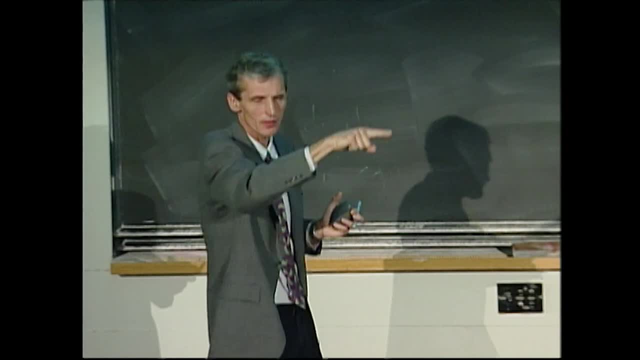 sort of a taste. what happens in building 26, is this tiny little cloud in a big vacuum chamber And then we use a laser beam And we rotate the laser beam around the cloud And with the laser beam we are spinning up the gas. 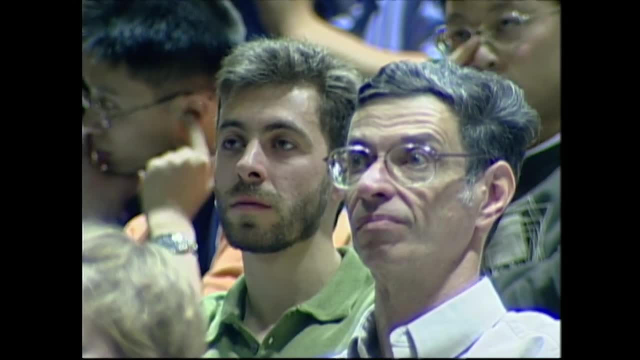 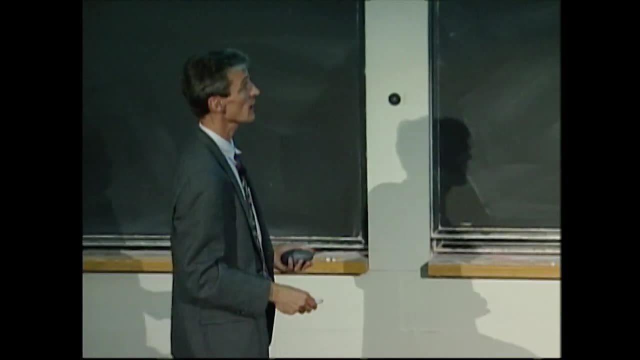 And we are setting the gas in rotation And then if you let the gas go, if you let the cloud ballistically expand, we can now compare the cloud without rotation: It's just a blob which expands, as I've shown you before. 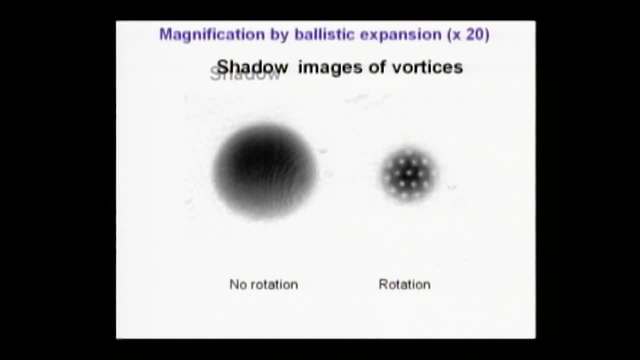 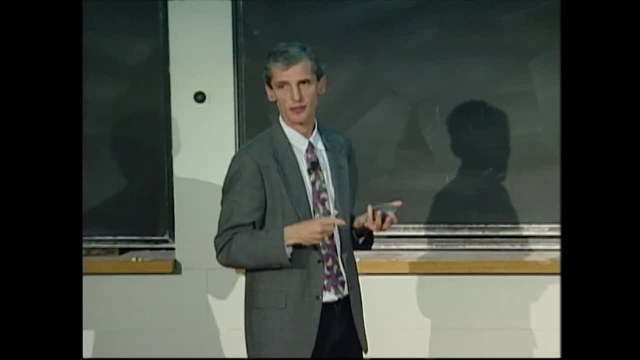 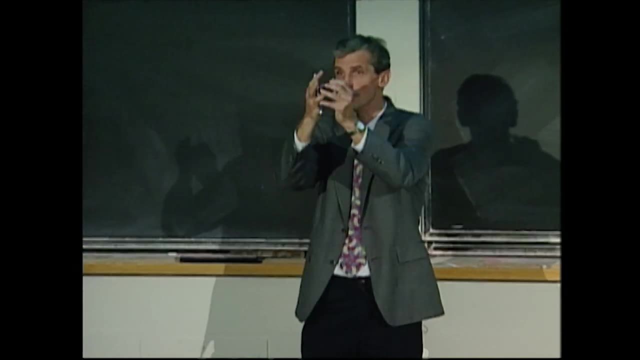 But with rotation we observe those whirlpools. So this is again a very clear manifestation of the wave nature of matter. Ordinary, Standard substances would not behave like this. And again it's the most direct observation. It's a cloud which rotates. 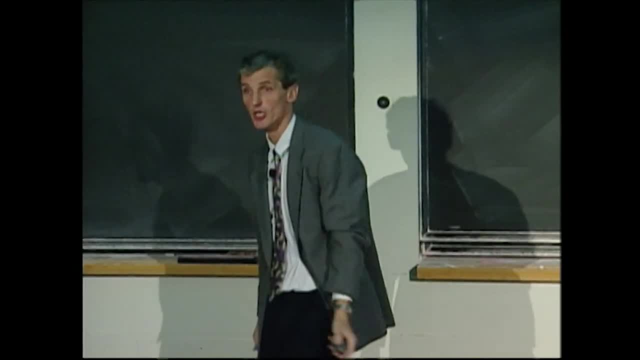 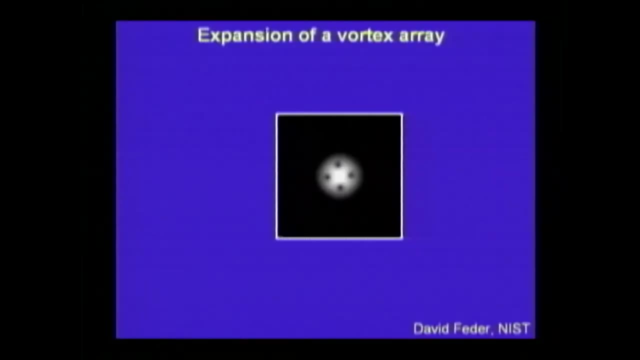 You let it expand, You take a picture, And this is a shadow, a shadow of this cloud. Actually, this is a simulation by one of my colleagues which shows that this structure of whirlpools is preserved upon expansion of the gas. We can't directly photograph the cloud while it is still. 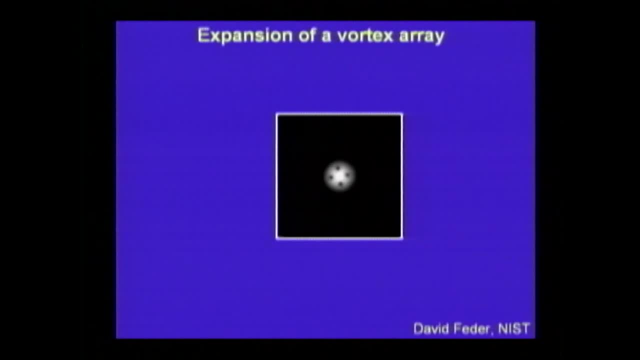 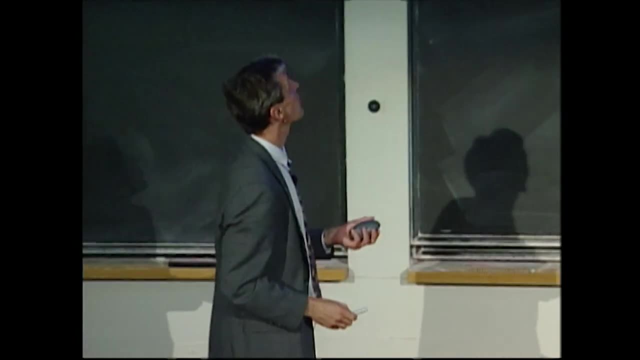 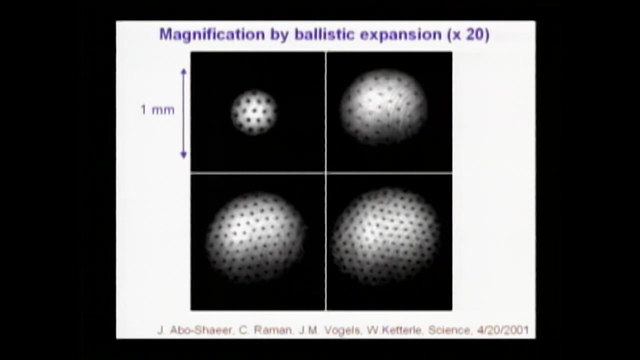 It is rotating because the structures are too small. But by simply switching off the magnetic trap and everything expands. we get a magnification factor almost for free. And the faster we rotated the cloud, the more vortices we observed. So this is an example of a vortex lattice. 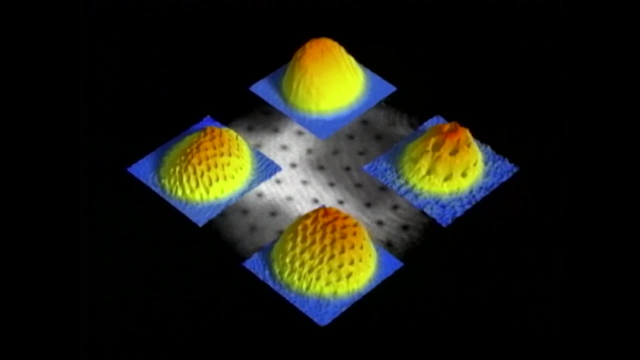 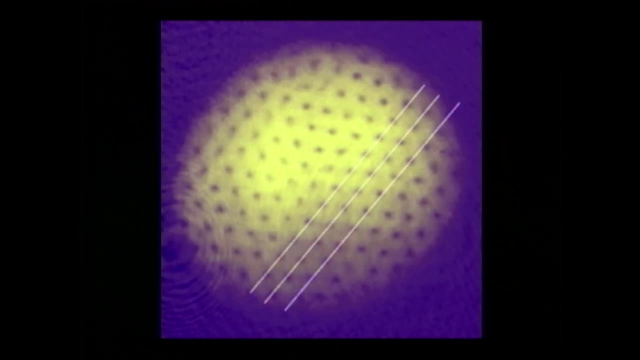 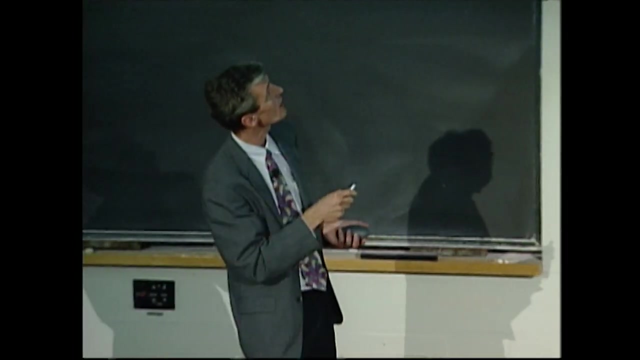 which is perfectly regular. This is just a more fancy representation. But let's just look at this very regular vortex lattice with, say, those lines which guide the eye. We see how perfect nature is, But it's not always perfect. And if you look carefully on the left-hand side, 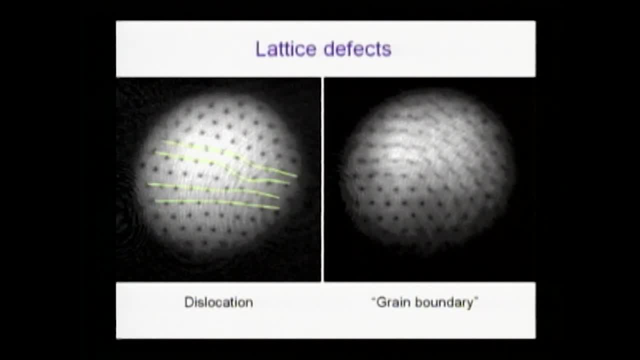 you see a lattice defect, You see a dislocation, an extra row of vortices. So we have now a system- It's a very dilute gas- And we can now study the properties of vortices, study their dynamics. 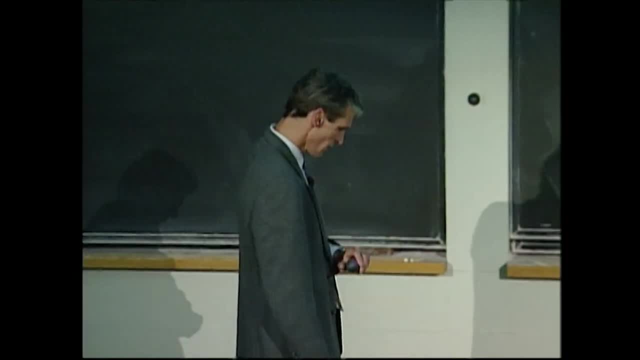 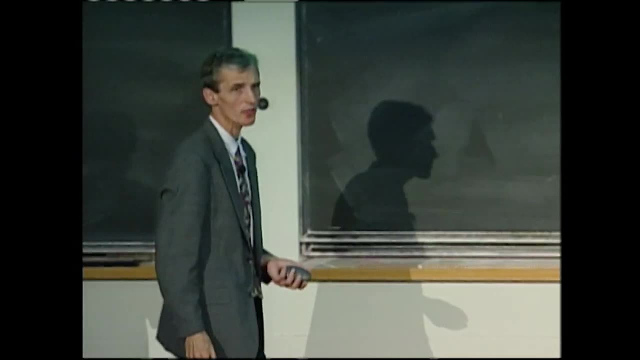 And there's a lot of interest in doing that. But finally, let me talk about this. Let me talk about something which is even more recent and some work which is currently in progress, And this is OK. I will tell you in a moment. 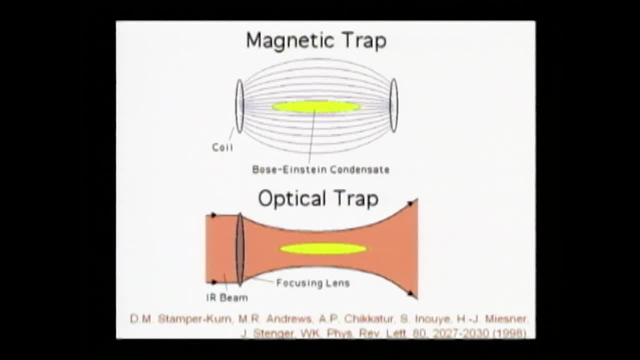 This is related to optical trapping. I told you that our workhorse is a magnetic container. But so well. magnetic containers are nice, They've allowed us to do all this work, But they have also the limitations, Because if you want to move magnets, 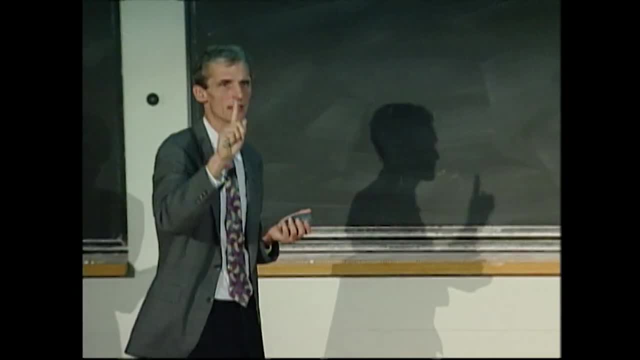 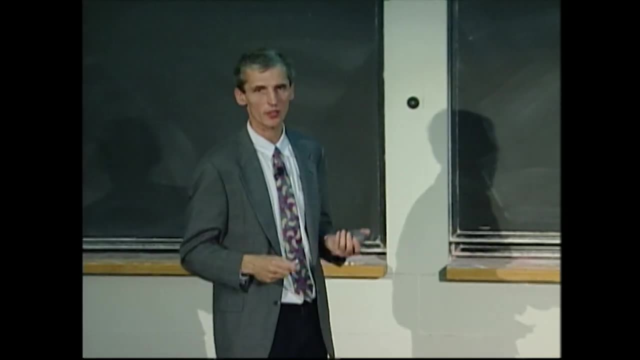 you may have to move all the magnets around, You can only keep them. You can only keep atoms in spin-up states and not spin-down states. So there are many reasons to put those Bose condensates into other containers, And this is a container which is not using magnetic field. 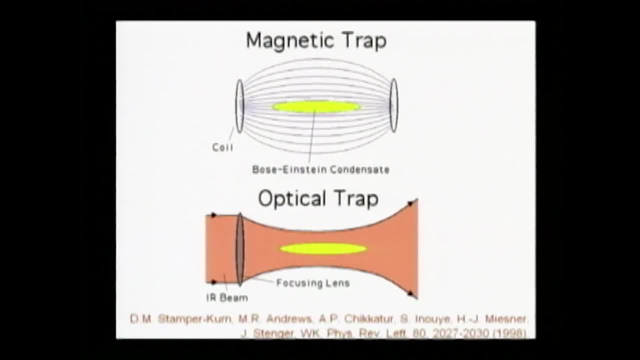 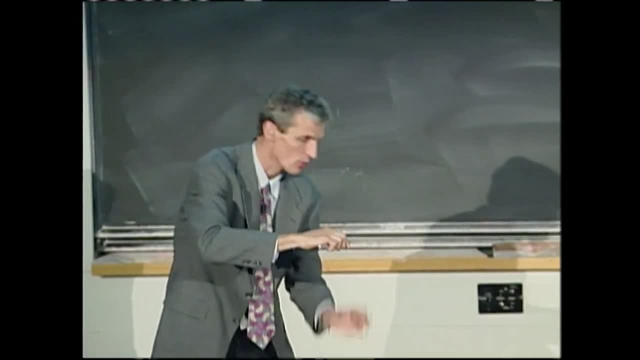 but electric fields, And it's the electric field of a focused laser beam. We call it optical tweezers because it's really like a laser pointer. We bring the light to a focus And this focus sucks atoms into it, just by electric forces. 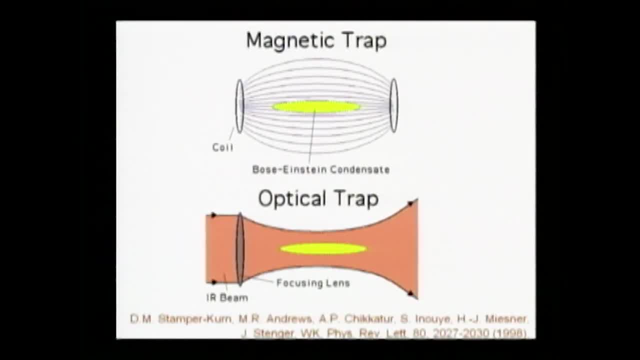 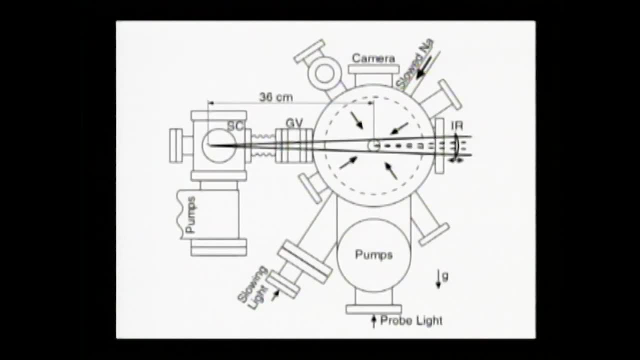 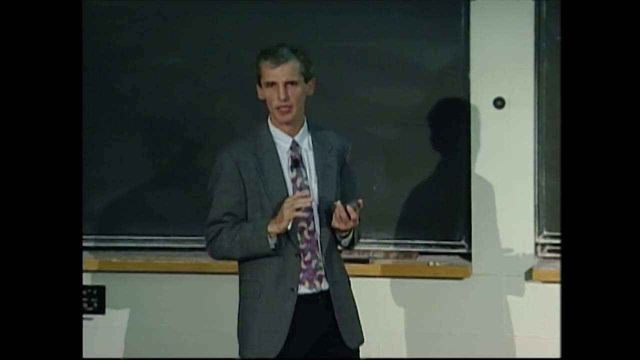 So a couple of years ago we showed that we can transfer condensates from the magnetic trap into an optical trap, But our piece of pride and our latest accomplishment is that we are now able to use this optical trap as a transport mechanism for Bose condensates. 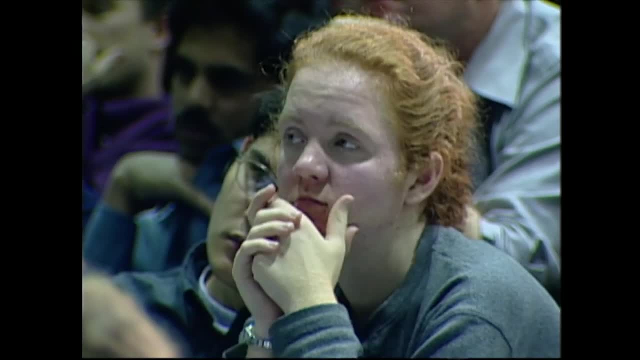 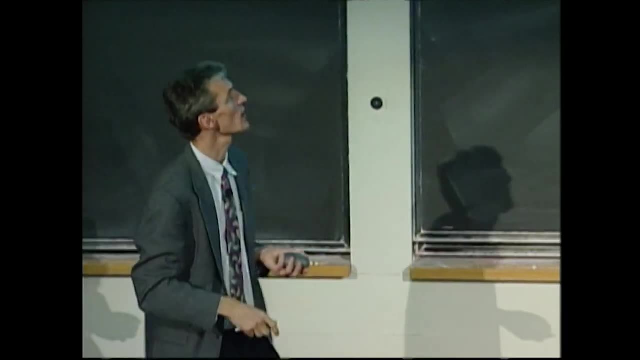 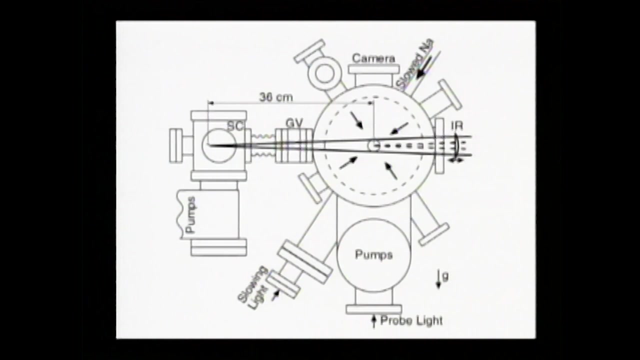 So by taking not really the laser but a lens and translating it, we can move the focus by 40 centimeters. So our group has now the unique ability to form a condensate in one vacuum chamber, then focus laser light on it and translate the focus. 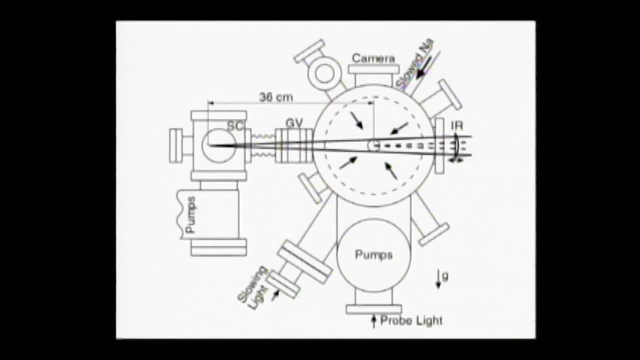 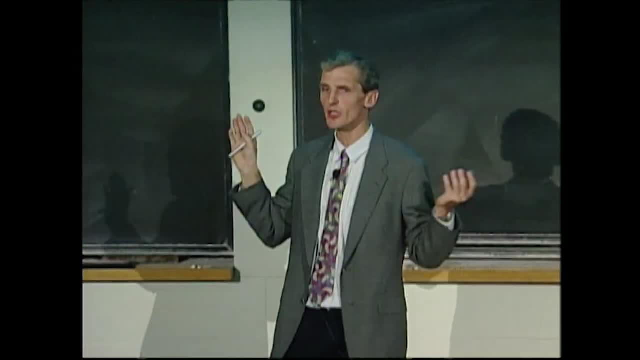 by about 40 centimeters and carry the atoms in a new chamber. So we are now able to deliver condensates with precision through pinholes and put condensates into whole new environments close to surfaces, into micro traps, into resonators. 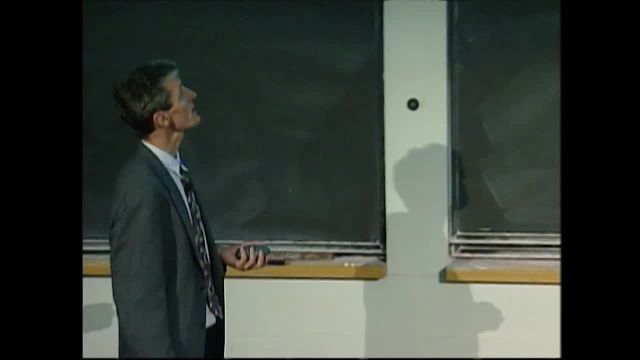 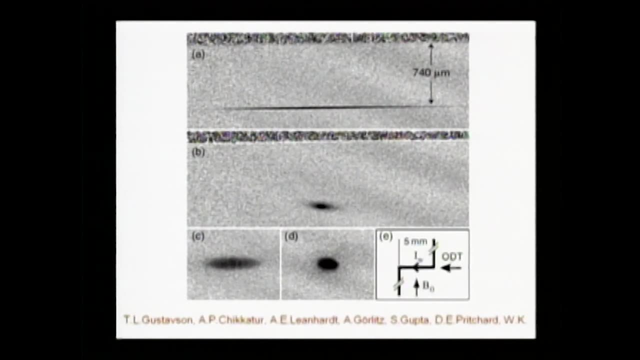 And there's enormous excitement. And let me just say, Let me just show you one of the results. This is 40 centimeters away from where we produce the condensate. And here it is, And it is less than a millimeter away from a surface. 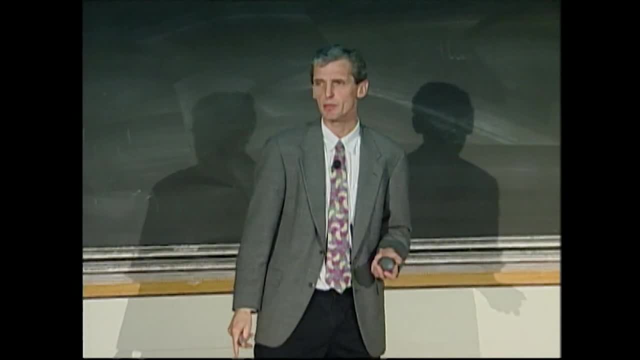 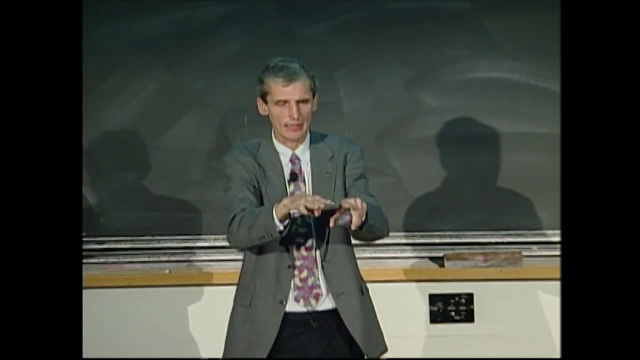 And we think there's a lot of future of atomic physics in that. Some people dream that we can take atoms guided matter waves on atom chips, tiny patterns of wires on a surface, and we guide the atoms around like in an ordinary chip. 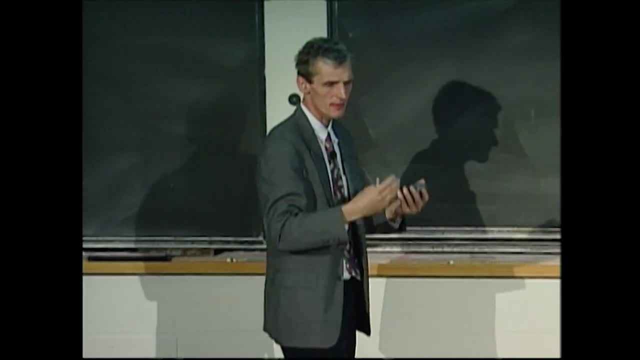 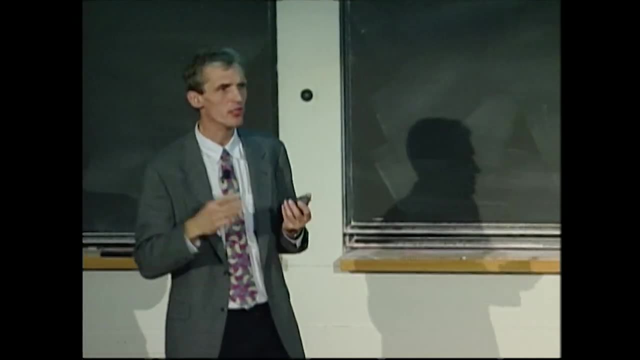 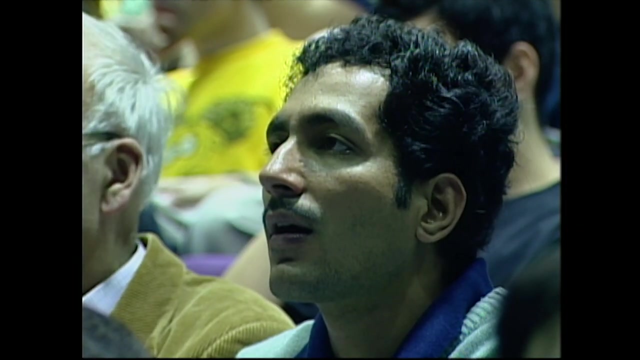 electrons, The atoms are guided And this may allow us to have new geometries, to find new properties of quantum systems. but it may also allow us to build precision sensors for rotation. But I think this example also, or the last two examples, 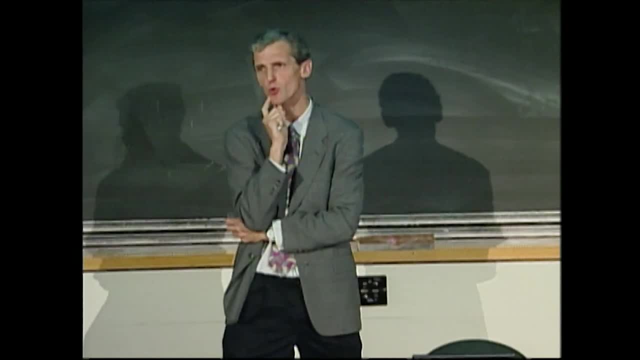 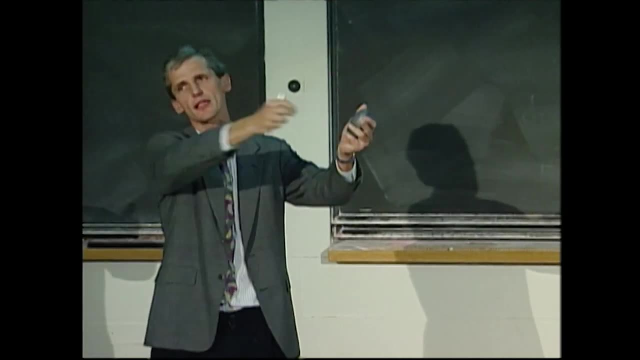 demonstrates some of my surprises. When we were hunting for the Bose condensate, we thought we would be so happy if you would just see it, if you would get there. But now We can take condensates, transport them over 40 centimeters. 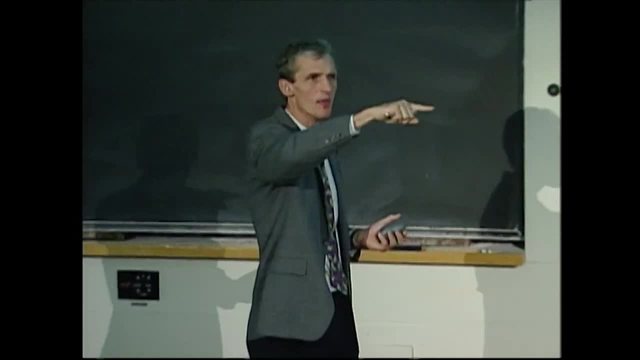 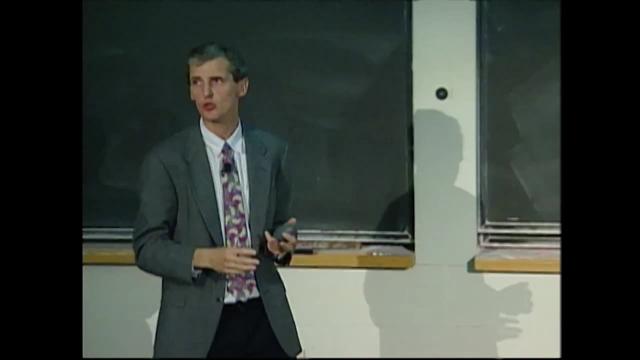 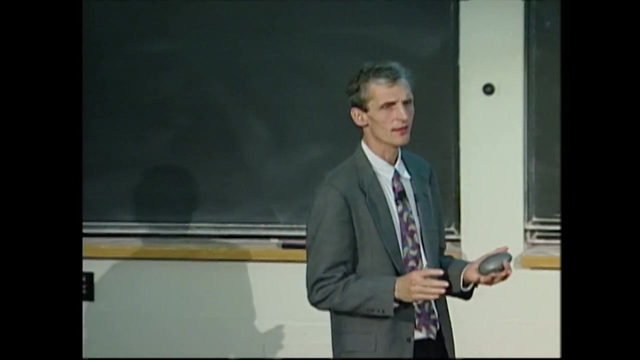 We can keep them for a minute and do experiments. We can spin them at high rotation and see those vortices. So the system is enormously robust and allows to branch out in a large variety of studies. So for me the Bose condensate is now a new laboratory. 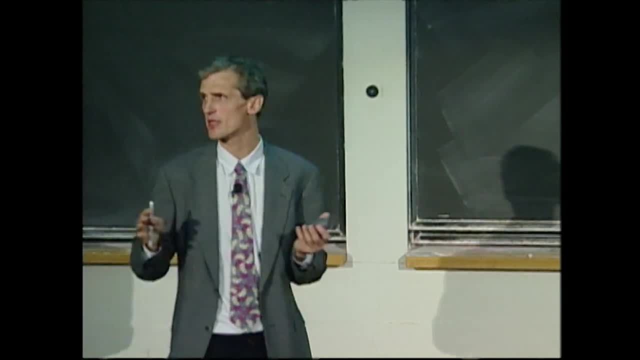 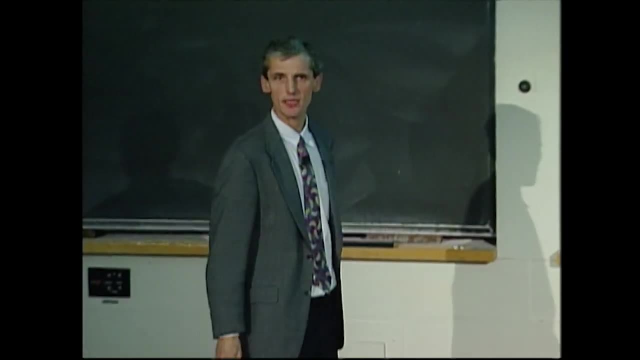 to do all sorts of physics, to do condensed matter physics, vortex nucleation, sound At densities which are extremely low that it's very easy for theorists to calculate the effects. And what I've done here is it's more for the experts. 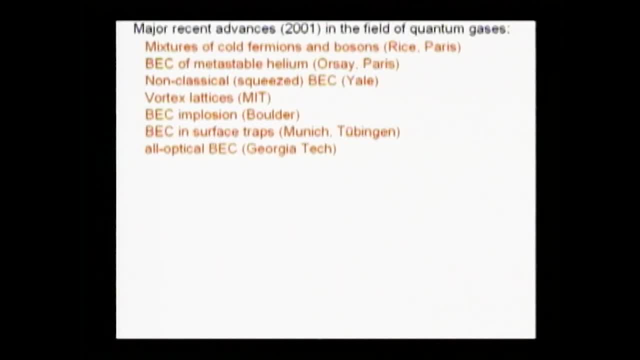 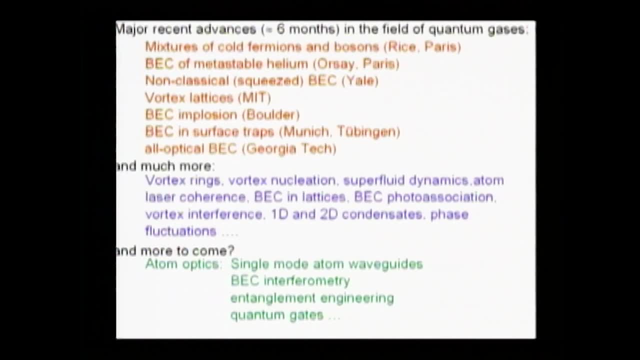 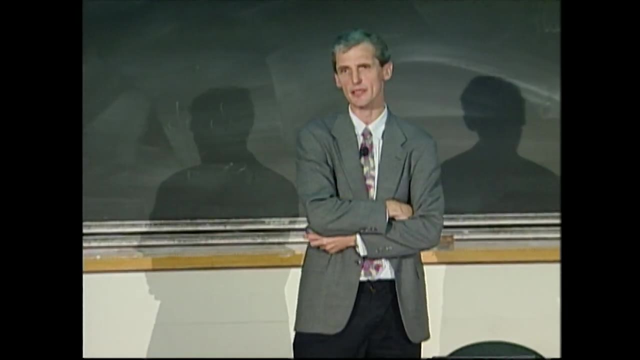 I've just listed major developments in the field which have happened just this year, And there are other exciting things And I think there's more to come. So it's a privilege for scientists to be in the middle of something like this, to be able to contribute to the basic concepts. 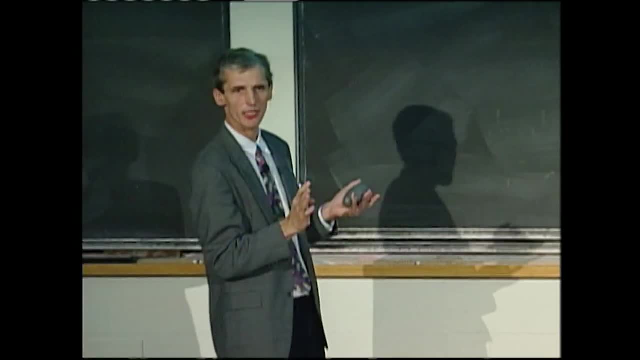 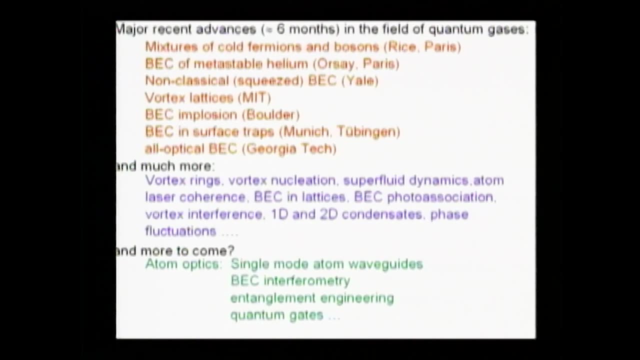 and see this growth of a field and see how it's branching out. Actually, I don't have a slide for that, But one question which almost everybody asks me: what is the application? What will come out of it? Now, my take on that is twofold. 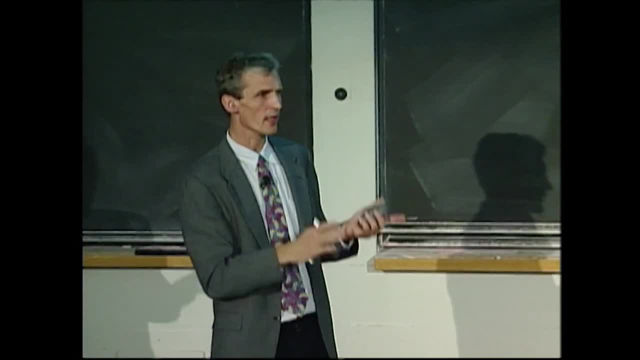 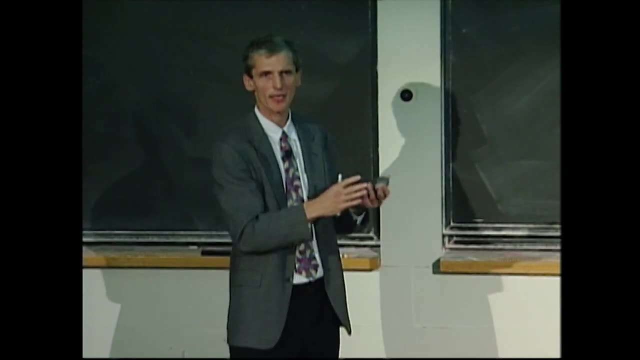 One is: it's fundamental research, And we do fundamental research to learn about properties of nature, to find properties of matter at ultra low temperatures, to understand macroscopic conditions, And that's what I'm going to talk about in the next lecture. 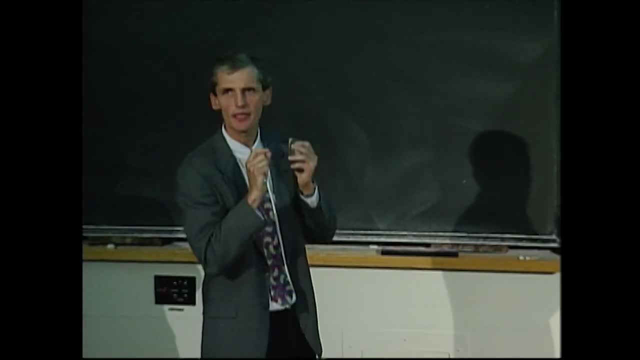 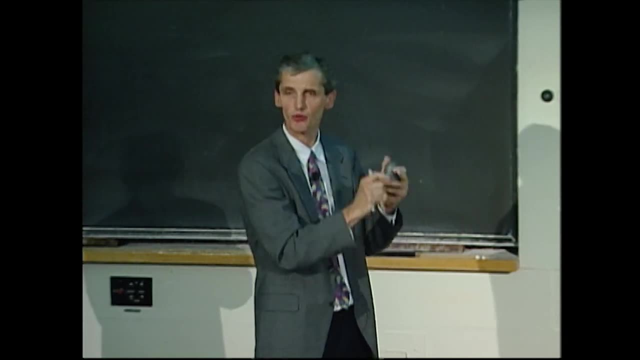 And then I'm going to talk about quantum mechanics and quantum mechanics and quantum mechanics and macroscopic quantum mechanics. On the other hand, what we are doing here is we are learning how to manipulate atoms, the building blocks of nature, with unprecedented precision. 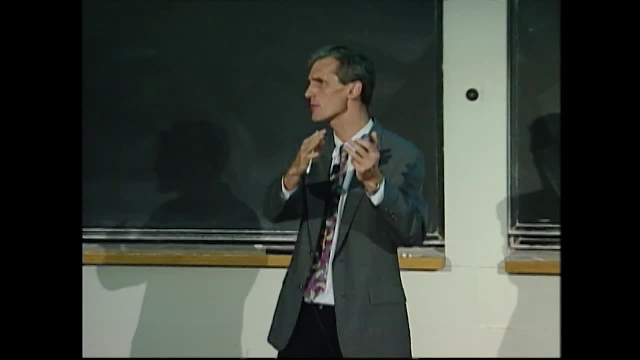 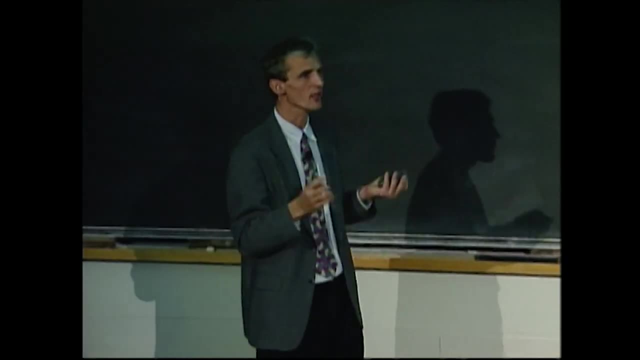 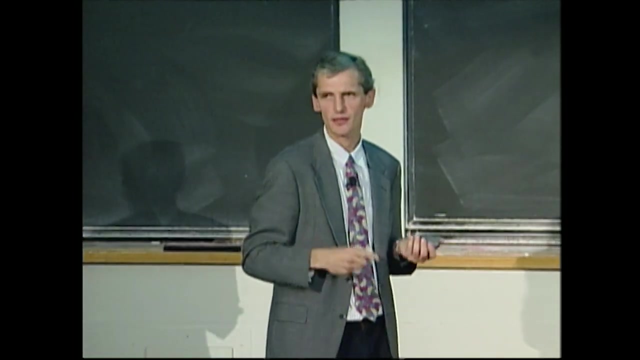 We have quantum control over the atoms, We control their wave properties And this unprecedented control over atoms may lead to precision measurements, may contribute to random computation. But this is at the horizon And collaborators and other groups are exploring that And future will tell what is possible. 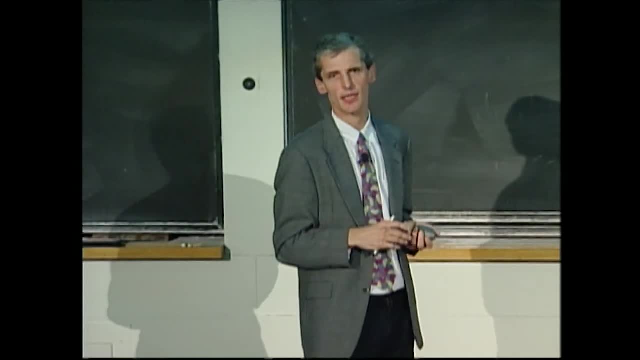 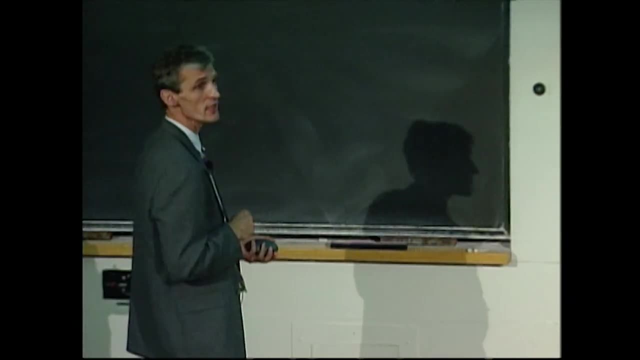 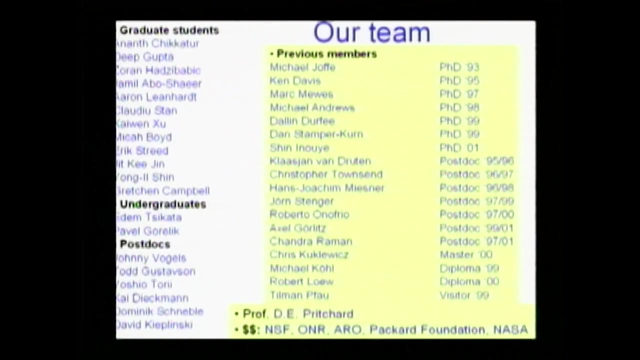 But if I look backwards, usually if something basic is done, our imagination is not sufficient to predict what it is good for. So finally, let me acknowledge the people I was really privileged to work with- I think the best team of students and postdocs in the whole world. 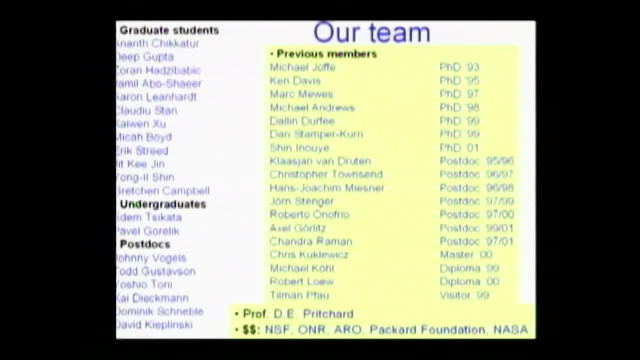 This lists the people who have left the group and contributed to the work, But here's also a long list of people who are currently carrying out this exciting work. Usually I show a group photo, But I realize we haven't taken a group photo recently. 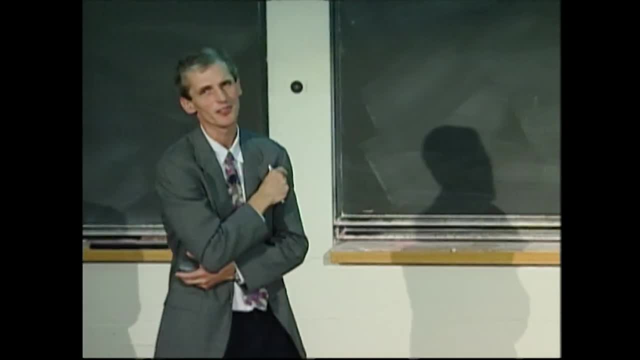 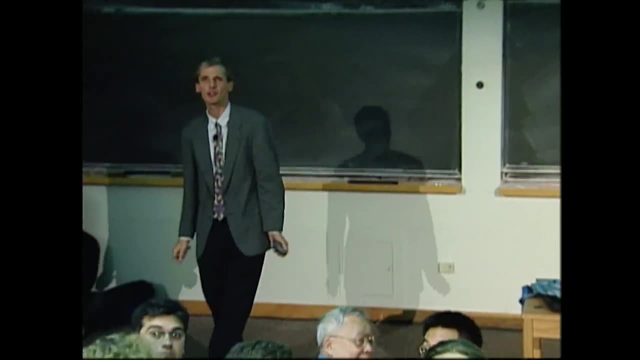 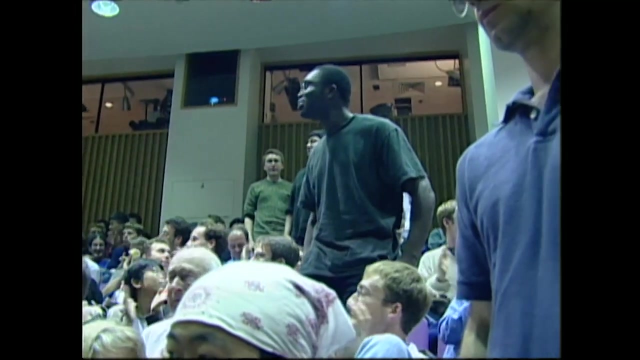 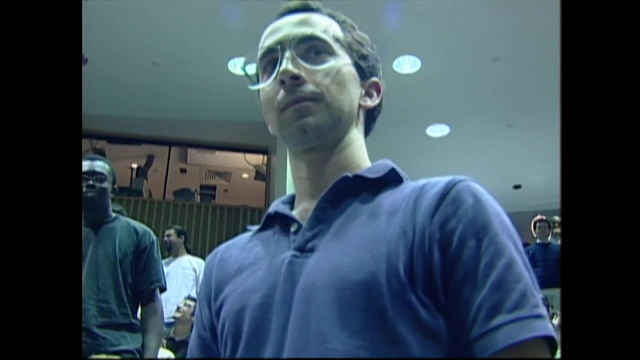 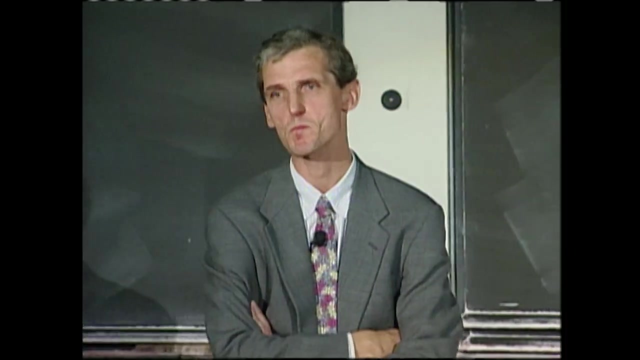 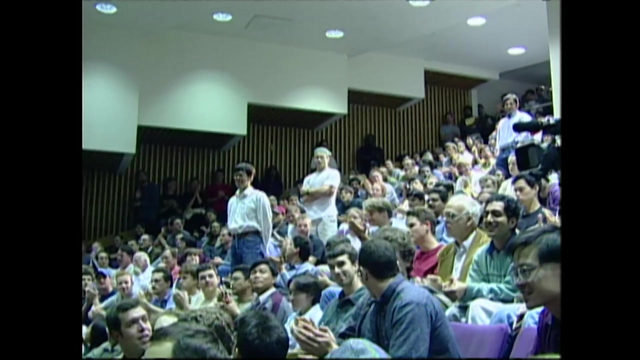 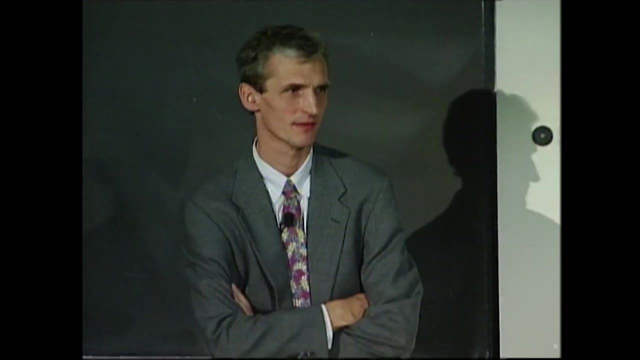 So may I just ask the people who are working with me just to stand up- And it's a live group photo And they're carrying out this work And they deserve the applause, And they deserve the applause, And they deserve the applause. 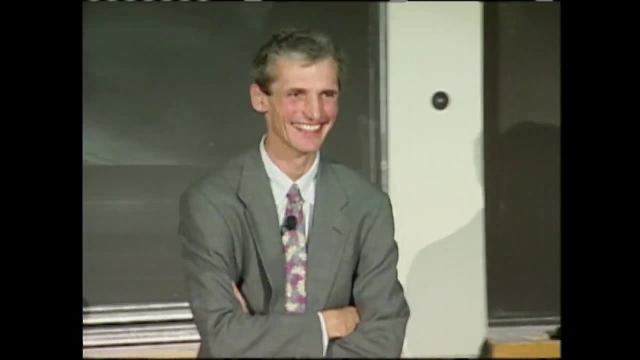 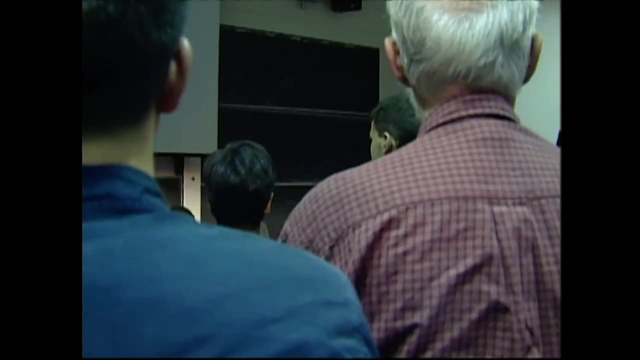 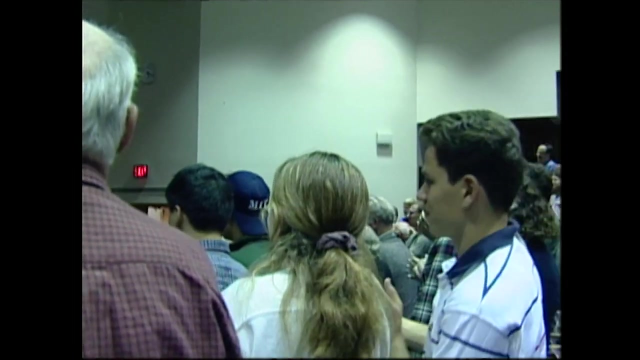 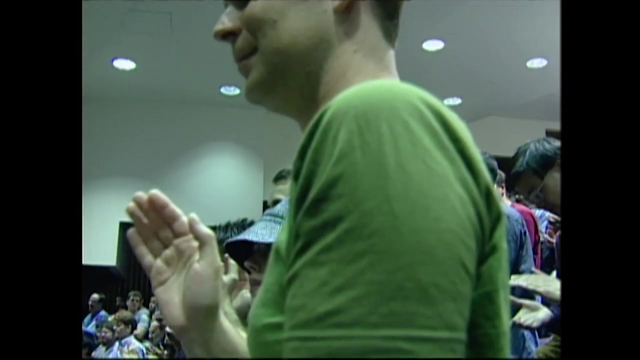 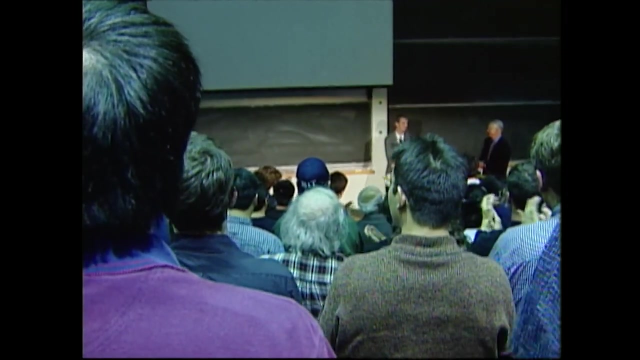 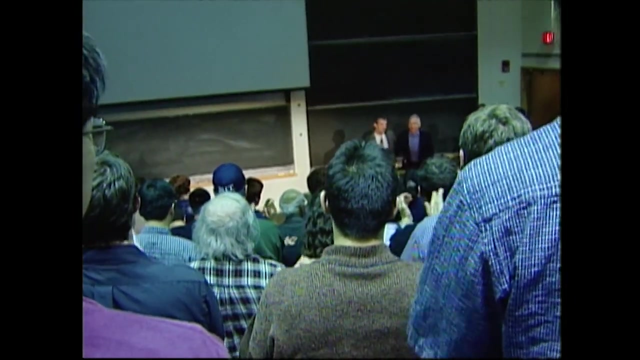 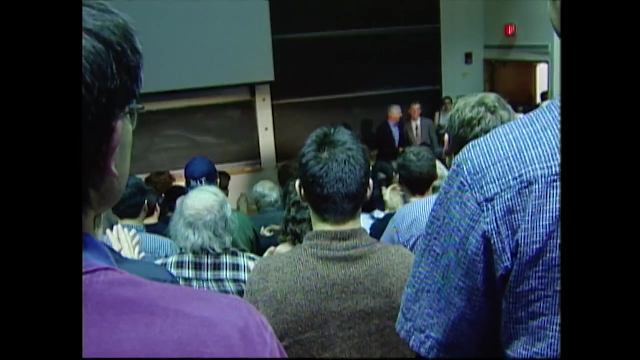 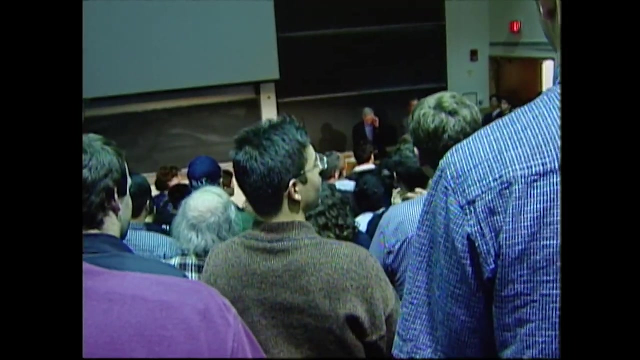 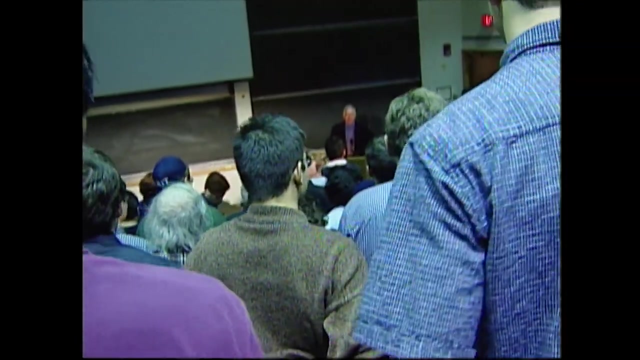 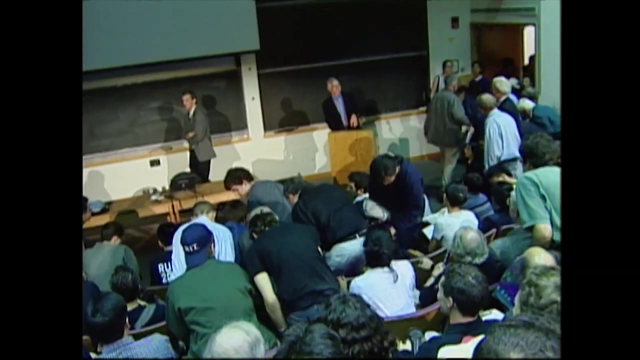 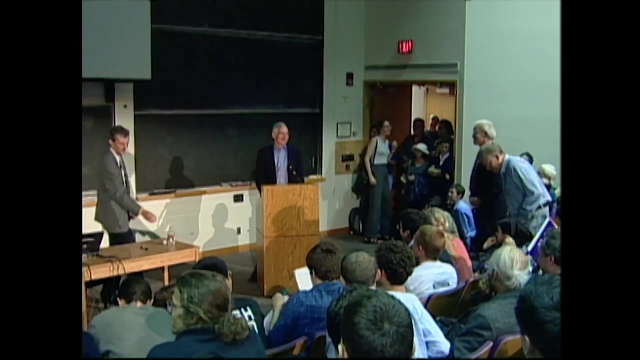 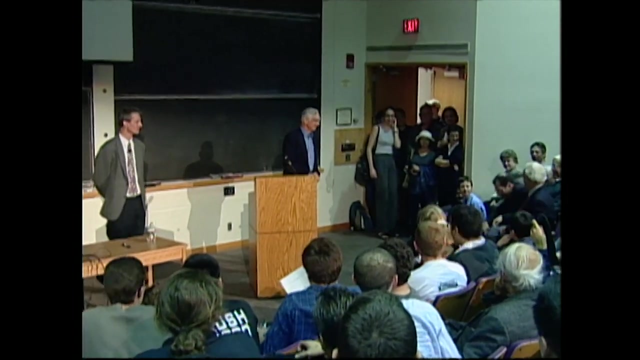 Thank you, Thank you, Thank you. Well, that was fantastic, Wolfgang. You've lived up to expectations. Are there any questions? Oh, OK, It's just fine. I don't think there have to be any questions. Mark, would you like to say something?